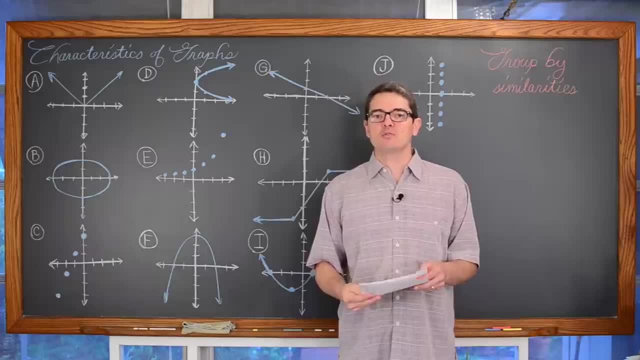 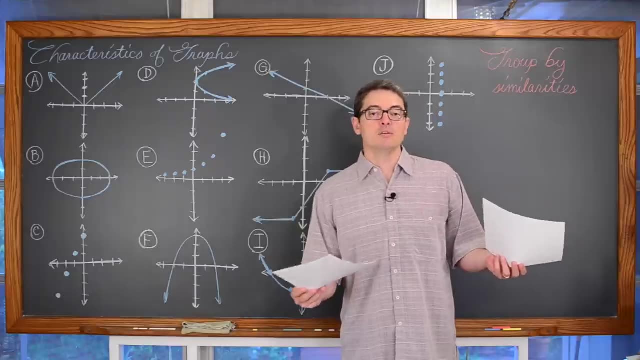 you can go to deepen that understanding. I am also going to include links in the description, in case you are using a mobile device and you don't have flash. Same thing with whether a function is continuous. There are fancy ways of proving if a function is continuous. 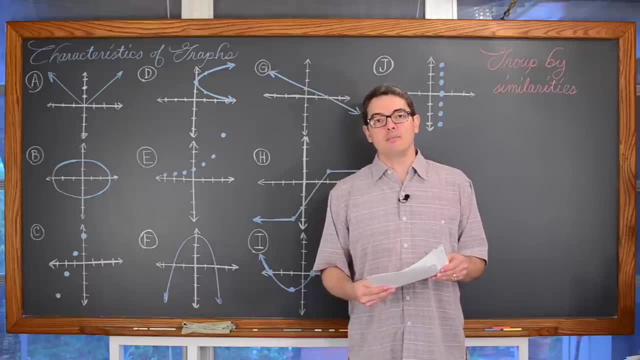 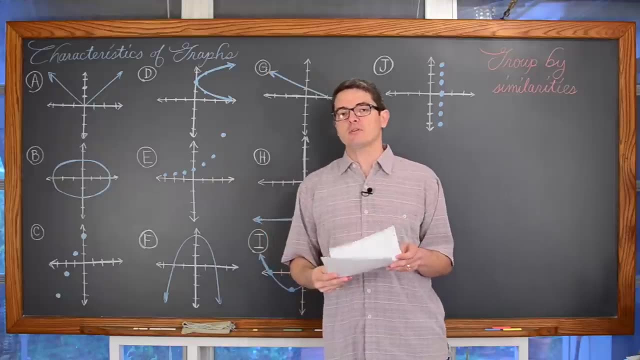 at a point in calculus using an idea called limits, Same thing of a smooth curve In an algebra class. we are just going to kind of look visually at how the graph looks. But there are more in depth ways of proving that, Proving whether a function, again, is continuous. 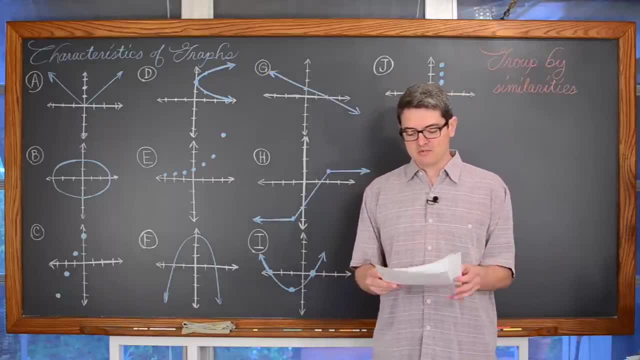 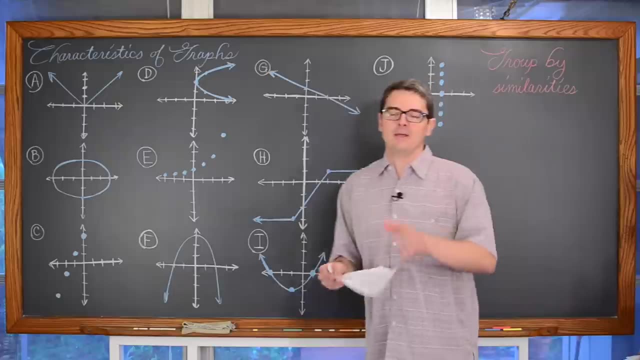 or smooth at a point using some calculus techniques. So if you need more understanding than I am giving you in this lesson, well then you will know where to go. If you are just in algebra and you are kind of like going well, how is this going to get used later, at least mathematically? 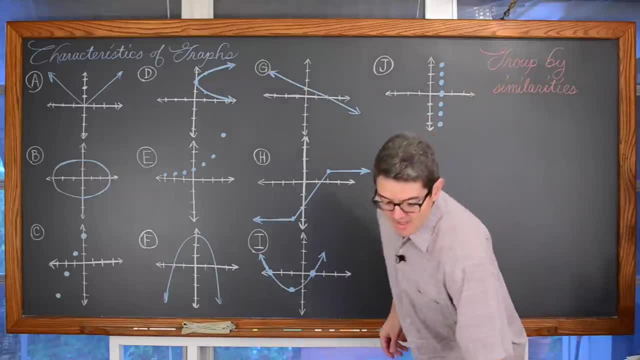 you can go to those lessons and get a more in depth understanding, But for right now, what I would like you to do is I am going to step off. I would like you to look at these ten graphs and group them- Just you know, by visualization. I am going to step off. I. 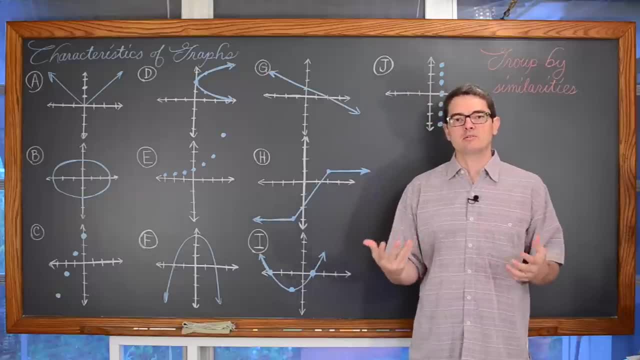 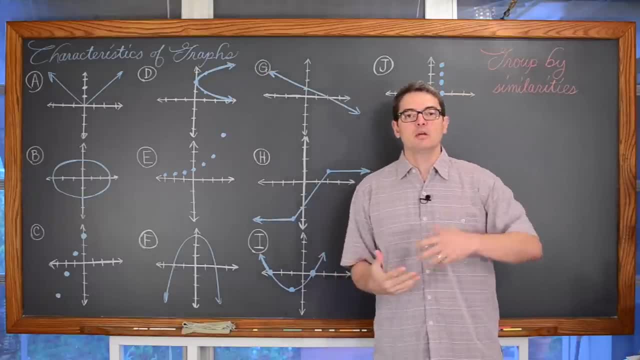 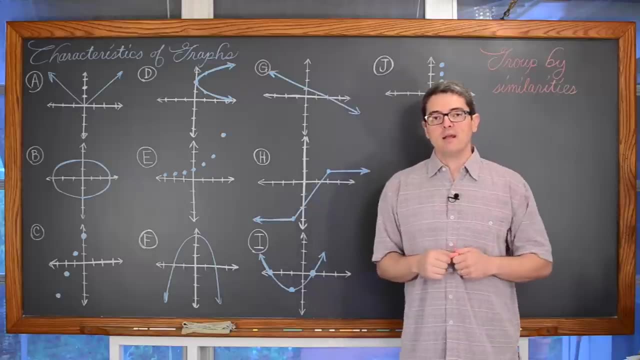 and maybe create, you know, six, seven, eight, nine groups of like type graphs by some visual characteristic. Then I have come up with my own groupings already. Maybe I will do more groupings than you, maybe less, but how I looked at these and I am going to use these, 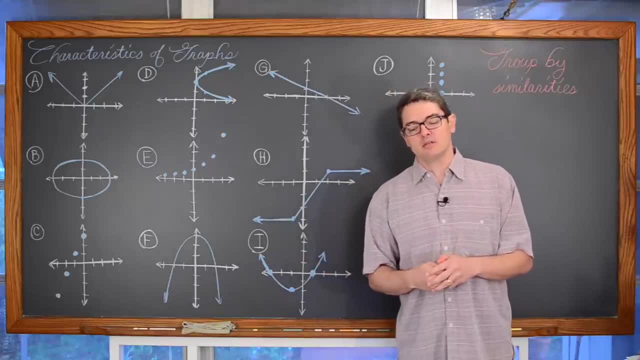 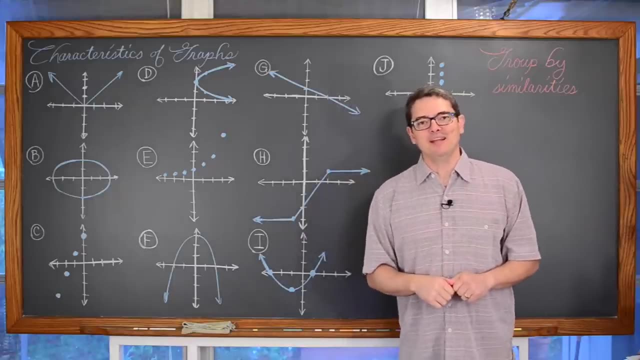 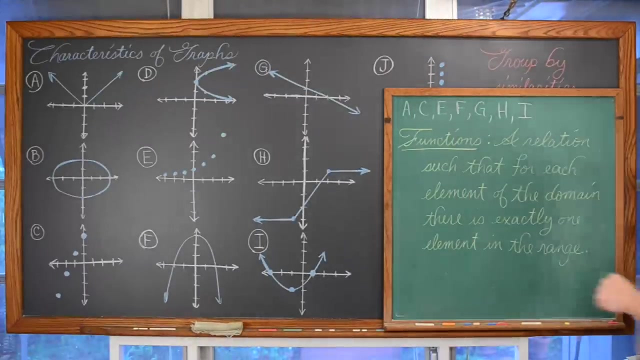 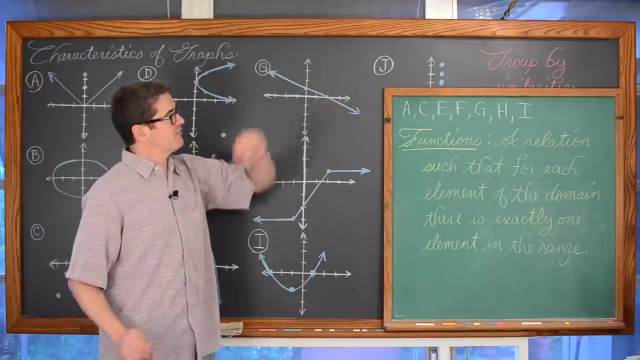 groupings to introduce the definitions that I just said we were going to go over in this lesson. So pause the lesson and make those groups. I will be back in just a minute. For my first grouping that I came up with, we have graphs A, C, E, F, G and H. Sorry, 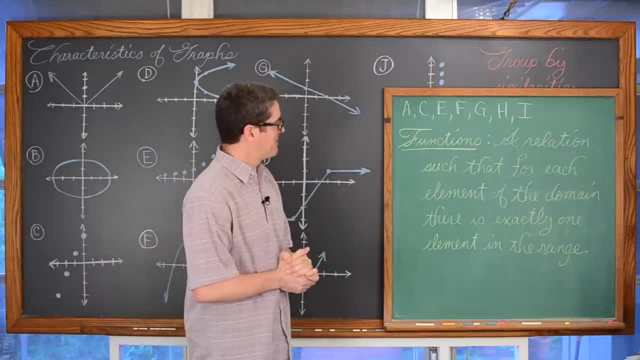 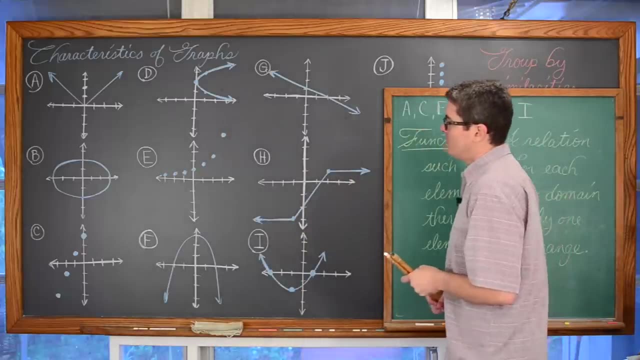 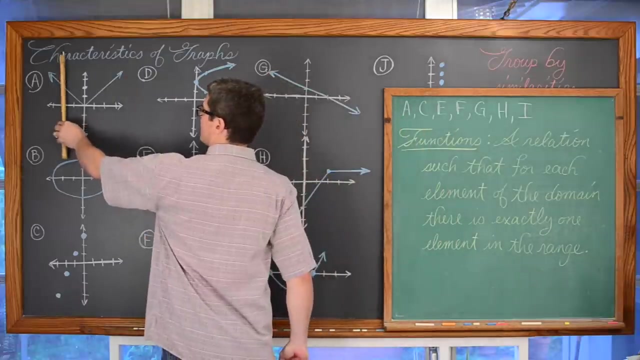 for covering up J. I guess I put it in a bad spot. But the reason why I have these all grouped together is because, when I look at them, well, if I use my chalkboard compass as a straight line, anywhere that I place a straight line- 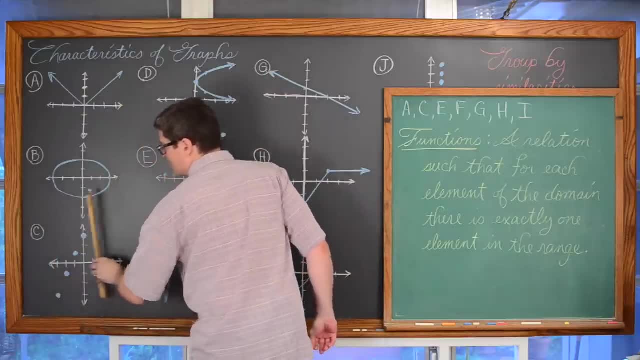 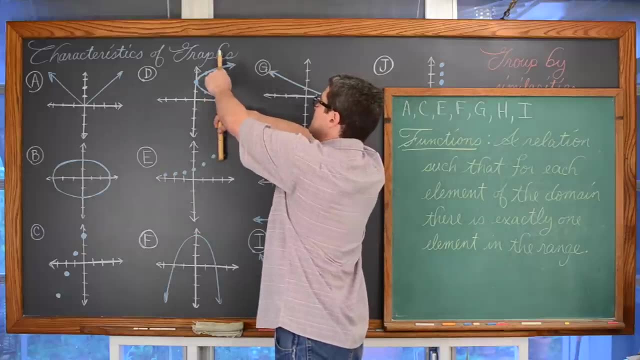 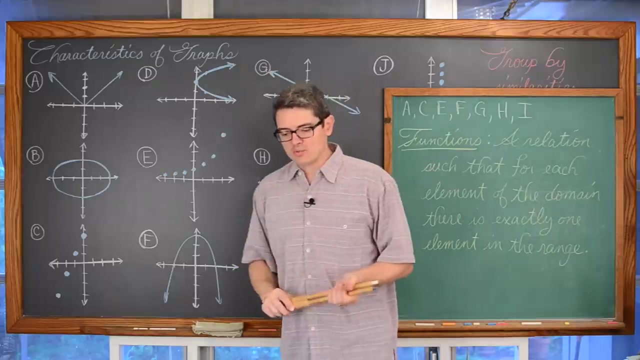 my straight line is only intersecting these graphs at one point, Like: where is D? The reason why that is different is if I place a vertical line here, I am crossing the graph twice. Ok, now a vertical line, depending on where you are in your algebra studies the equation. 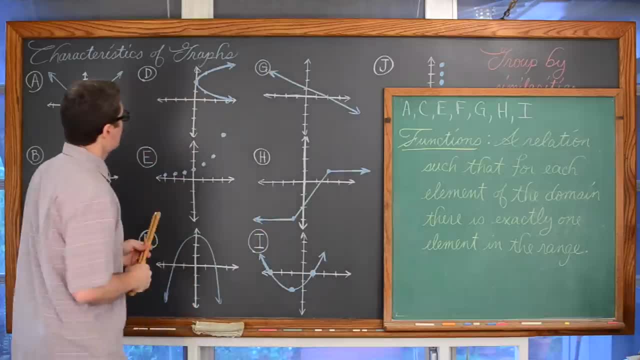 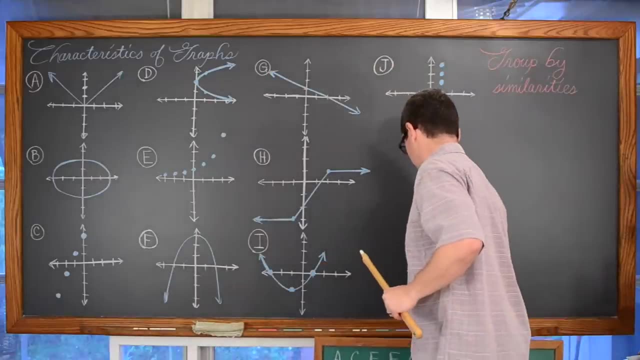 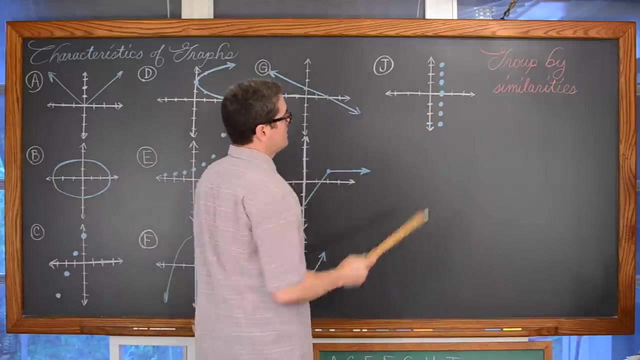 of a vertical line is x. x equals a number. If I say: well, let's see here actually the points that I covered up, those blue dots are in a vertical line. This is point. This is actually- excuse me, I just misspoke- is right there. 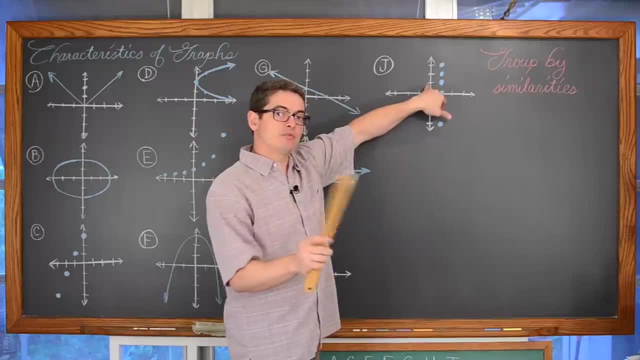 When you plot a point, the first number, the x, tells you how to move left and right, and the second number, the y, tells you how to move up and down. So means from there, From the origin, don't move left and right at all. zero, and then one move up one. 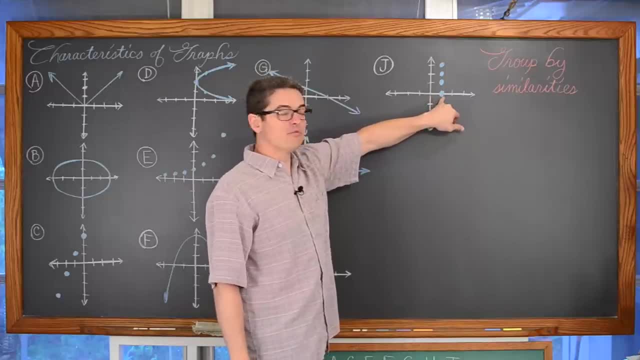 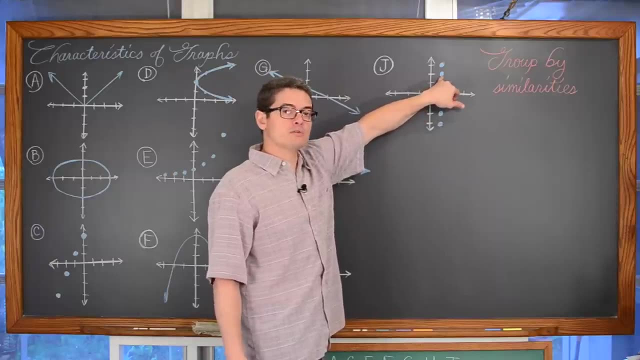 So, excuse me, this first point is one zero. One. move over, one zero. don't move up and down at all. This point, this coordinate of this point, is the coordinate of this point, is the coordinate of this point, is the coordinate of that point, is that point. 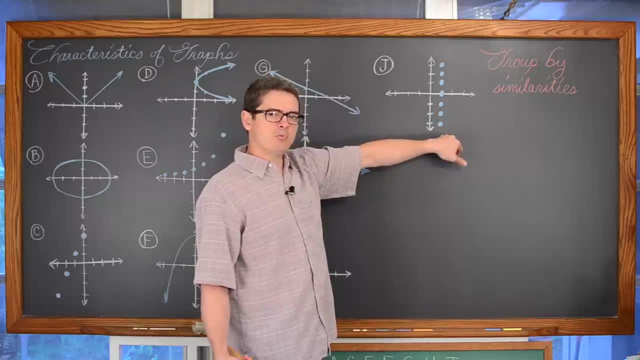 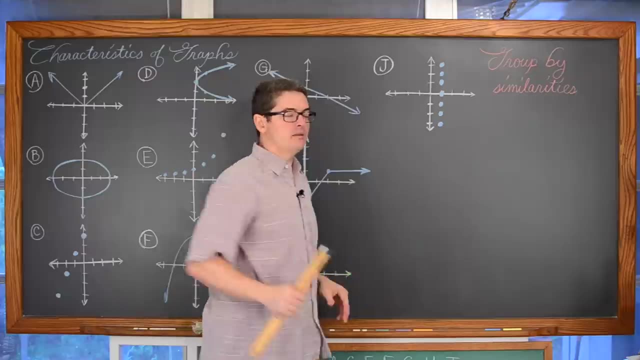 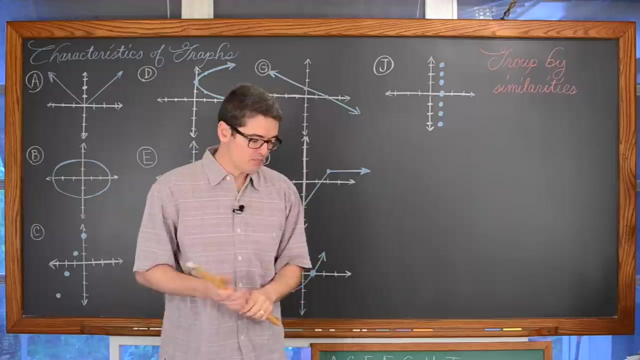 is, Every time I point to one of these blue dots, I am saying the same x coordinate one. Ok, So when you look at a vertical line, the equation of a vertical line is: x equals a number, because every point on that vertical line is going to have the same x coordinate. 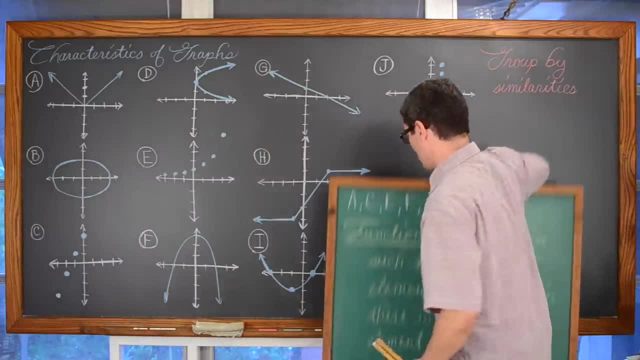 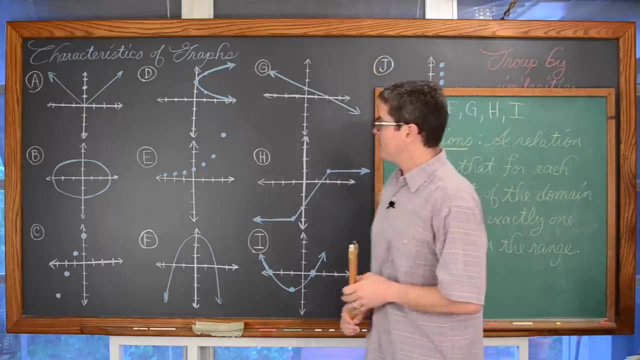 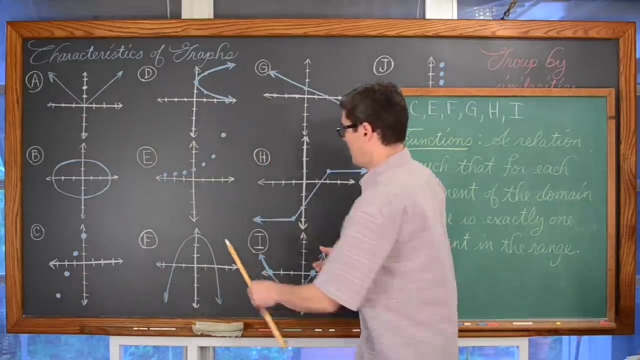 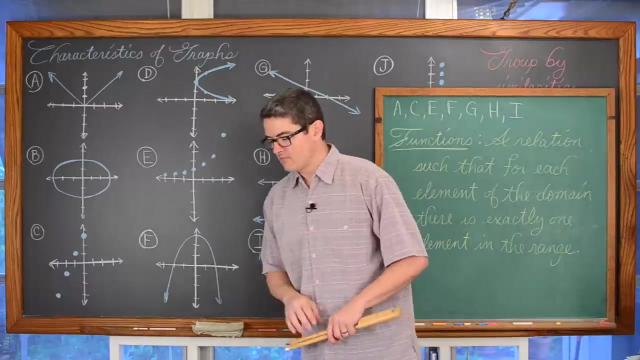 So, as I hold up my compass in an up and down fashion or as a vertical line, I am really identifying an x coordinate. And so, for each of these values of x, for each of these values of x, for each of these values of x, that vertical line is only crossing the graph once. 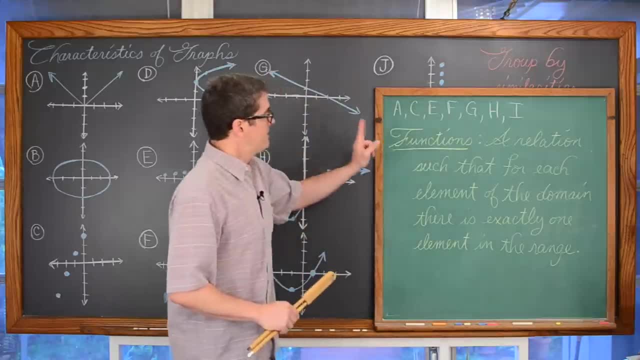 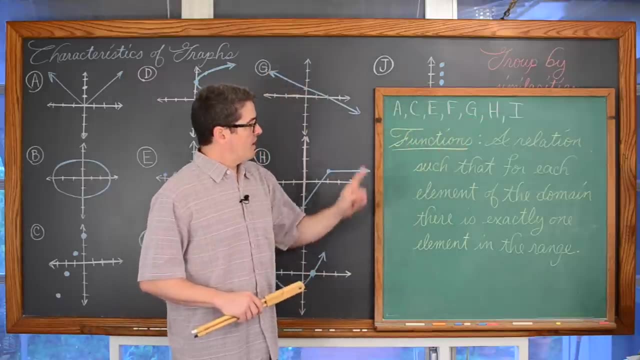 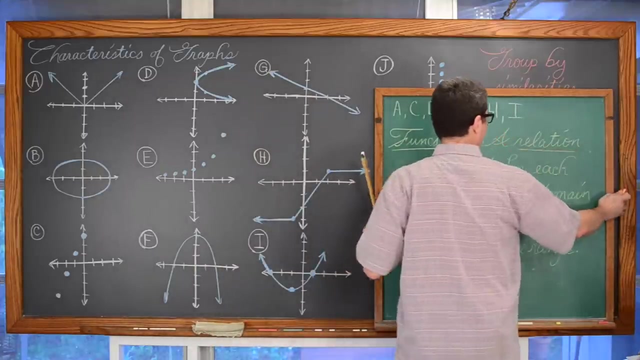 Well, that means that for every individual value of x, there is only one y, That is identifying- whether you have heard this definition or not- that these graphs are all functions. A relation, a function is a relation. Now, this is a bit of a problem because, at least in this video, I have not defined yet. 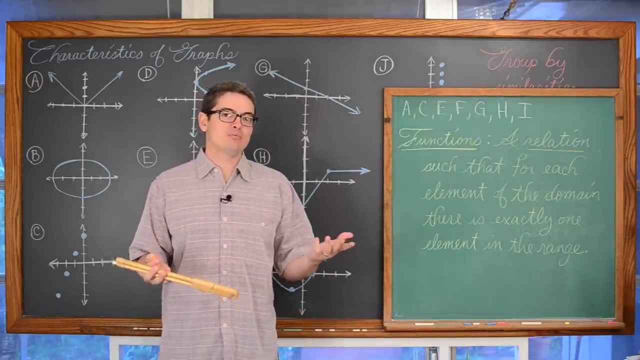 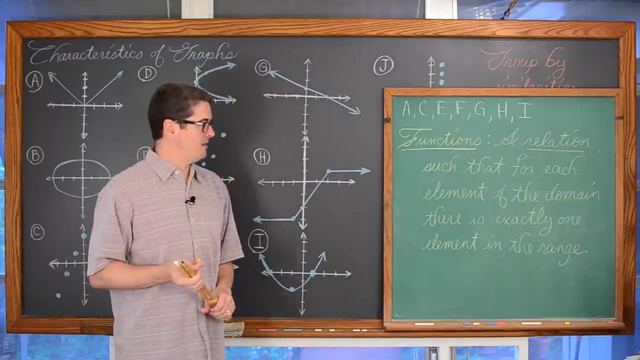 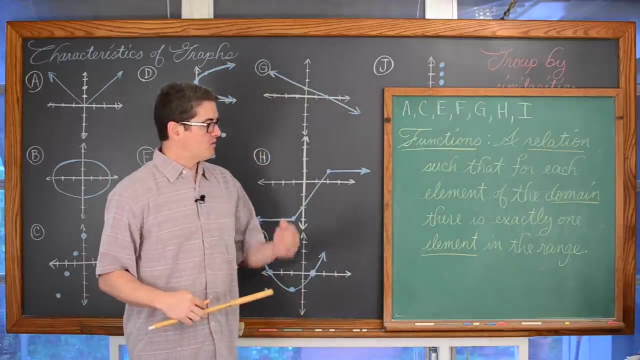 what a relation is. So I am using my vocabulary. You don't know yet, so I will make sure I clear that up next. A relation, a function, is a relation such that for each element of the domain there is exactly one element, that is basically number in the range. 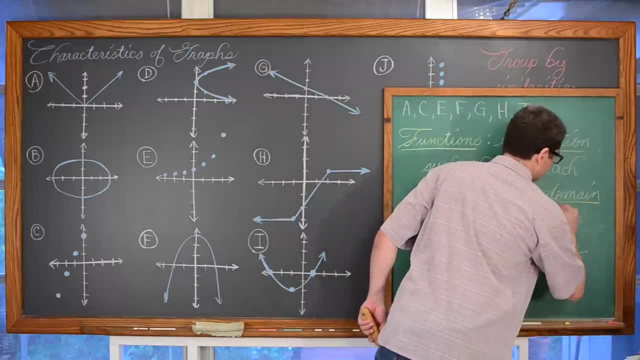 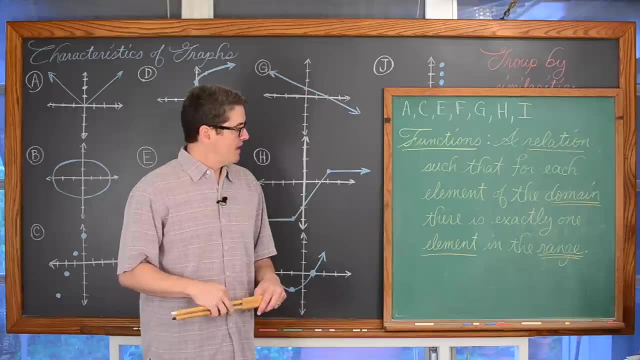 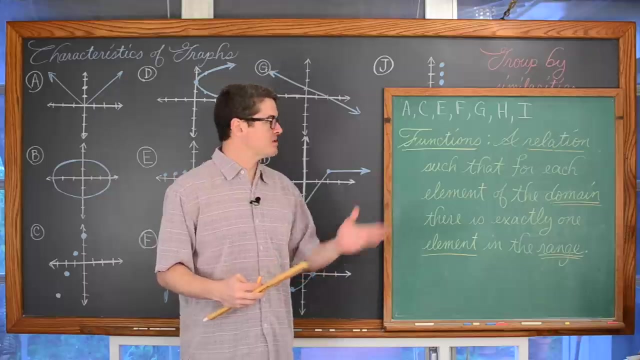 Ok, well, this idea of element is really just a number for our purposes and, well, really for any graphing purpose, And it is talking about domain and range. so there is a couple of words in this definition of a function that you may or may not know. 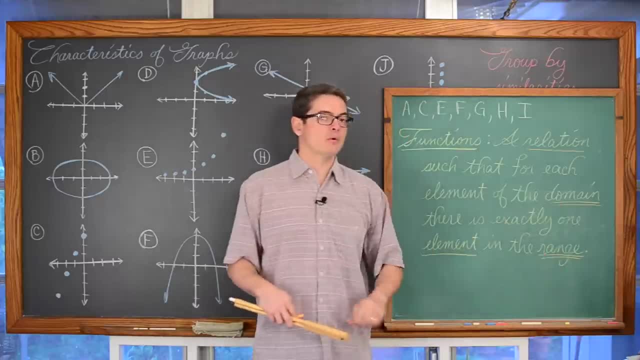 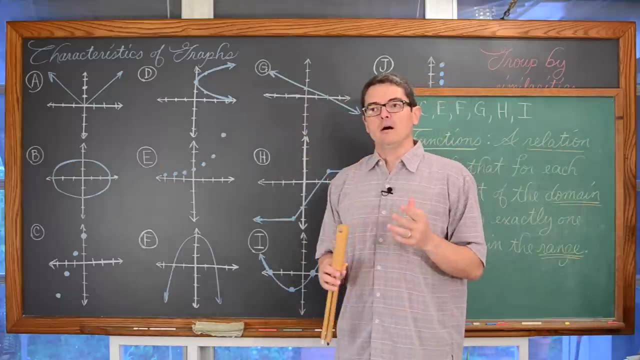 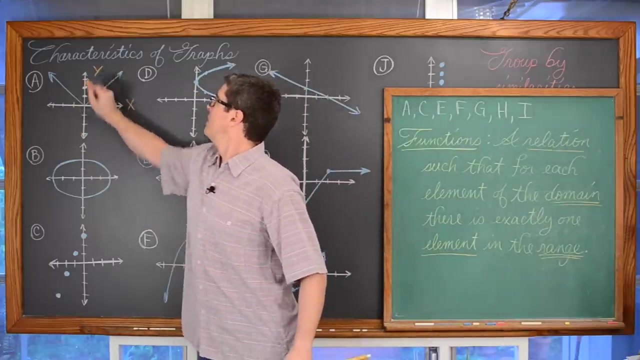 Now, if you are watching my algebra lessons in order, we have already defined what domain and range is. The domain is an input value into an equation, or at least when you are talking about graphs on the Cartesian plane, an x- y axis plane, then the domain are simply all of the x values. 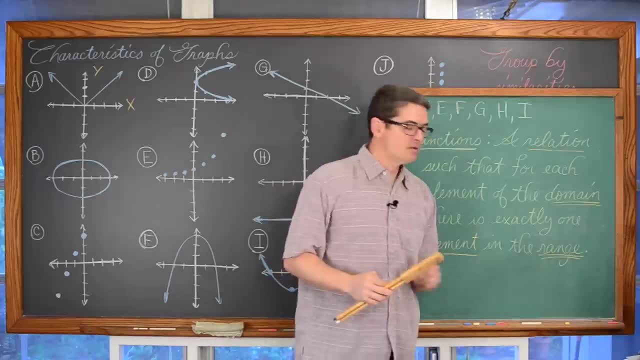 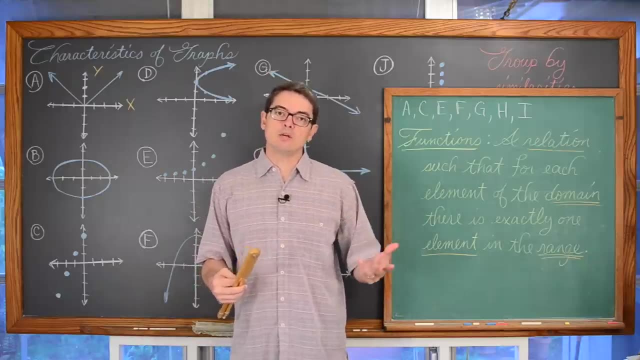 that are included in the graph And range, if you have an equation, is the output value is the answer that you get from your equation. Well, graphically that means, at least on these Cartesian planes, that the range is going to be the y value. 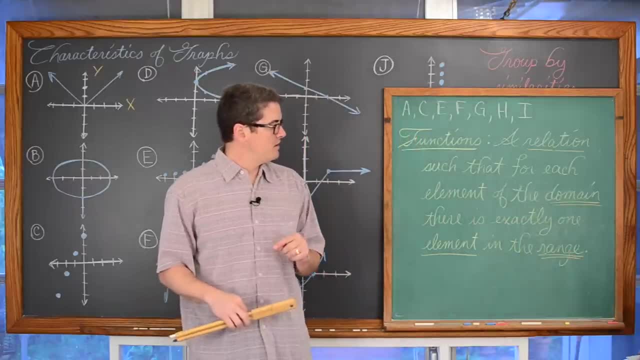 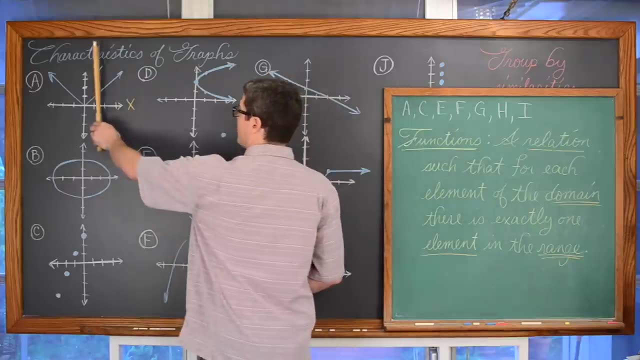 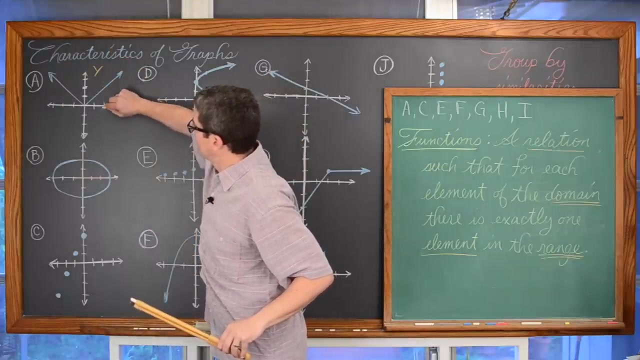 So domain is x, range is y. so for every value of x there is only one y. And again, that vertical line that I am holding up with my compass is representing an x value, and if it is only crossing the graph once, then for that x there is only one y. 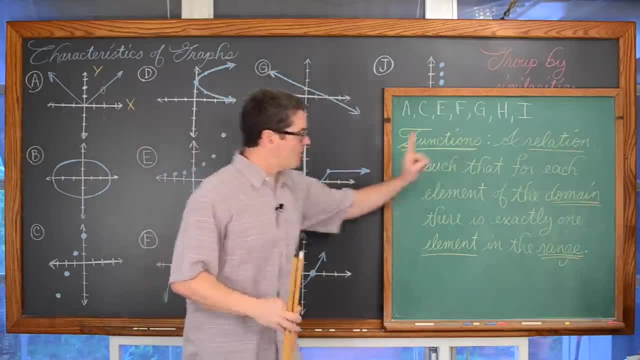 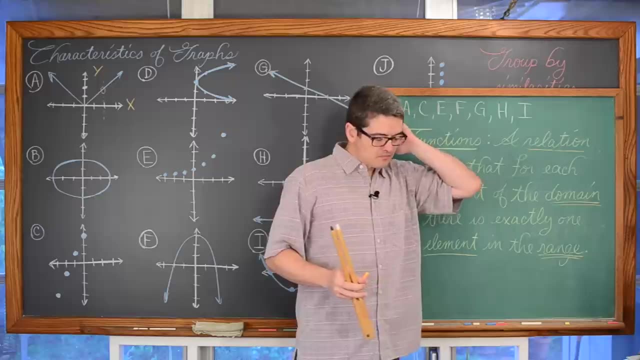 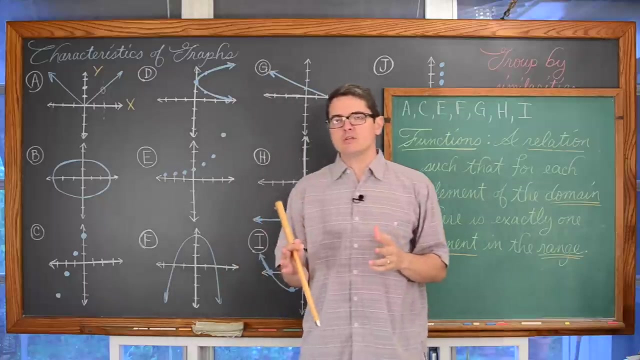 And indeed with a function, every single x in the domain, every single x value can only be paired up with only one y. A relation doesn't have that limitation where every x can only match up with only one y. So for a relation, if an x can be paired up with one y and x can be paired up with more. 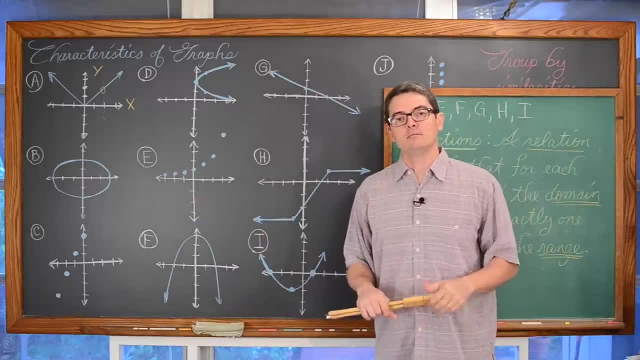 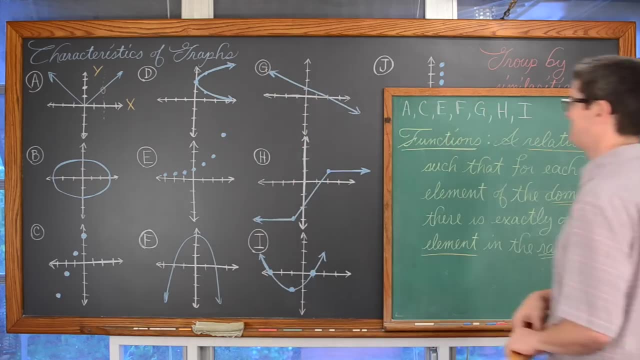 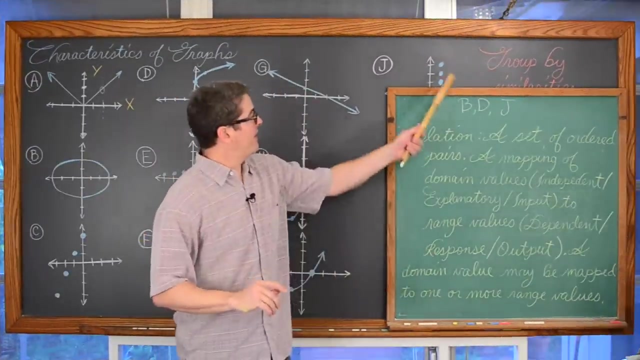 than one y, which of these graphs would be a relation? That will be our second grouping that we discuss. I will have that definition written on the board. No, no, no, no. Graphs of b, d and graph j that I covered up. those are all relations. Again, if I hold up a vertical, 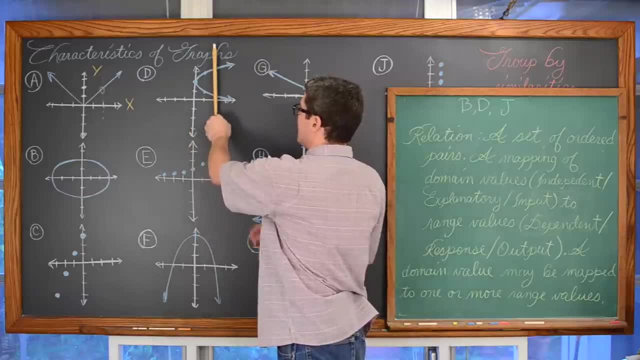 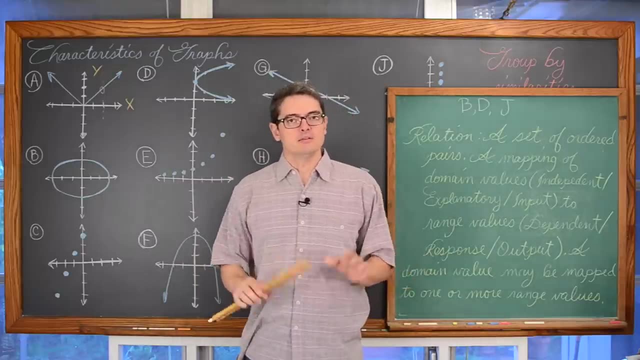 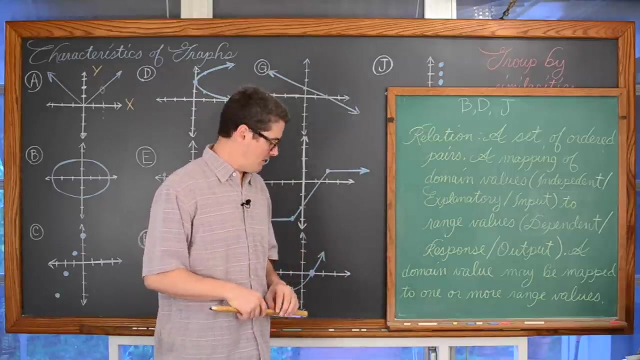 line representing a value of x. in this particular case, that x value is connected with or related to two different y values. Thus it is a relation. Now, a relation is a set of ordered pairs. By the way, an x value can be connected with, or a single x value could have ten different. 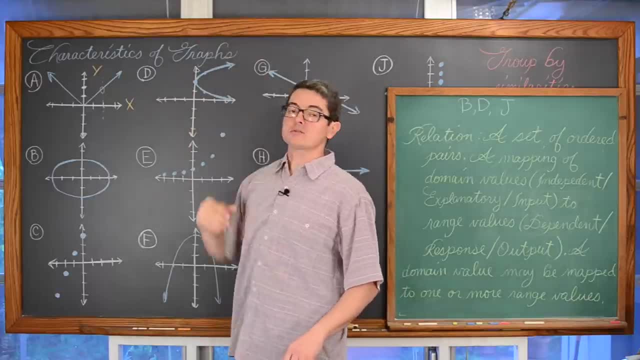 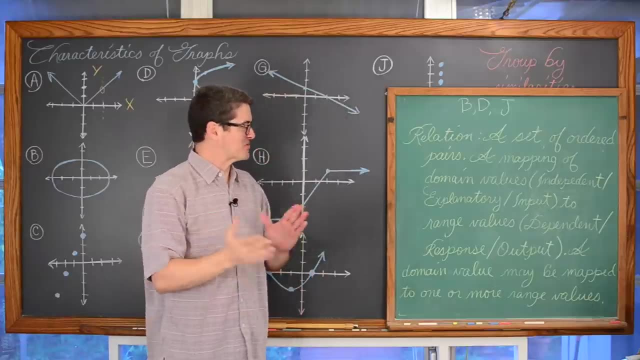 y values that it is related with, if the graph keeps sort of snaking up vertically Like a, Like a sign graph, going up the y axis. if you have been introduced to trig yet, A relation is a set of ordered pairs. Any collection of x- y coordinates that I give you is automatically 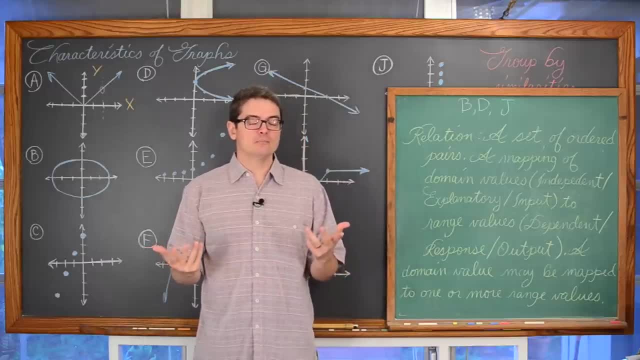 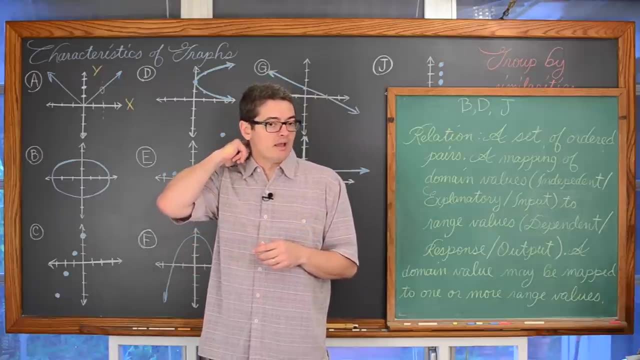 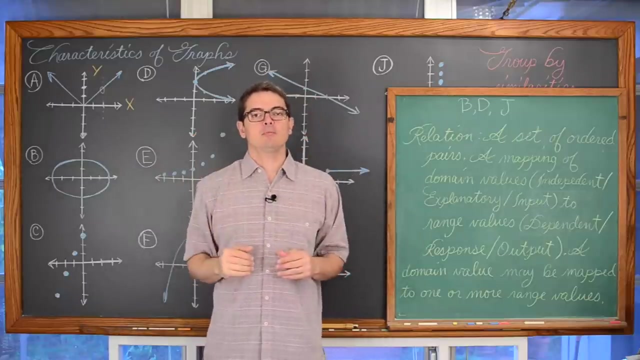 going to be a relation, Then a function is a special type of relation. So think about if you have studied any geometry at all yet. a straight sided figure with four sides is a quadrilateral. If the opposite pair of sides happen to be parallel, well then it is a parallel. 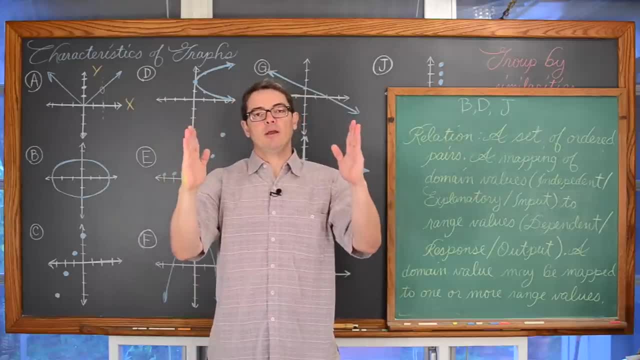 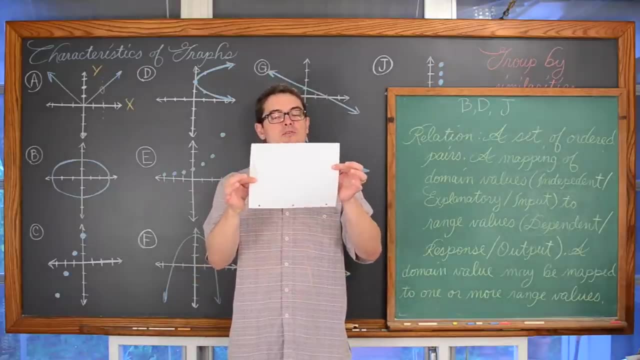 parametric. If the opposite sides happen to be parallel but the corners are right angles, like a piece of paper, then that is not just a quadrilateral, It is not just a parallelogram, it is a rectangle. And then if all four sides happen to be equal, then 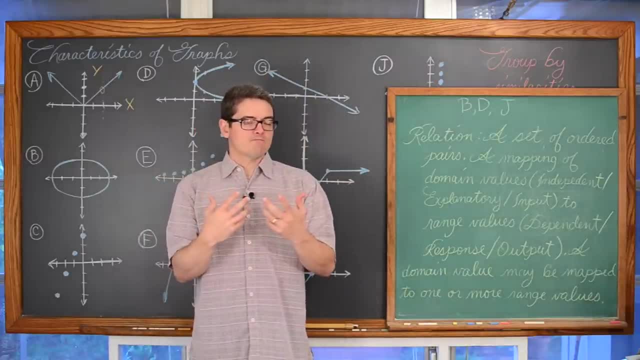 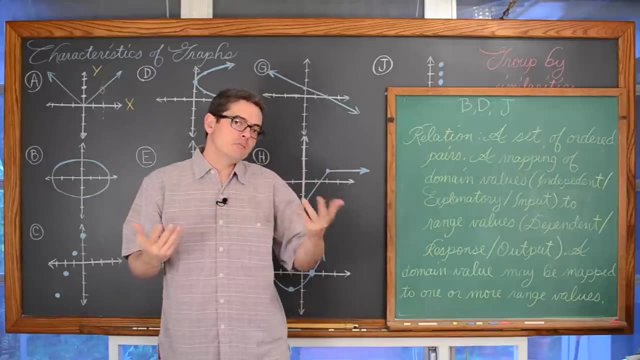 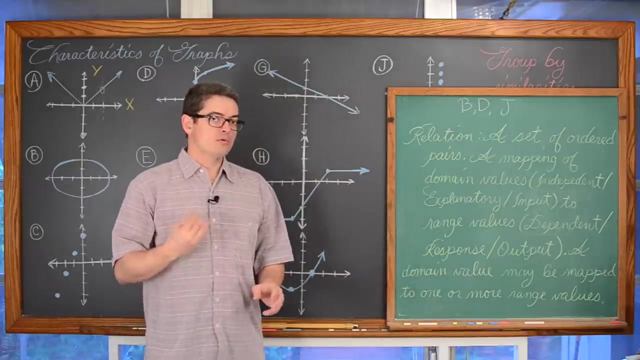 it is a square, So a relationthe difference between a relation and a functionall functions are relations. but for you know, you just saw the previous definition- a function is is a special type of relation, A mapping of domain values. or you could read possibly: 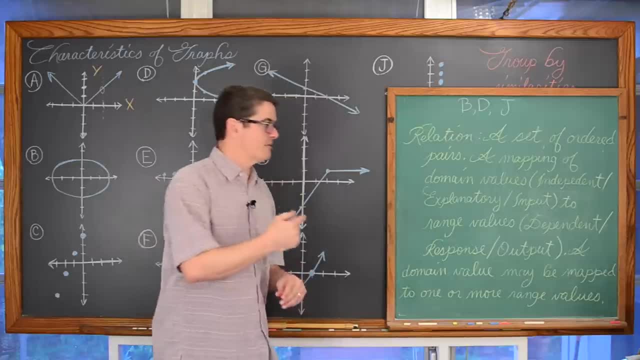 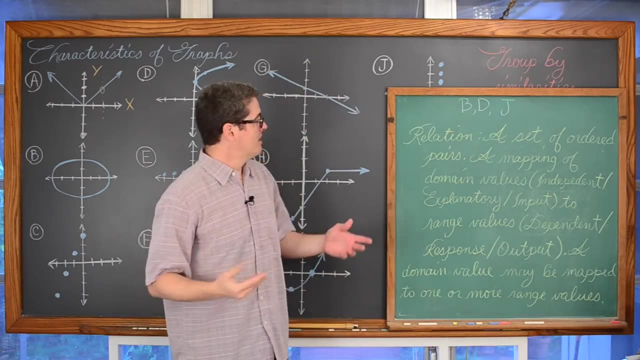 in your textbook or hear from your teacher. independent variable, explanatory variable, the input value, those all say the same thing, At least in terms of graphing on an xy axis. they all mean the x? A mapping of domain values, again, independent, explanatory or input value. 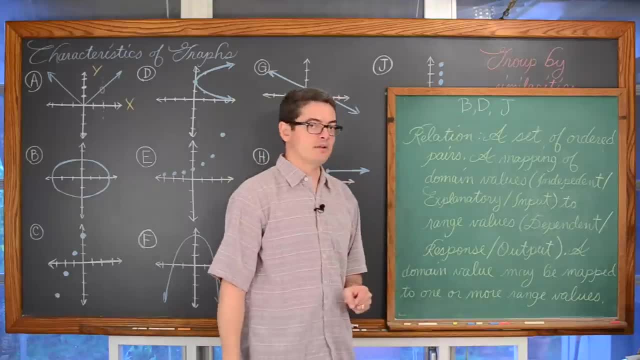 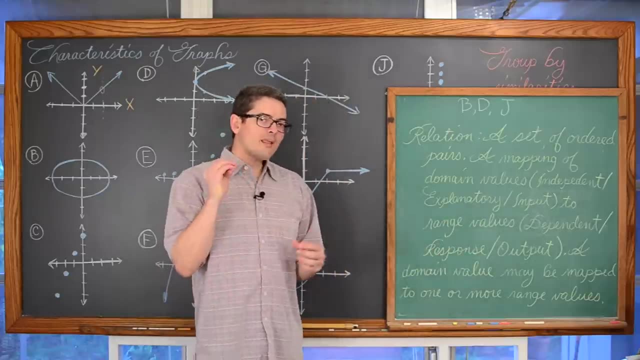 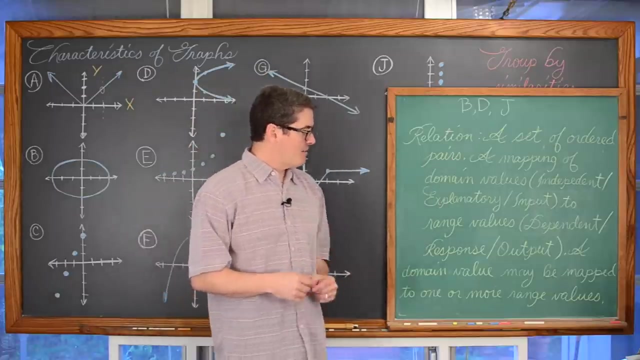 is mapped to a range value, or mapped to a dependent value, or mapped to a response or output value. A little bit more simply stated, without all that sort of alternative vocabulary, a domain value may be mapped to or connected to more than one range value. To make this, 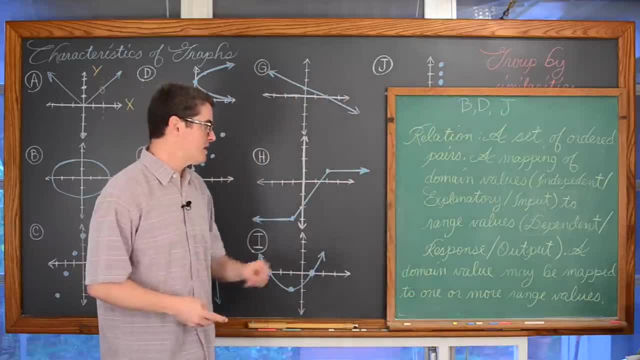 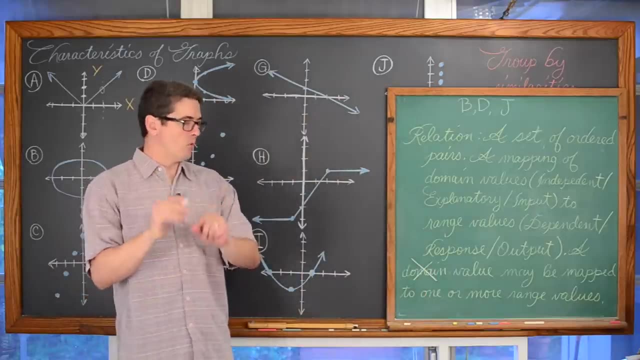 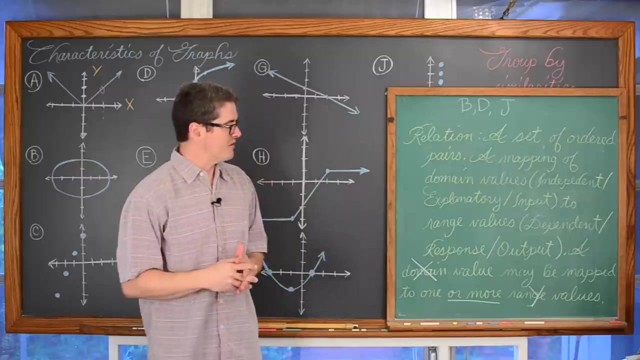 even simpler and write it in terms of, again, graphs: a x value may be mapped to or connected to one or more y value. Now don't just think. focus on the x and the y, because vocabulary is very, very important in mathematics. You. 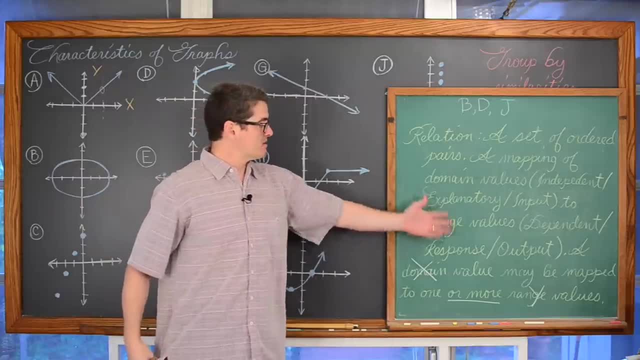 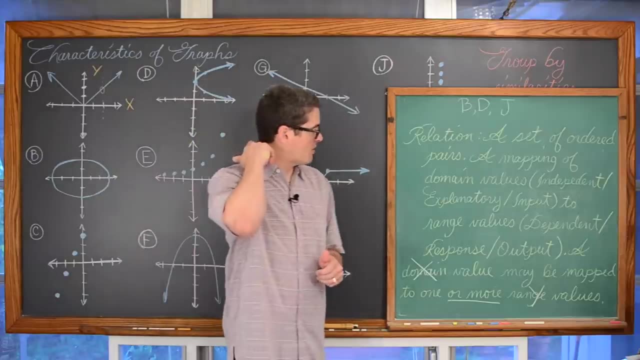 might have a test question or a word problem that uses some of this language, that if you knew the language you could do the problem. But if all you think of is in terms of x and y's, you won't understand how to work out the problem. So we have again this pairing. 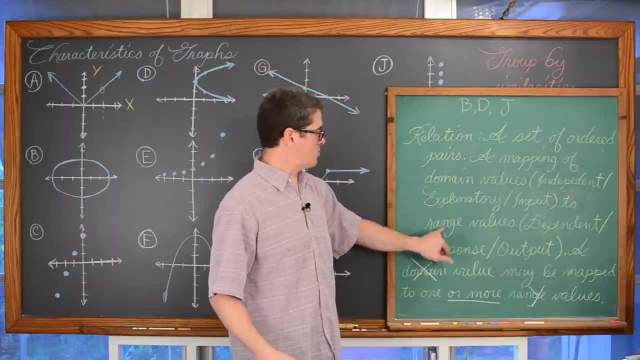 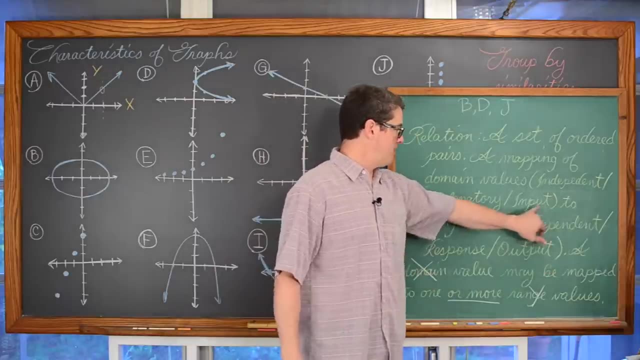 of something could be a domain, range, x, y, independent, dependent. Those go together Vocabulary and response values and input and output. That is how they kind of pair up. That is the difference between a relation and a function, If you want a more in depth. 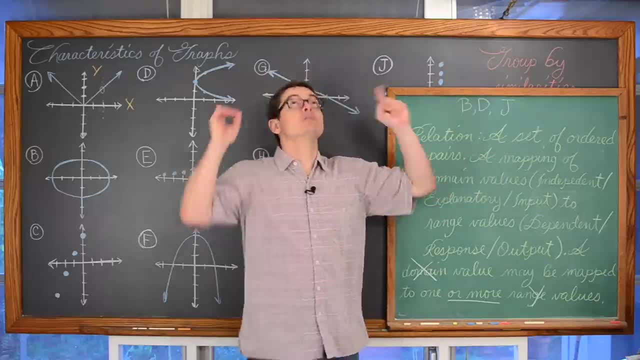 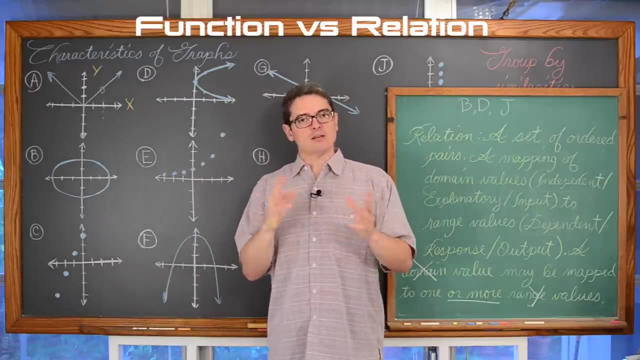 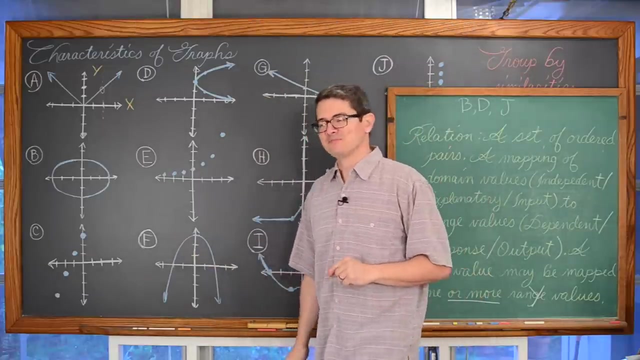 understanding or understand what this idea of this thing called mapping is. check out the link above my head or in the description of the video for a full length introduction to the difference between, and understanding the relationship between, relations and functions. Let's move on to another grouping of these ten graphs. 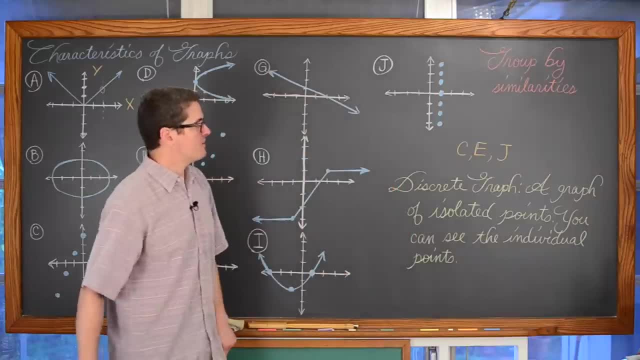 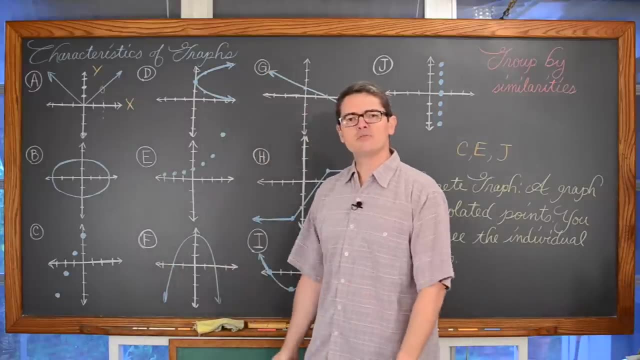 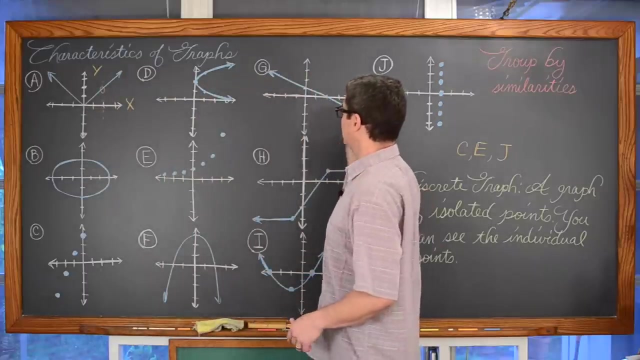 I got you grouping of graphs right there. How about graphs of c, e and j? Excuse me, that would be j, c, e. All those graphs are a bunch of dots, Not? well, not whatever this is called- where all of these lines seem to just sort of go on and I can't see the individual. 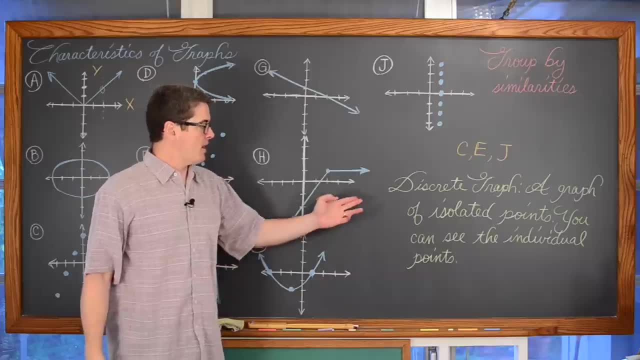 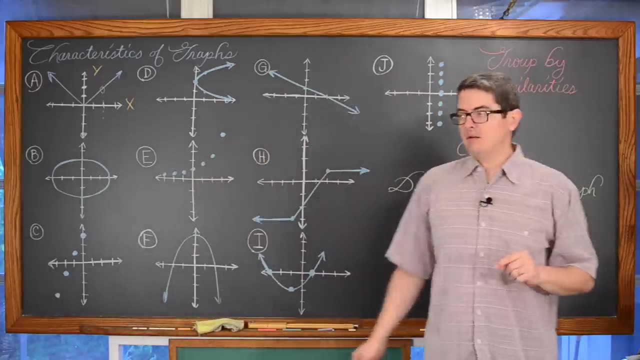 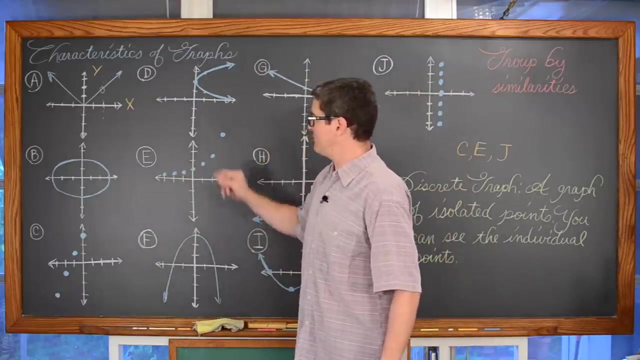 points. Those are examples of discrete graphs, A graph of isolated points, where you can see all those individual points. We are going to be talking about domain and range at the end of this lesson. If I wanted to talk about the domain and range that is included in this graph, I would be just listing: 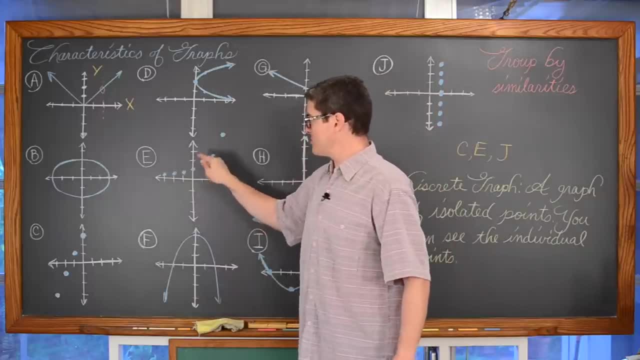 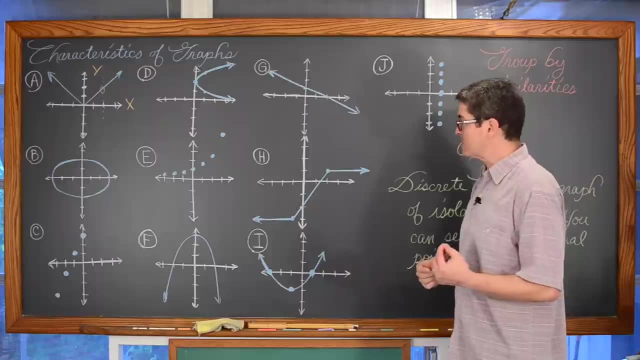 off a bunch of numbers, because there is a dot, there is a dot and there is a dot, or a point, and there is a point and there is a point, and so on, and so on, and so on. Really, all of these graphs are a collection of points, but some of these graphs, the points, 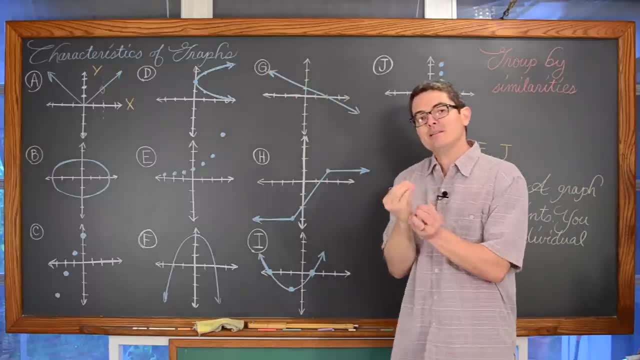 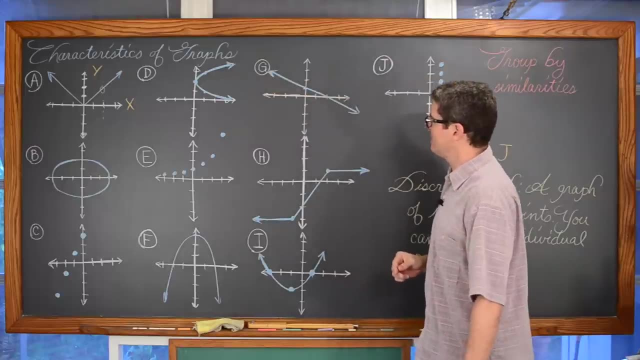 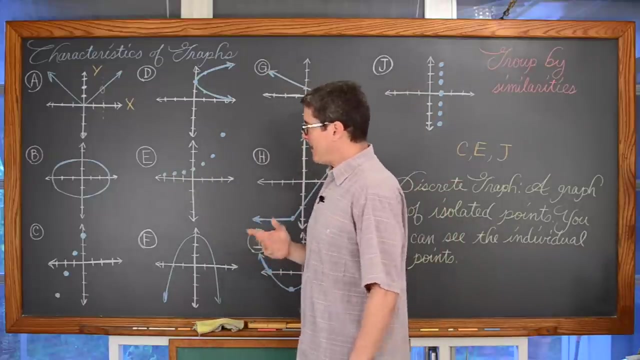 are so close together- They are infinitely close together- You can't distinguish them. Thus, these other types of graphs that we are going to be grouping in our lesson are constructed of an infinite number of points. Here, with a discrete graph, I guess it could go on forever. 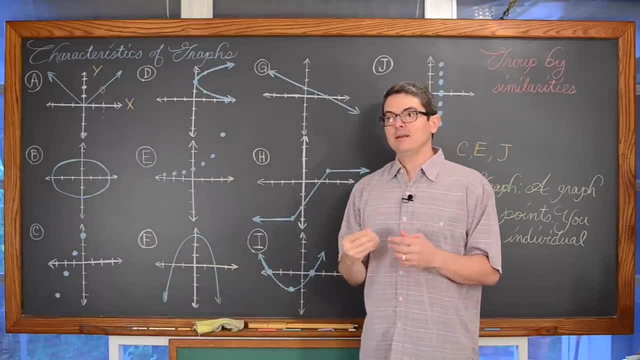 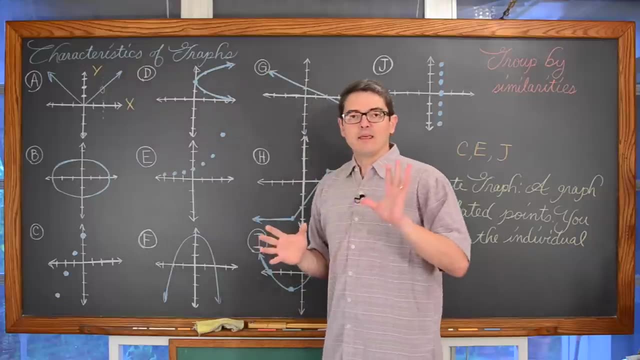 and maybe still potentially involve an infinite number of points, but there is a lot of points that are left out. actually, there are different sizes of infinity. Also, this definition, this concepts of discrete and what is coming up. I will give you a hint: It is a continuation. It is a continuation of different systems. Again, that is a concept of discrete. and what is coming up? I will give you a hint: It is a continuation of the discrete. If you want to do this, that is a follow up question of having no definite answer. so, if you want to, 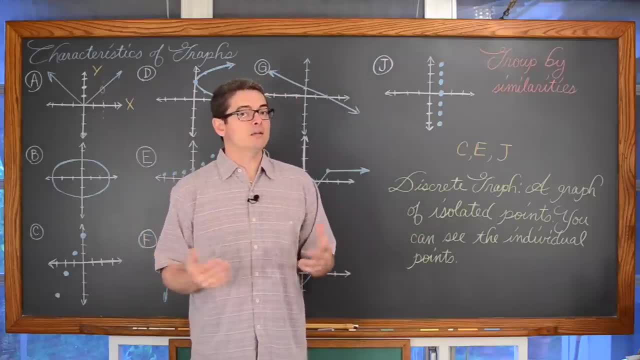 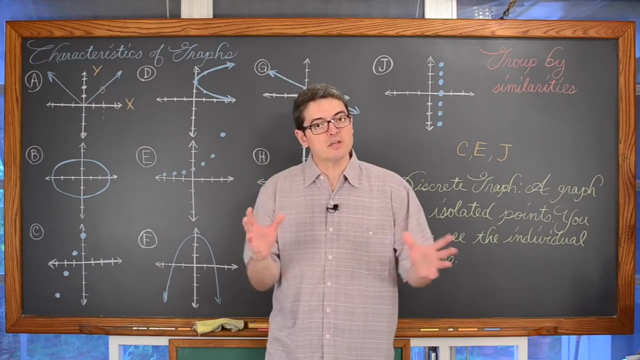 get that, you will have to go to the next slide. I will just drop that and get back to you. I will just continuous graph. that vocabulary will come up again in statistics and have a lot of meaning in those application problems, those word problems. So let's move on to another grouping. 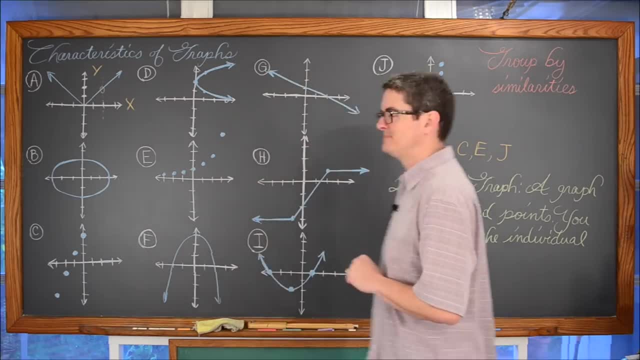 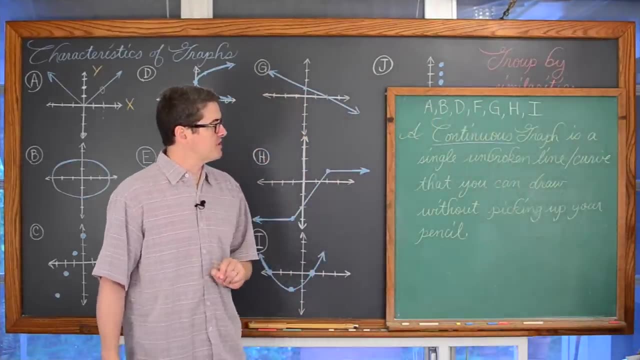 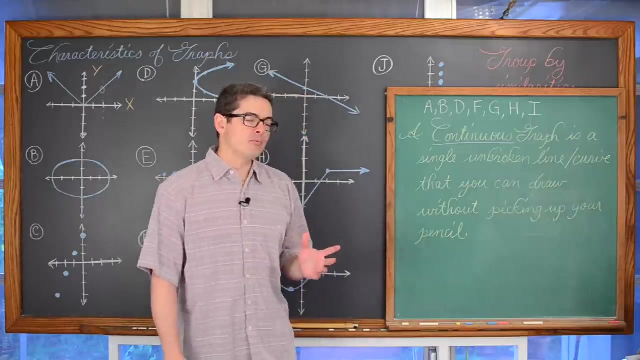 of graphs which are not discrete. Well, if a graph isn't discrete, it's going to have to be continuous. A continuous graph is a single unbroken line or curve that you can draw without picking up your pencil. If you want to know how to prove if a graph is continuous, 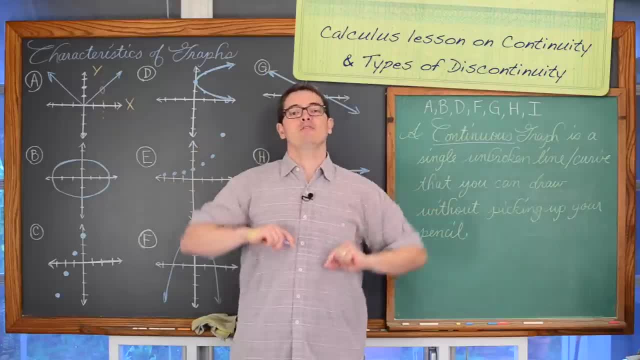 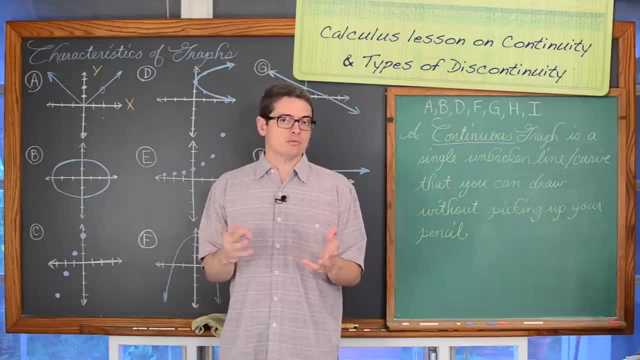 at a point using some fancy calculus stuff. that link will be above my head. Just one example of where this definition will come up again. and I said, in statistics you will learn something called a discrete variable and a continuous variable as well. So these 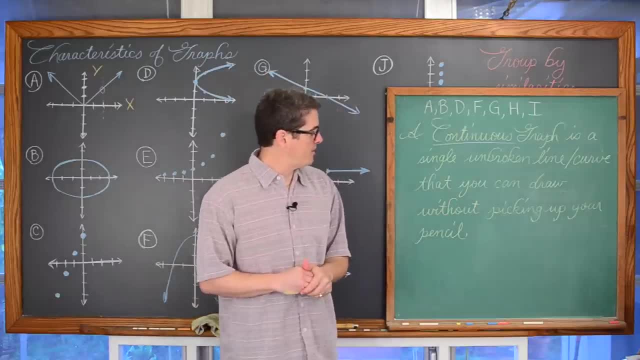 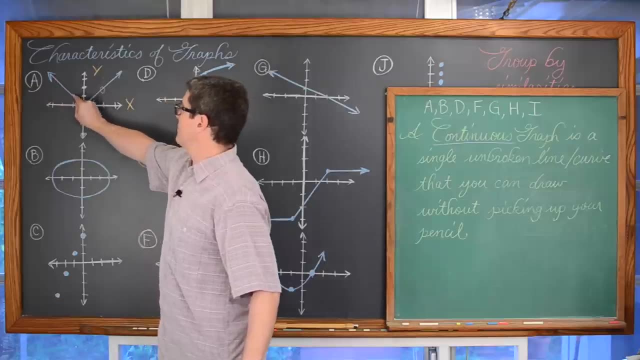 definitions, and this is only applied to graphing, but they come up over and over again in your math studies and you can draw these without picking up your pencil, So I can drag along this line- there is sort of a sharp point there- and go in another direction, but I can. 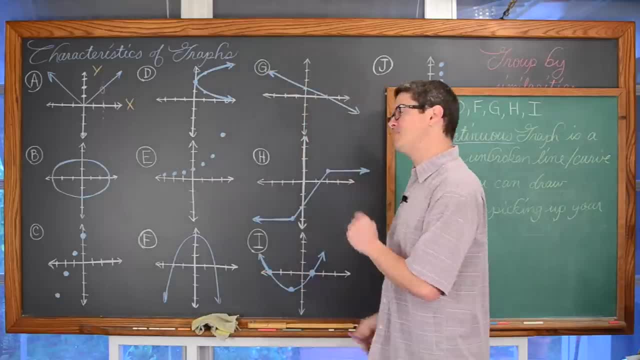 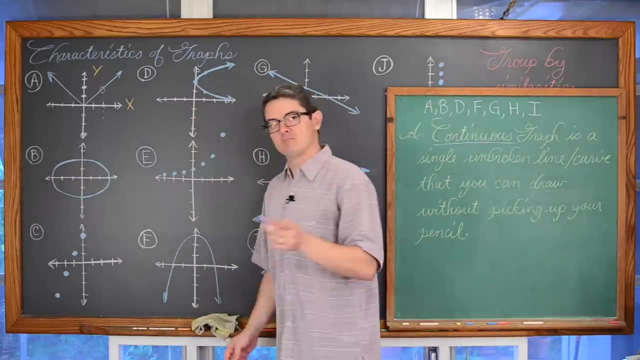 draw that entire line. Well, really, it's a linear absolute value graph. without picking up my pencil, I can draw this in ellipse, which, by the way, again that ellipse. first time I've said that would fail the vertical line test and thus this is a relation and not a function. So I did. 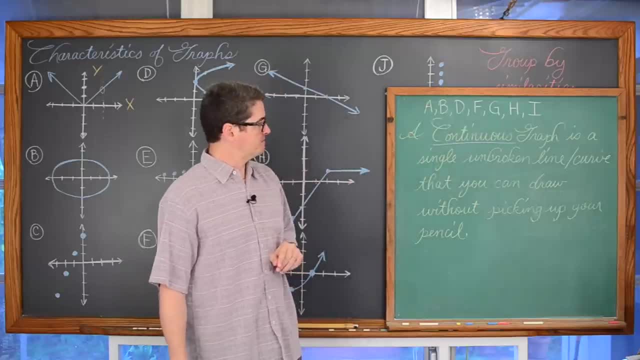 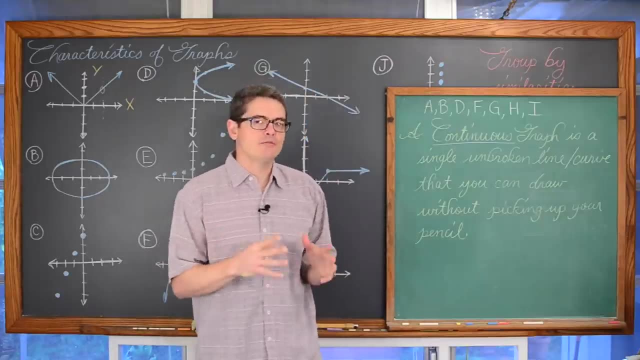 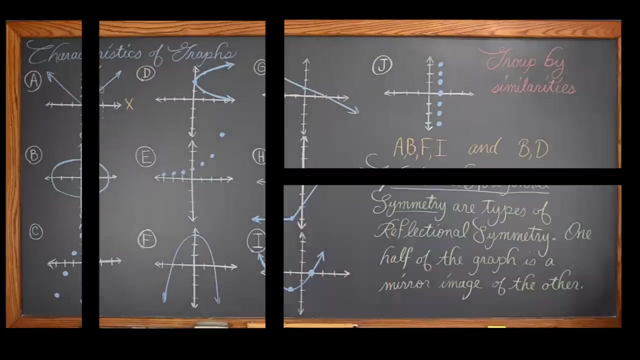 mention, it's a continuous graph, not a continuous function, And that grouping is A, B, D, F, G, H and I. So let's move on to a different vocabulary here, vocabulary word and a different grouping of these ten graphs. Two more groupings of these graphs are groupings of A, B, F. 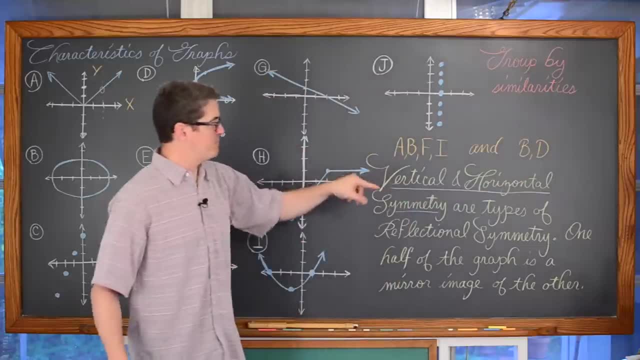 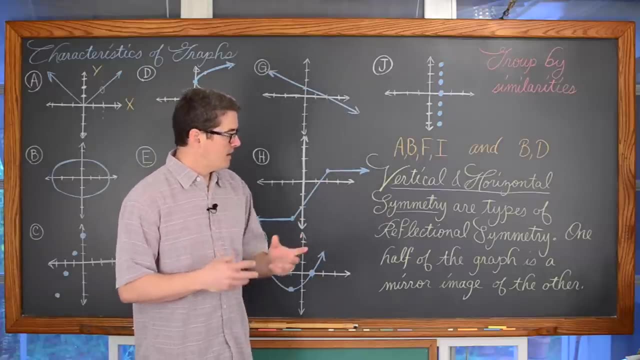 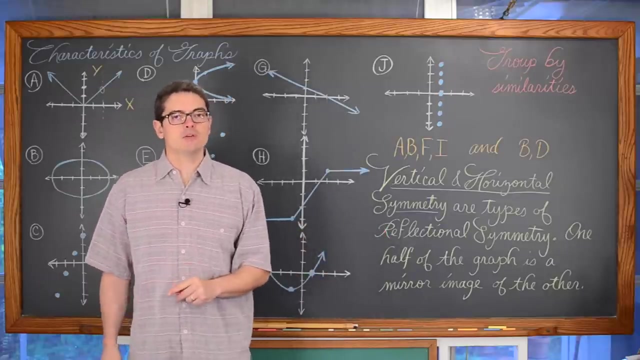 and I, and B and D, And you'll notice that graph B is showing up in both of these groups. Well, these groupings represent vertical and horizontal symmetry. This is a type of reflectional symmetry, One where one half of the graph is a mirror image of the other. So you can. 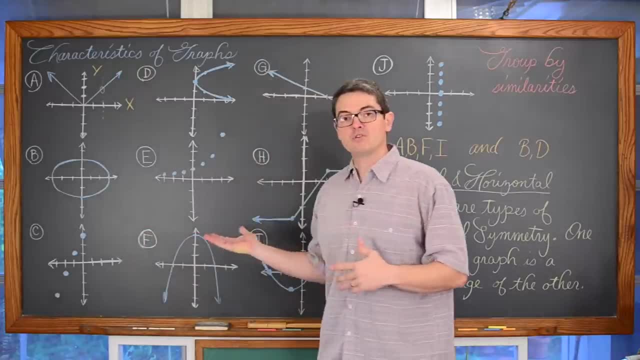 just draw a line right through the graph And then you can draw a line right through the graph. Or you know, if this were a big sheet of paper, right, I could fold the paper and then kind of like, look through it and the graphs are going to perfectly line up. 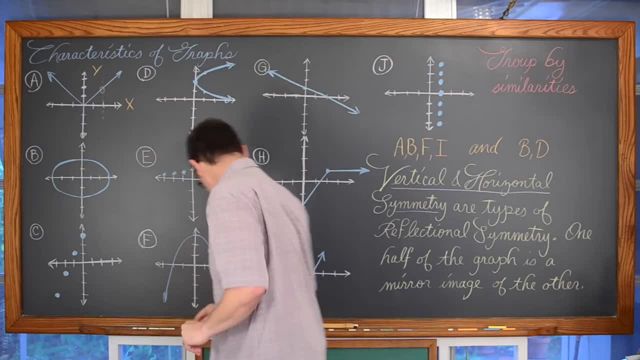 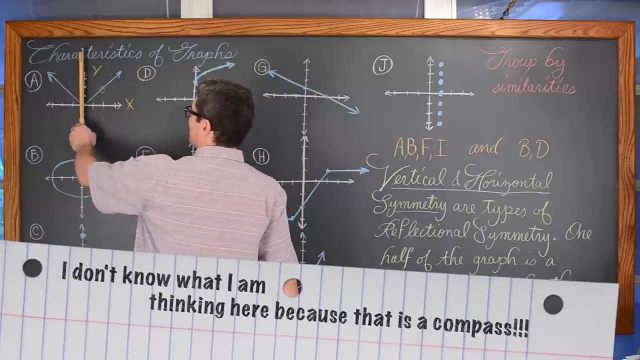 with each other. So when I look at A and where's my compass at here- Or not my compass, but my protractor, I think I called this my compass earlier in the video. Anyway, if I put a vertical line there and I fold the chalkboard on itself, this line is going to exactly. 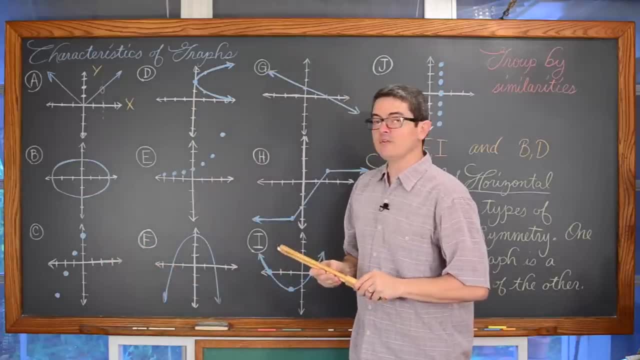 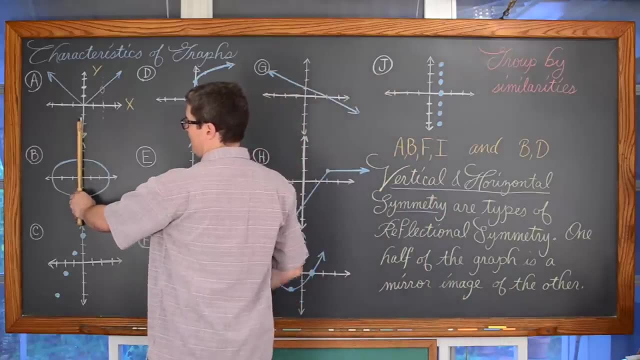 if drawn correctly, line up on itself. on the other side B, you'll notice that B is in both of these groups. Well, I can put a vertical line here and this will fold over and line up exactly to the left, Or I could put a horizontal line. 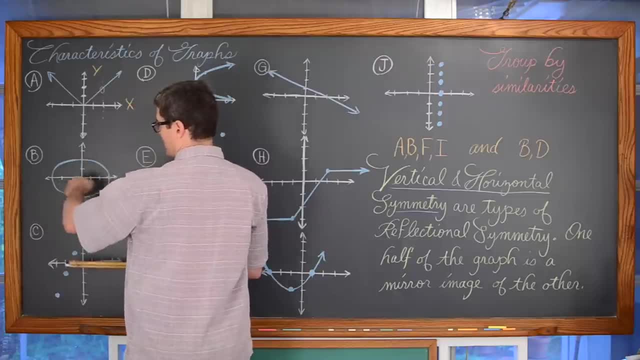 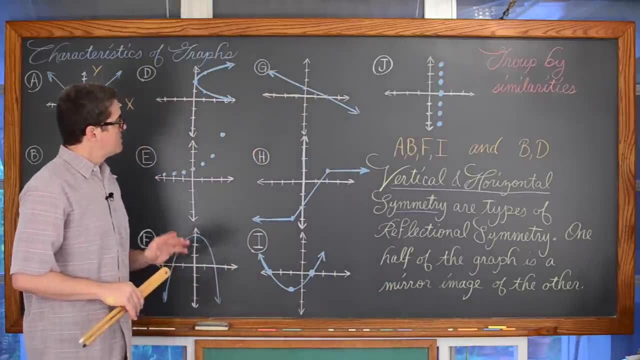 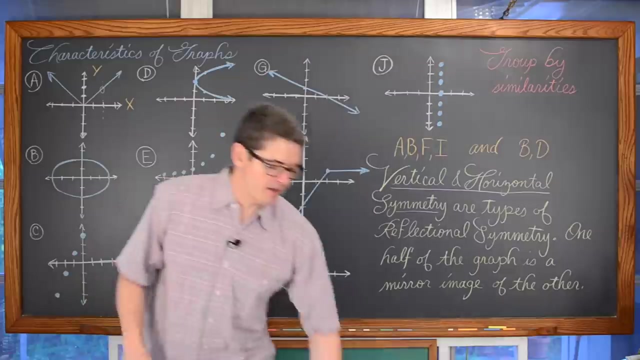 and maybe fold the bottom up and, if drawn correctly, that bottom part of that graph will lie right on top of the top half of that graph. Now, just to make sure that you understand that this horizontal and vertical symmetry doesn't have to be the x and y axis we've 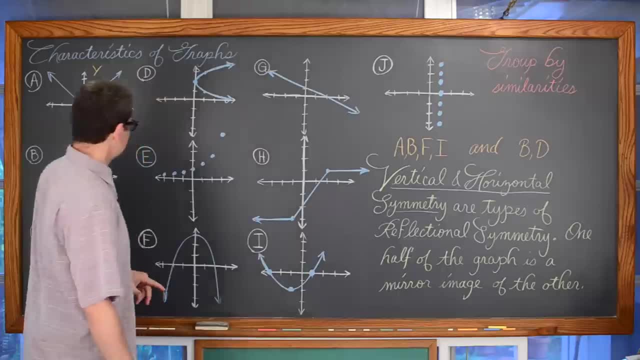 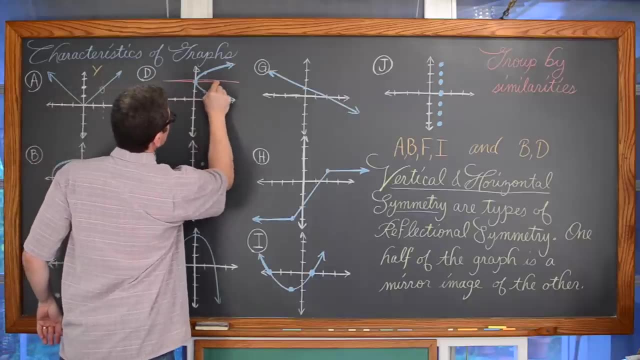 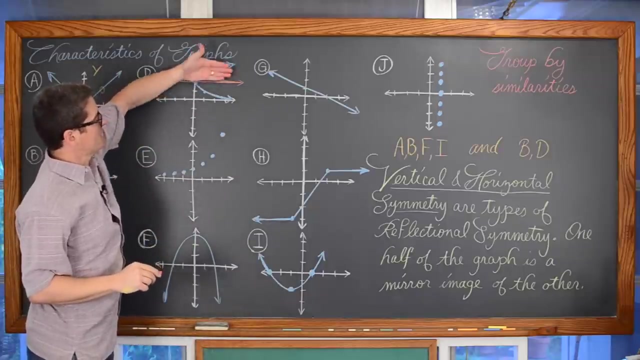 included the graphs of D and I Indeed here the horizontal line. let's go ahead and put that in here, this horizontal line, maybe draw it a little better than that. if I were to fold, that probably should be a dotted line, but if I were to fold along that line, 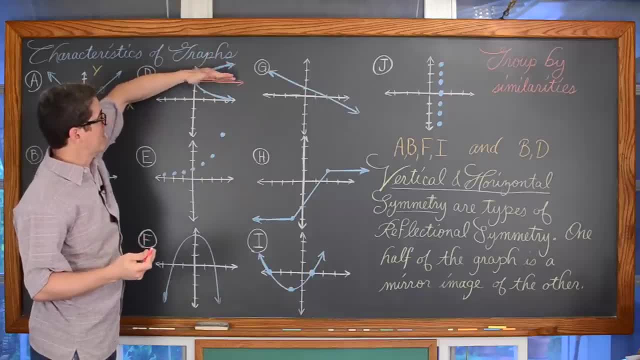 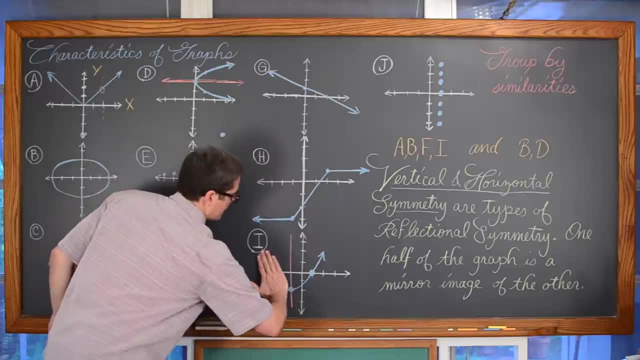 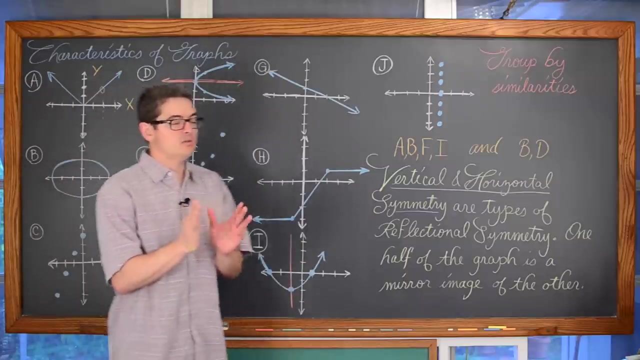 the top half of this parabola would line up exactly with the bottom half. And same thing here. if I put a vertical line through, x equals negative one. this left side, when folded, if drawn exactly correctly, would line up right on top of the right hand side, And that. 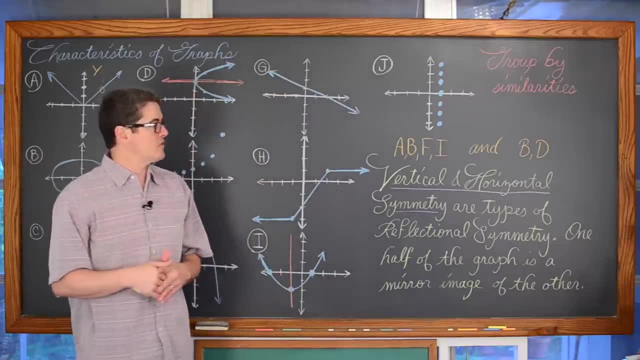 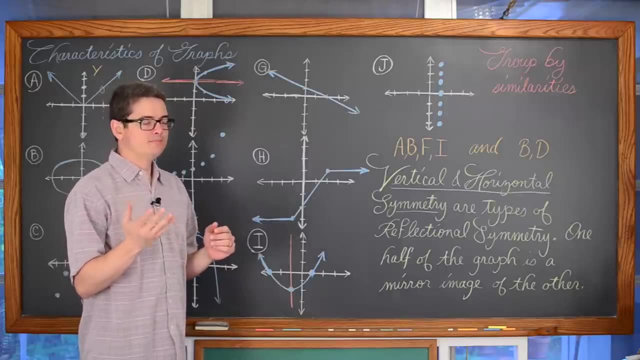 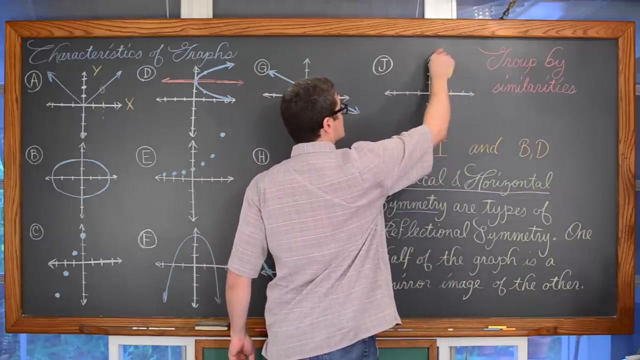 is what you're going to look for when identifying lines of symmetry. Now, I didn't include J simply because the points well they're. I don't know, maybe you could argue that they're symmetry or not, but if you draw a vertical line through, you know that sort of line. 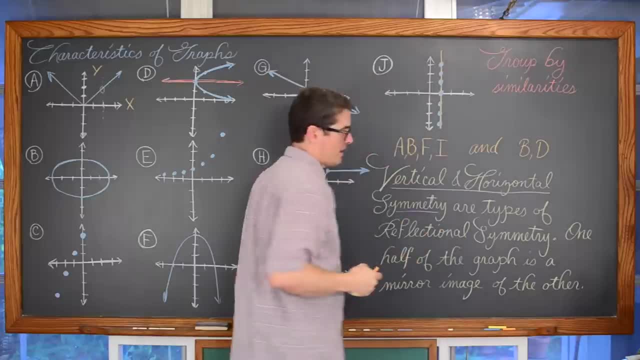 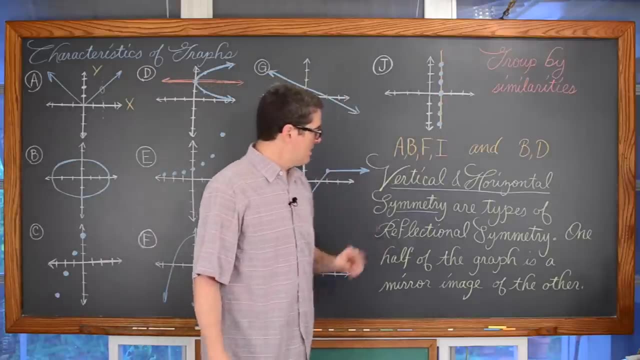 is the graph itself. There's nothing to the left or the right, There is no left and right halves that are mirror images of each other, except that there's nothing to the left of the line and nothing to the right. So let's move on to- let's see here- the next grouping. 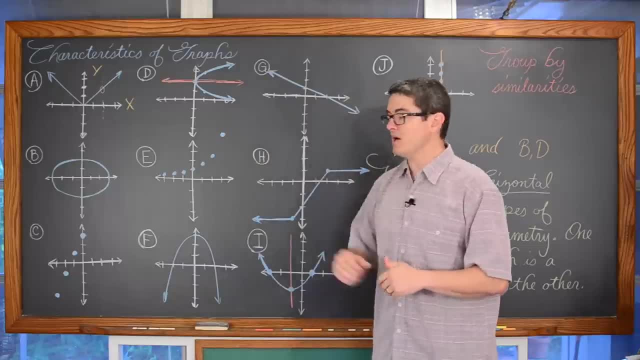 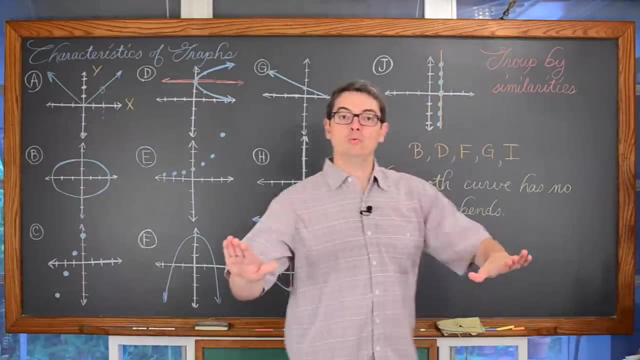 that I'm going to be doing is smooth curves. So what curves up here are smooth? No, no, no, no, no. Smooth curves have no sharp bends. So in this group I'm including B, D, F, G, 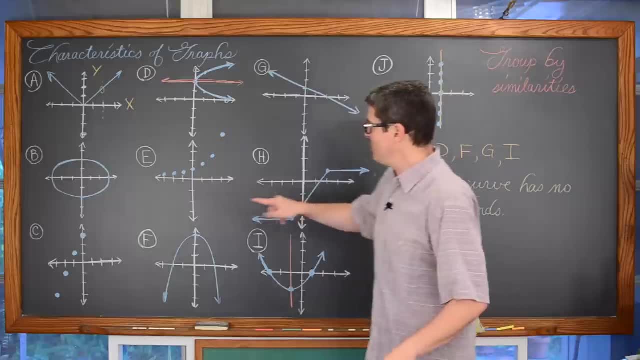 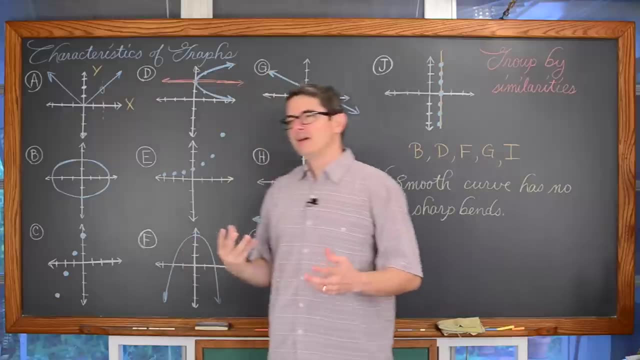 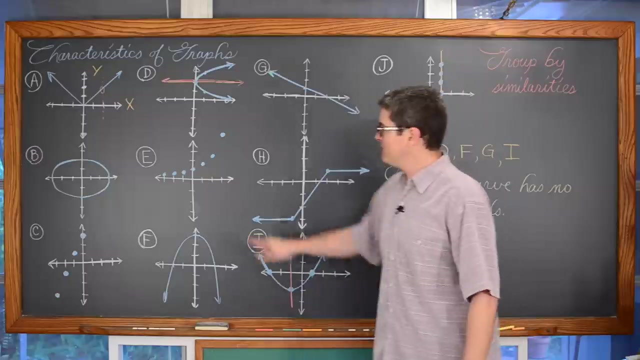 and I, Depending on what your teacher wants, I guess maybe you could include these curves here that are made up of a discrete number of points, because there's no sharp bends. But I have a little bit of a problem including those because, well, it's not a continuous graph, But these are forming a smooth arc or a straight. 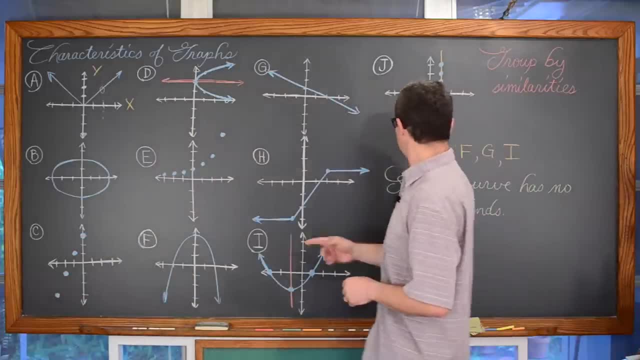 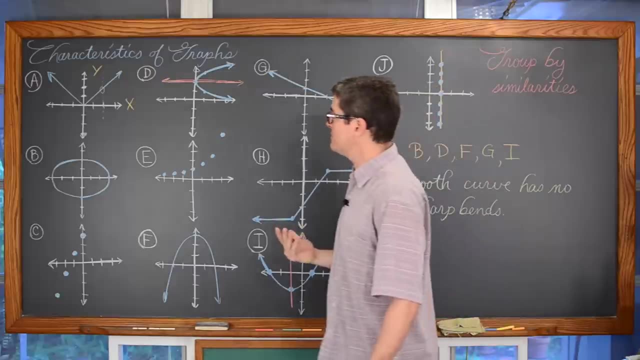 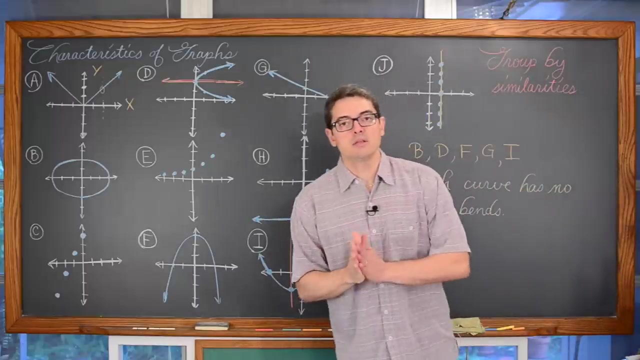 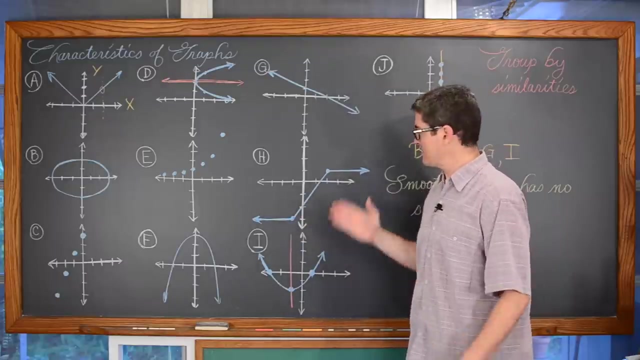 line. I'm only including the continuous curves of, again, B, D, F, G and I, Simply no sharp bends. So I'm including these A and H that have two sharp bends in those. By the way, this is an example of a piecewise function, because there's three straight line segments that constitute 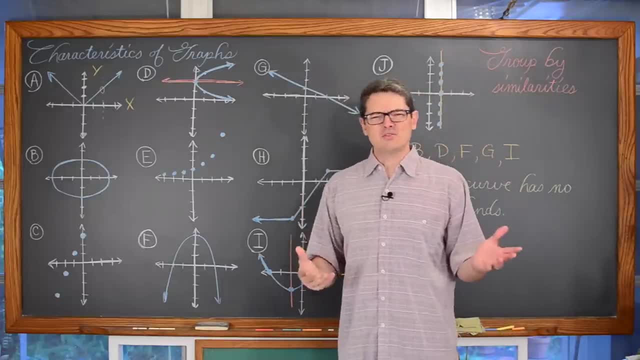 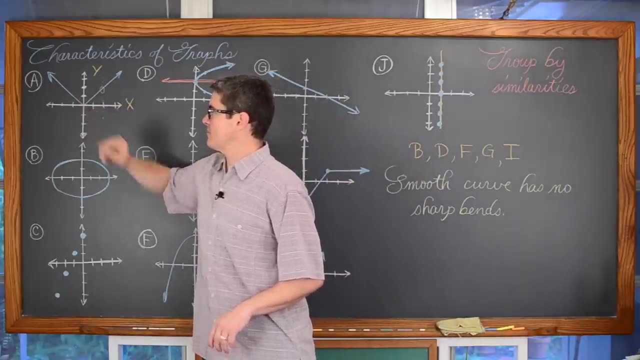 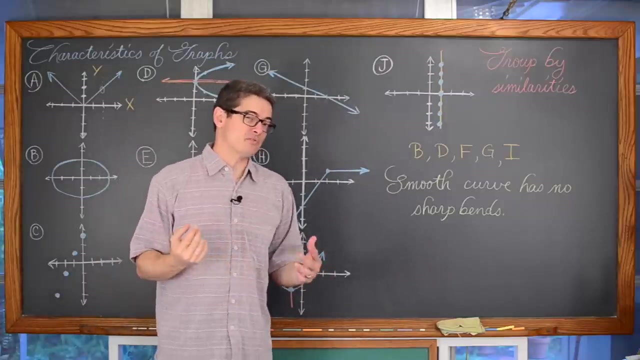 this entire graph. We're going to be talking about piecewise functions not too far from now. Again, this is a graph of a linear absolute value function that has a sharp bend at the x value of zero. This is only definitions based off of drawing I can just see. is there someplace that I could? 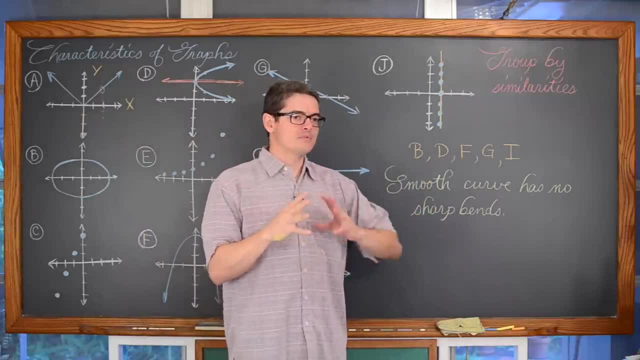 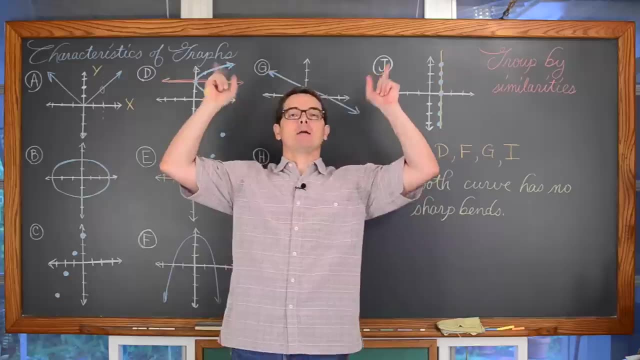 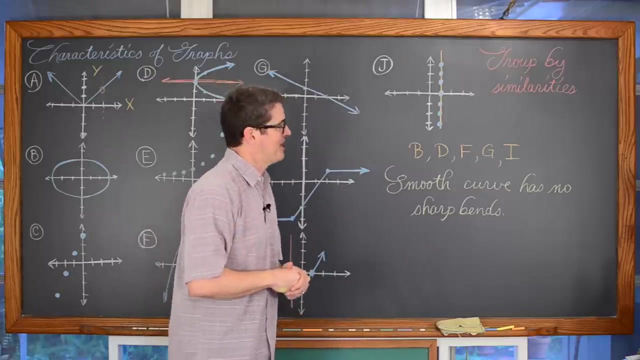 hurt myself on that sharp bend. There's a much more sophisticated way of proving if a curve is smooth at a point, involving calculus. That link is above my head or down in the description of this video. if you want a little calculus in your algebra lesson, Ok, so now. 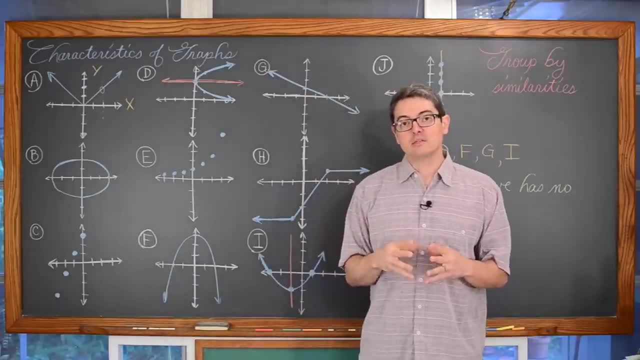 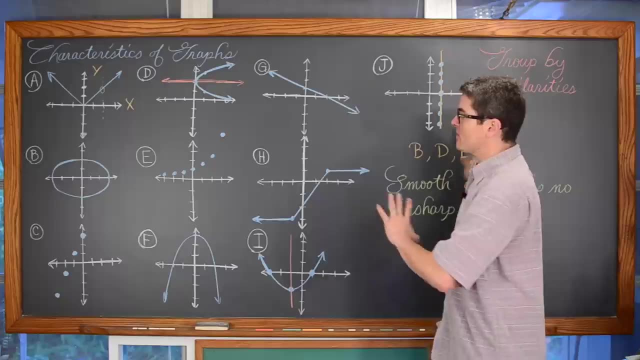 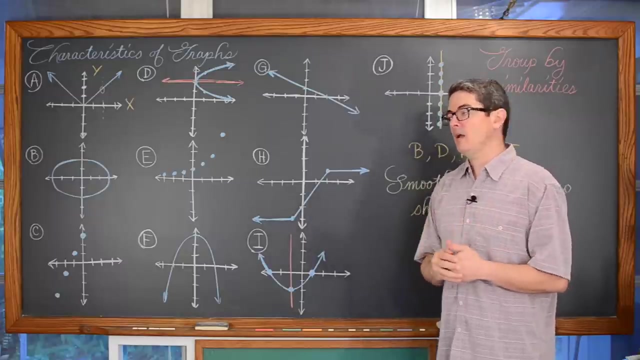 we're going to move onto what an increasing and decreasing function is. Seventh equation: function is Now. I am going to erase all of this and include all of the definitions up here at once, Then include an example where we identify intervals where a function is. 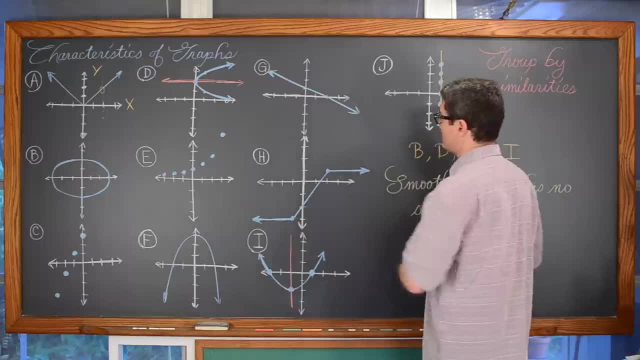 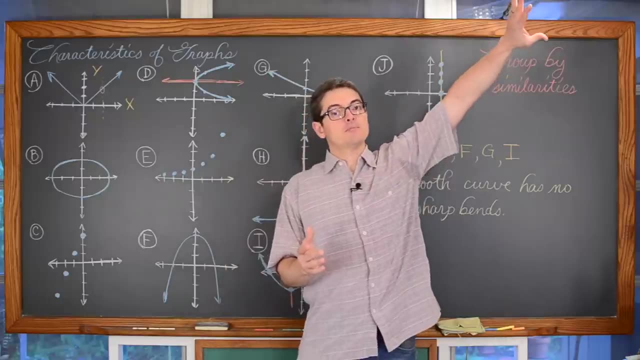 increasing and decreasing, But just verbally. before we get on to that, because we have all of these nice graphs up here already. A function is increasing. if, as you read it left to right, you notice that it is moving up to the right, I will give you a real definition in words. 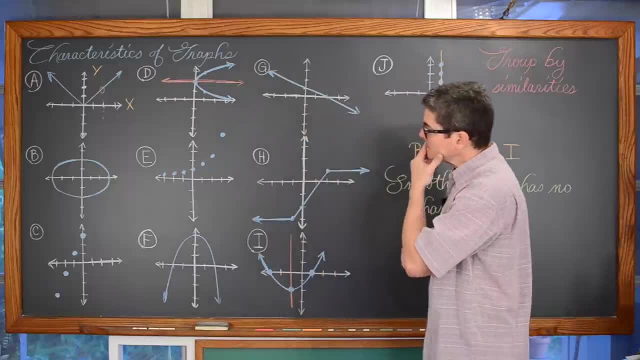 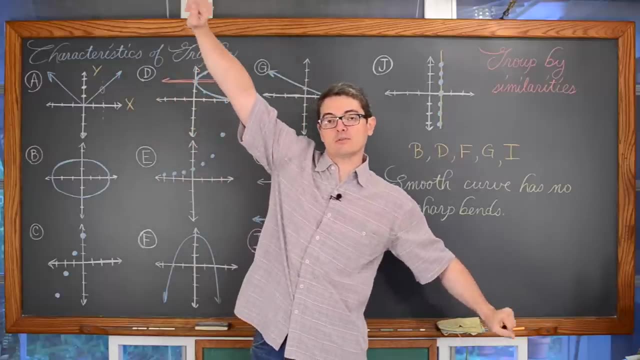 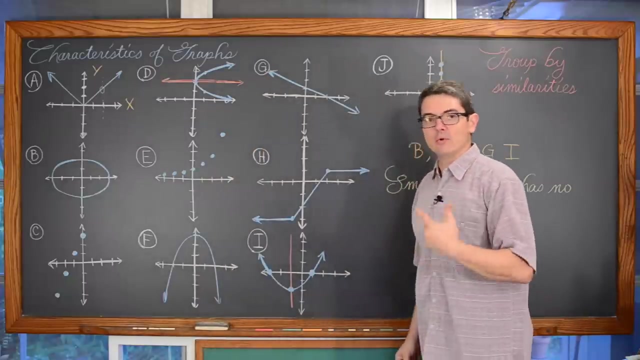 in a second Graphs that are going up to the rightoh a graph, when it is decreasing, is going down to the right. This is sort of like a decreasing line and an increasing line. You read graphs left to right like we read our English books. This graph is both decreasing. 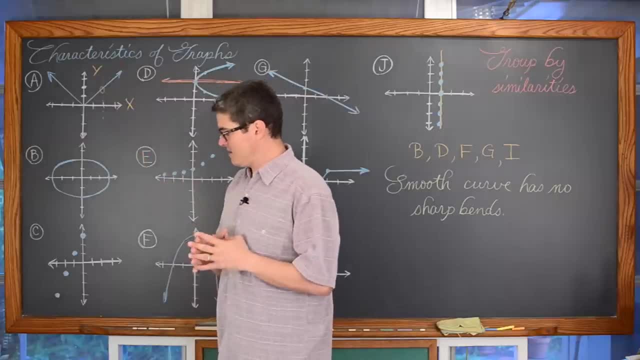 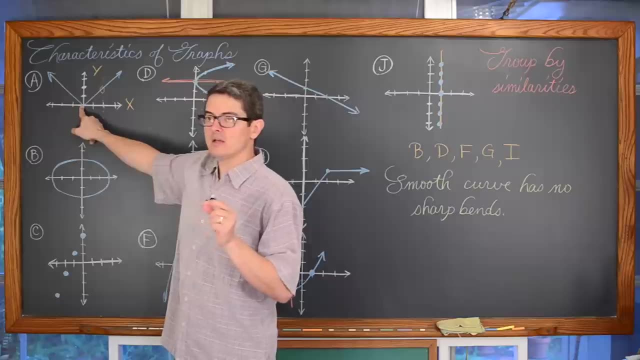 and increasing over two intervals. That is what I want to formally teach and have written definitions. on the next screen It is decreasing from negative infinity down to zero. There is a sharp bend at zero, so it is decreasing as you approach zero. Then, from not including zero but just to the right. 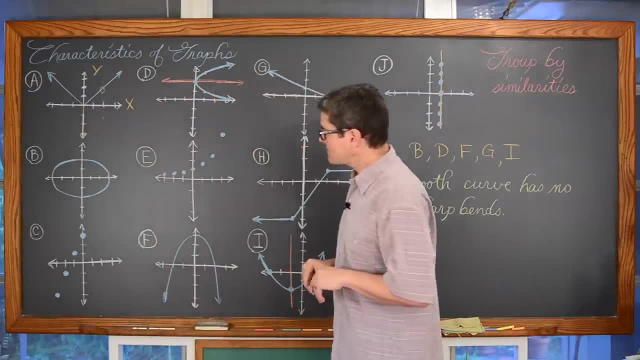 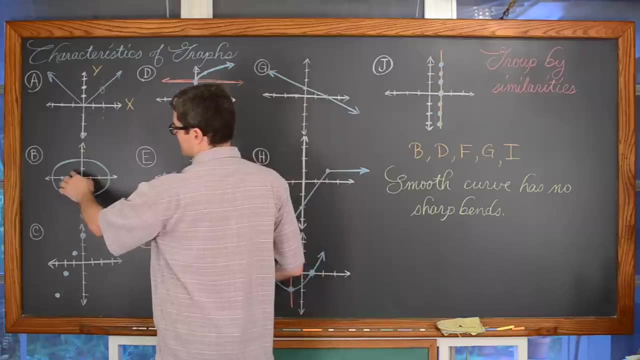 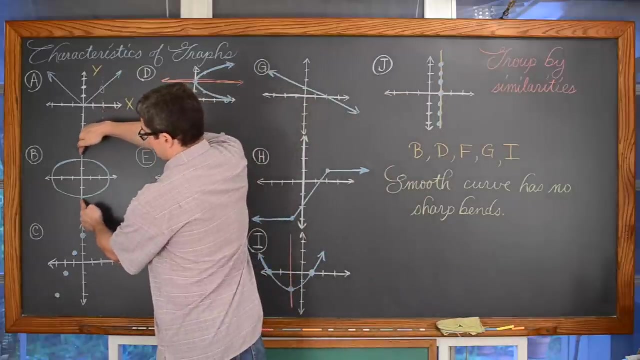 of zero and then on to infinity. it is increasing. This not being a function, it is almost like you would have to break this graph up into quadrants, So I don't really want to talk about increasing and decreasing there, Because, say, from zero to, 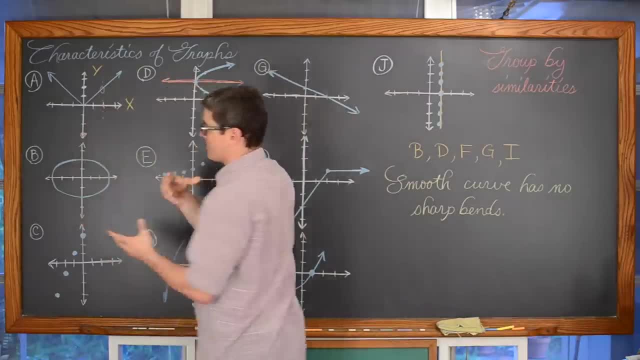 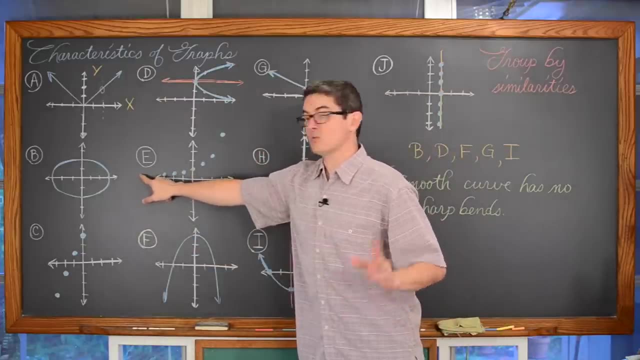 3. the graph is going up to the right at the same time as it is going down to the right, because that is a relation and not a function. This graph is all the way along. Now. it is a bunch of individual dots that are discrete, But as you go to the right, these dots are. 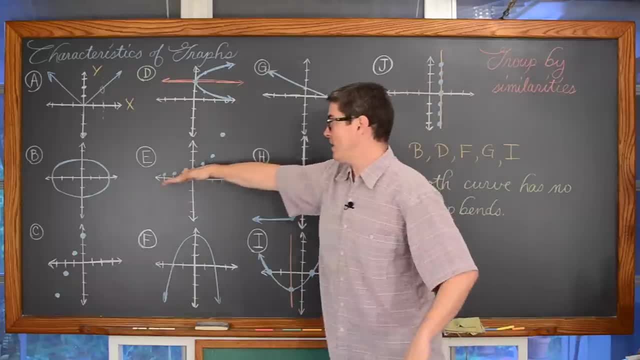 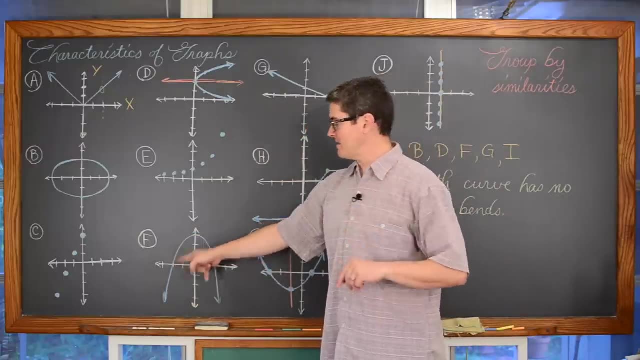 getting higher and higher or farther above the x axis. The y values are increasing, So that is increasing. This is going up as you read left to right. I see there is an arrow pointing down there. But as you read left to right, this graph is going up, so it is increasing. 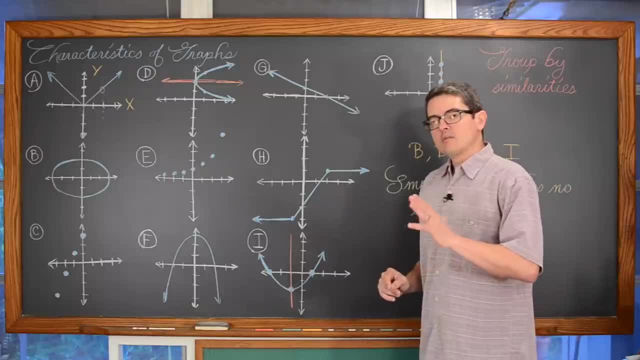 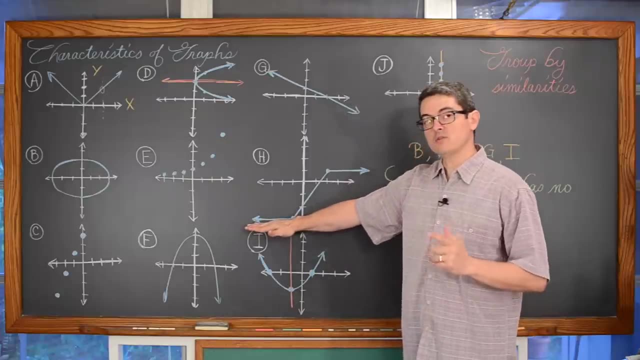 and then it starts to decrease. We have talked about this vocabulary of increasing, decreasing and constant in a previous algebra lesson. Here we have a portion of this graph, this piecewise function that is constant. Then it rises to the right, so there is an interval. 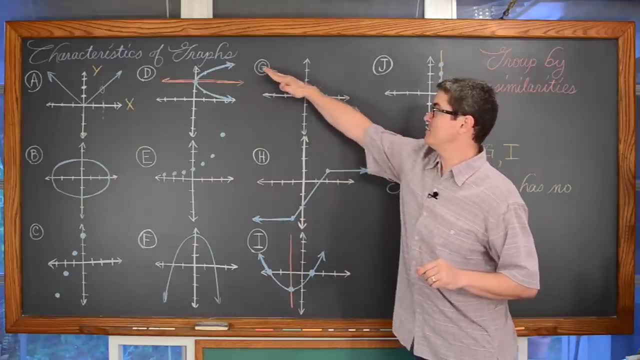 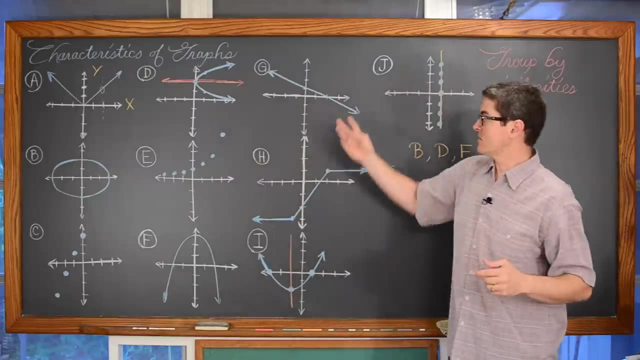 in which the graph is increasing and then it is constant again. This graph is decreasing through its basically forever, throughout the entire domain. It is falling to the right. That is called monotonic decreasing, if you want to be specific. So let's get this graph. 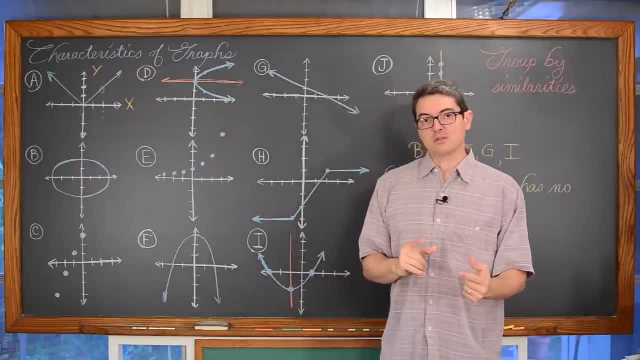 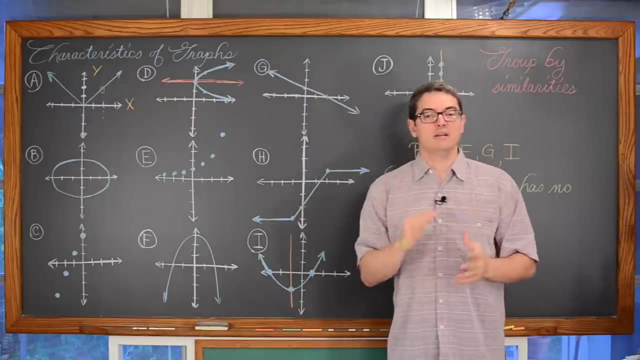 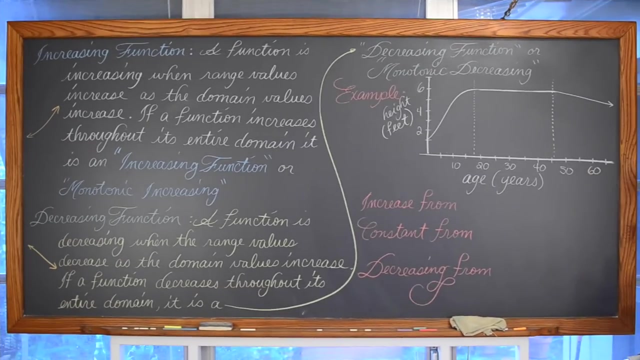 out of the way, Write these formal definitions of increasing and decreasing on the board and get a graph up here where we are going to identify and put it in writing what I have just done here verbally, Identifying intervals where a function is increasing or decreasing. 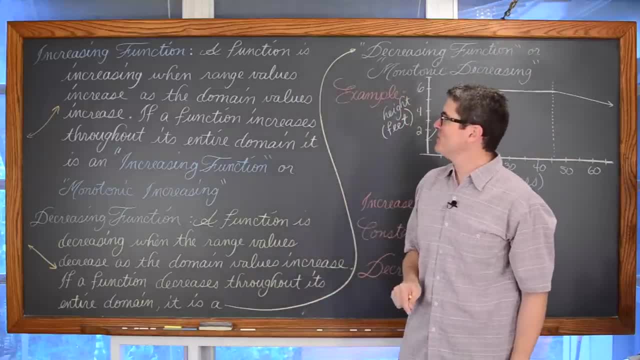 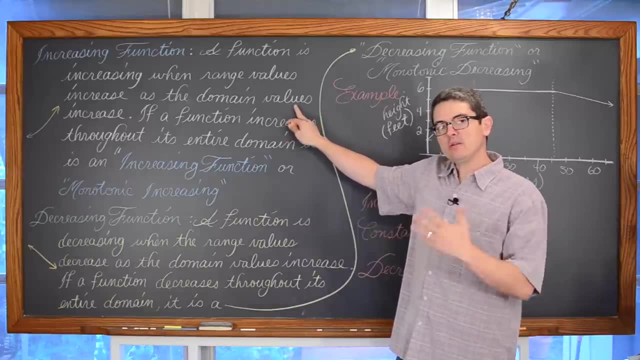 Increasing function. BAM. A function is increasing when the range values, the y values, increase. as the domain values, the x values increase Again. you want to read this graph. as you read these graphs left to right, As the x values get bigger, you are going to the right If 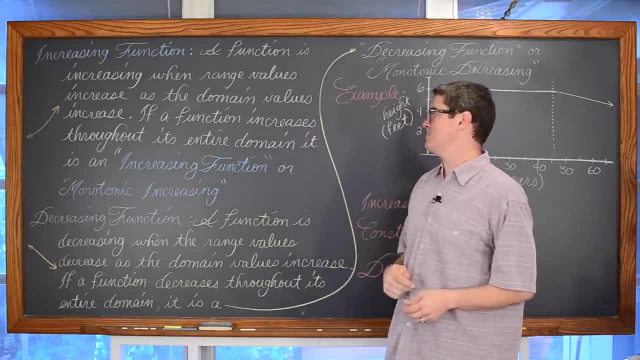 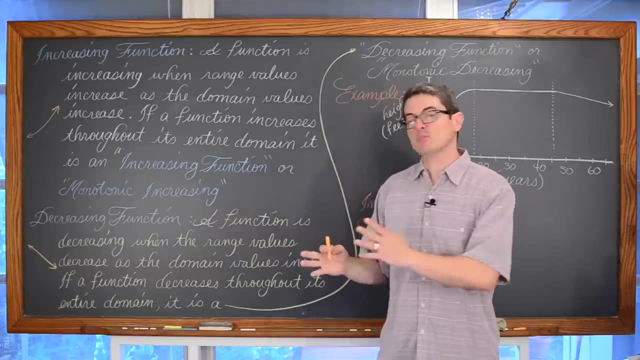 a function increases throughout its entire domain all of the x values that are included in the graph, then it is said to be an increasing function or monotonic increasing. I had some of those examples in the previous board. One maybe is like a graph, that kind of curves. 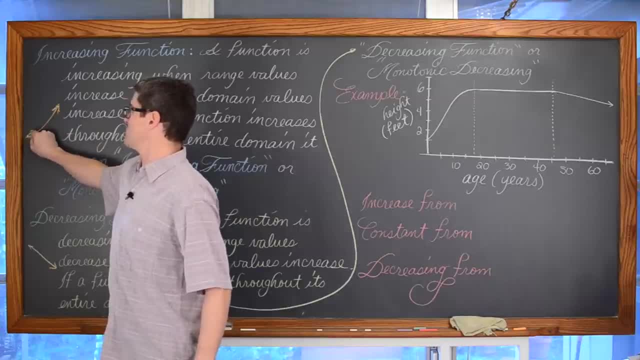 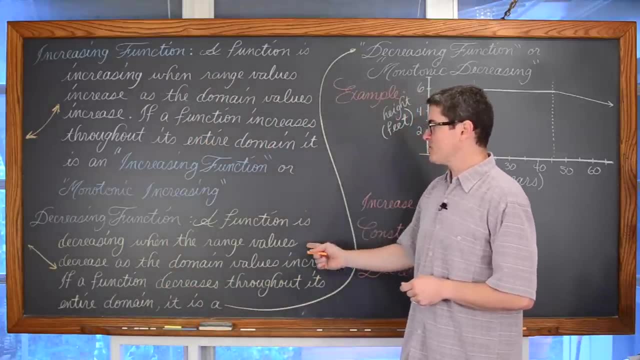 up and keeps going up and up and up and up, more as you go to the right. Those are generally going to be exponential growth functions. A decreasing function is a function that is, a function is decreasing when the range values, the y values, decrease, get smaller as the 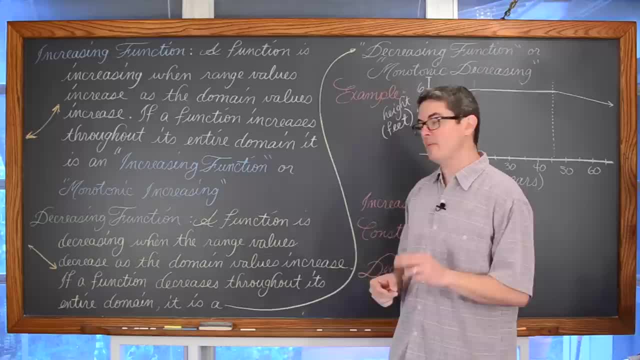 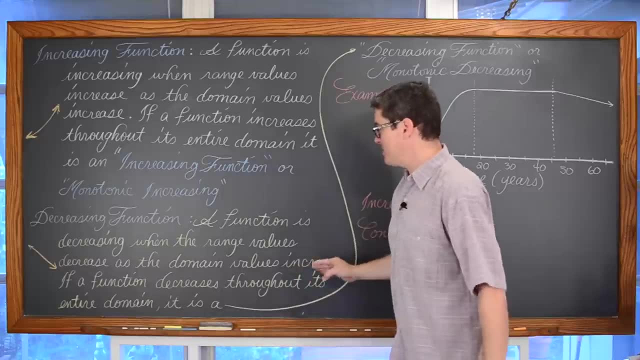 domain values increase. If a function decreases throughout its entire domain, in other words, as you look at the entire graph and you include all of the x values, if it is decreasing throughout that entire domain, it is a decreasing function, or again said to be monotonic decreasing. if 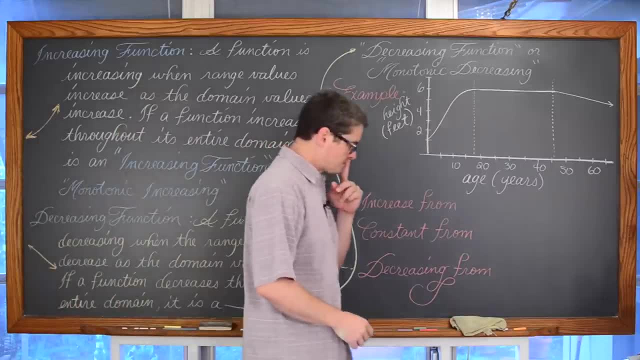 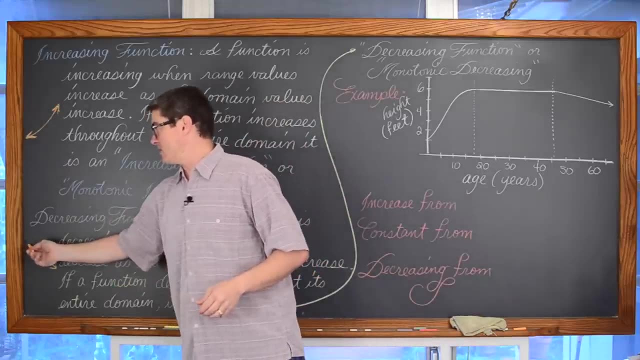 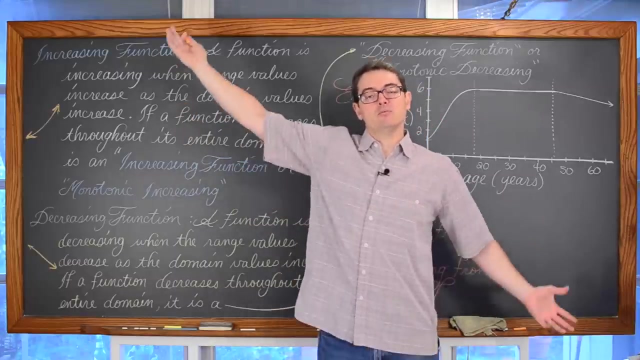 your textbook uses that phrase. Now, when you draw functions like parabolas or zons or this little curvy thing I have done going up to the right, or this line going down to the right, we have to put arrows on both sides if that graph continues in both directions. 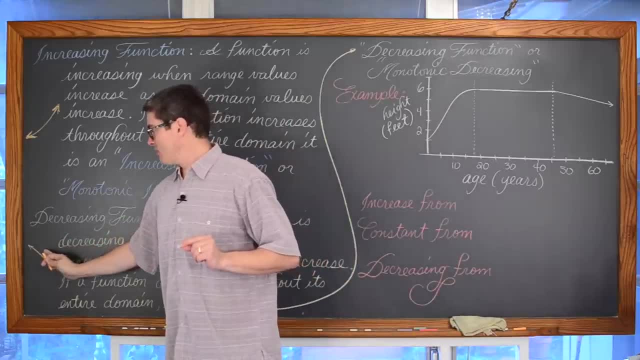 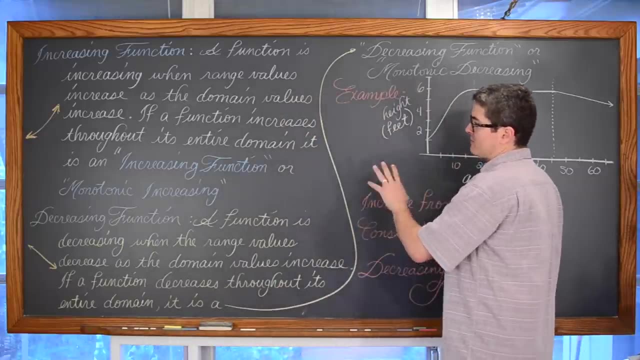 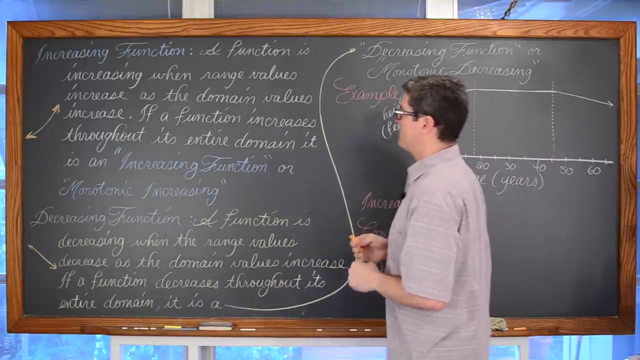 forever. But again, we don't read graphs from right to left as we are identifying intervals where the function is increasing or decreasing. Now these definitions are for an increasing function and a decreasing function. Part of that definition is it is increasing or decreasing. 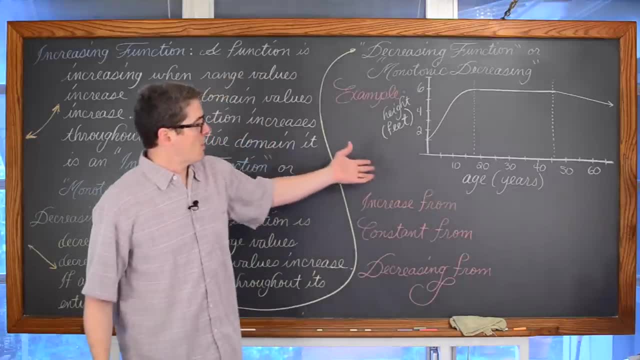 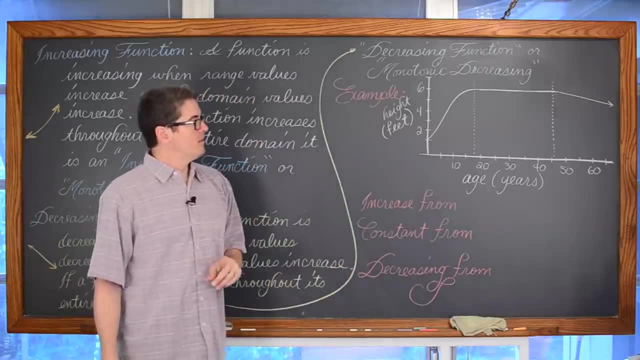 the entire domain. My example here is a graph. actually it would pass the function test. It is a function. Every vertical line you draw is going to only have one y value. But it is not an increasing or decreasing function. It is simply a function. but there are portions. 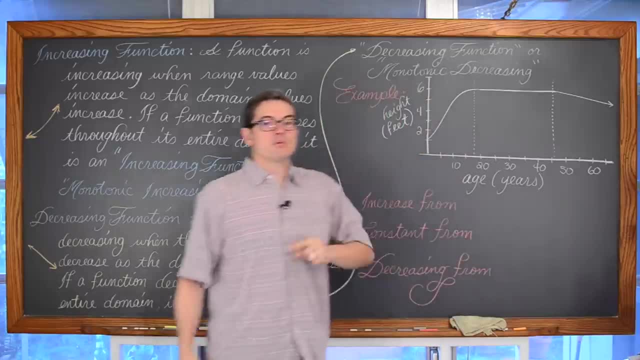 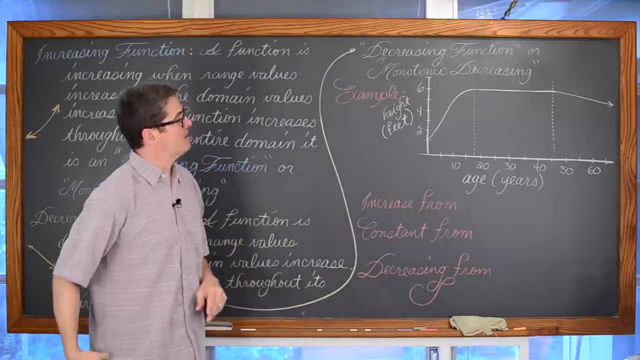 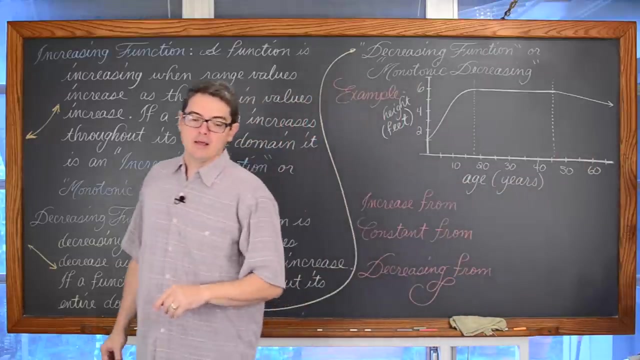 of. there are intervals along this domain where the graph is rising to the right, increasing horizontal constant and decreasing a little bit. It is tracking a person's age from the time they are born through the time they are 65 and beyond. We understand how we, as humans, 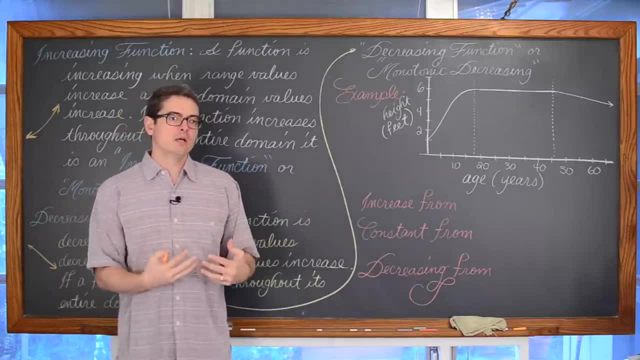 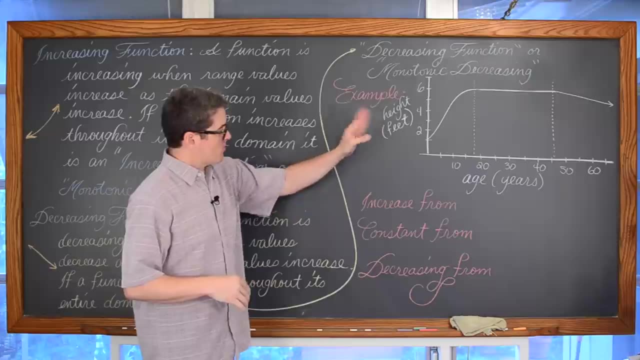 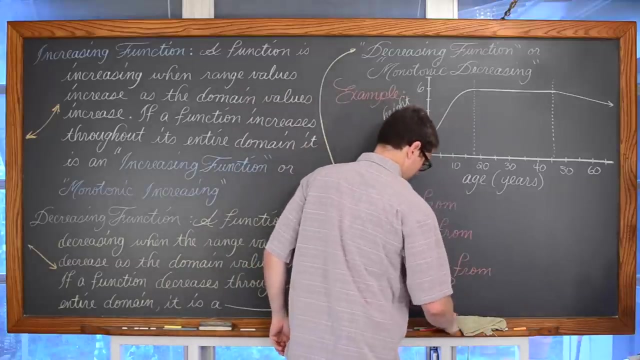 are right. We grow, we stay the same height and then eventually, as we grow older, the cartilages between our bones and everything, especially in our back, start to wear and we actually shrink a little bit. So this graph is increasing from zero to well, let's say, 18.. Or you could. 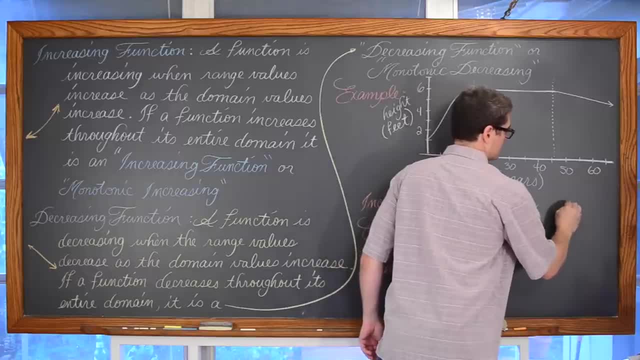 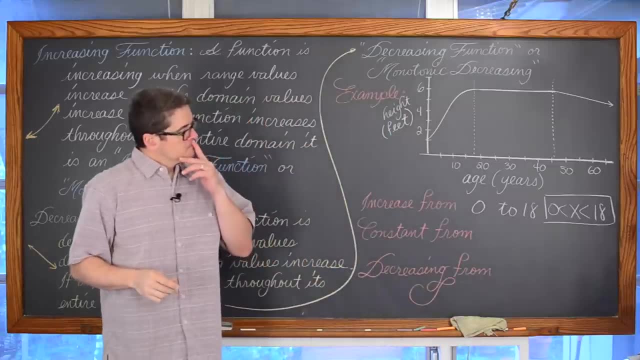 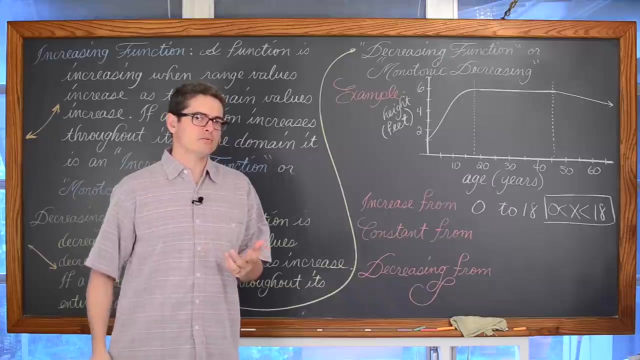 say that it is increasing from the interval of x is greater than zero and less than 18.. There is another way of writing that, using interval notation, and you would see that interval notation maybe if you were like in my precalculus class, But I wouldn't use it. 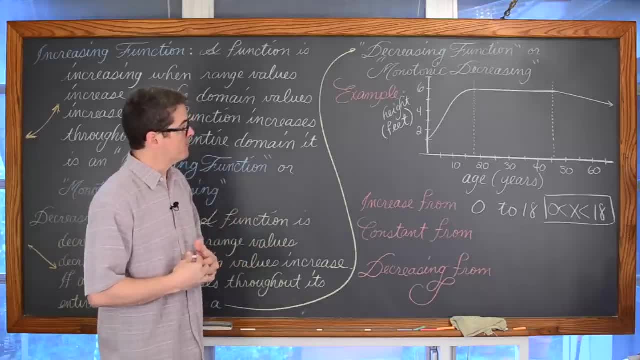 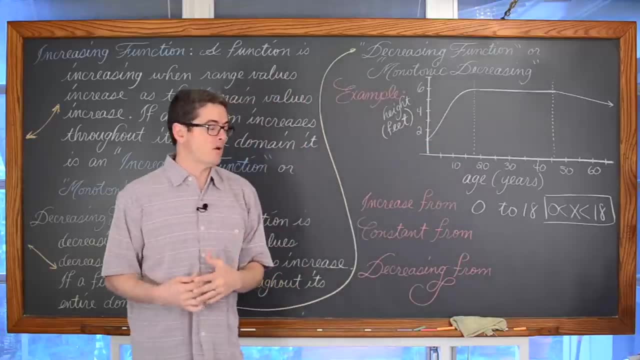 for algebra, At least it is not in the algebra textbook I am teaching from. Then we have a portion of this graph where the x's are changing but the y's are staying the same. Basically it is a horizontal portion of the graph and that is constant from x is greater. 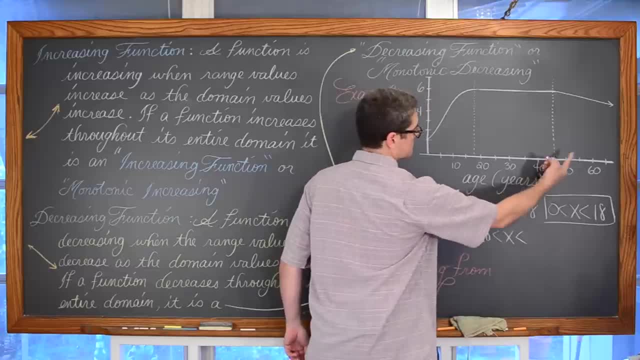 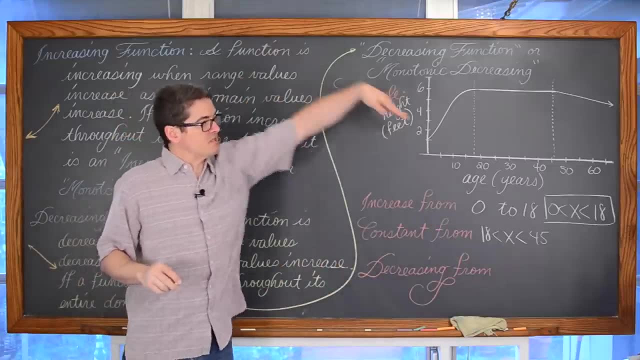 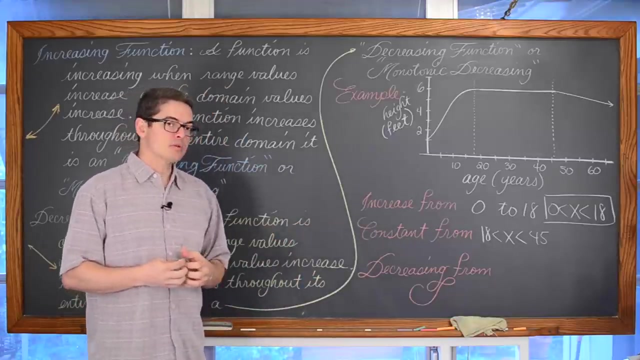 than 18, and let's just say it is less than 45.. Then, from there- and I am exaggerating to make sure that you can see that I have drawn a portion of this graph where it is falling to the right and therefore it is going to. 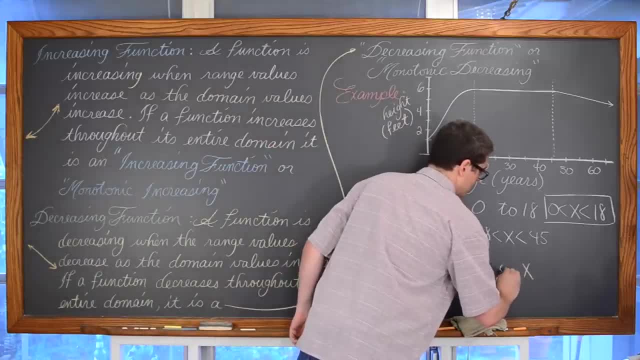 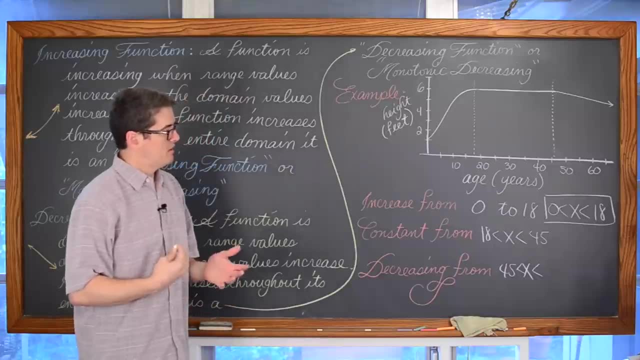 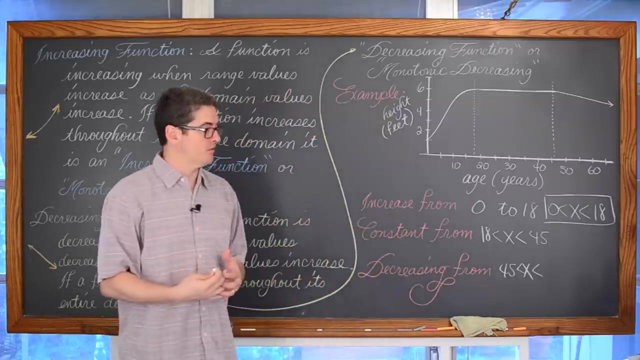 be decreasing from the x values of 45 to however long. it is a reasonable life span for a person, But I don't want to say that it goes to 100 because people have lived beyond 100. Maybe eventually people live long- 110, 120, 130 years, I don't know. 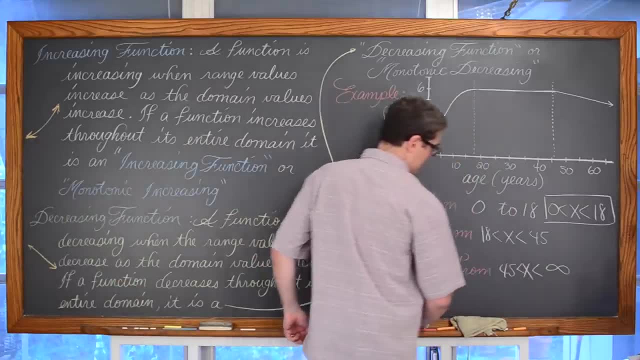 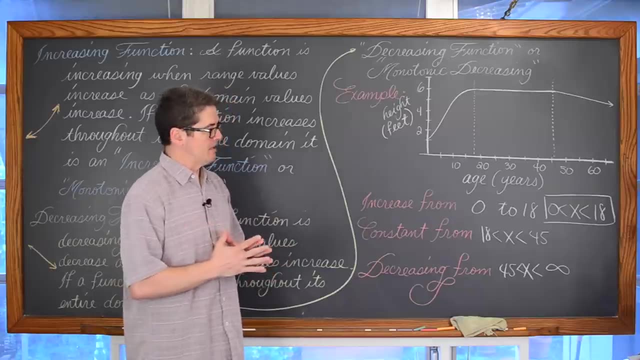 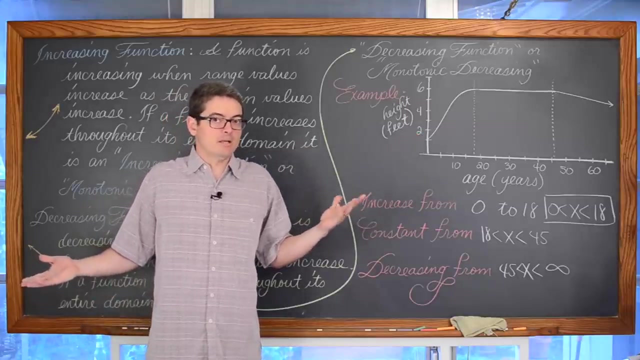 I am going to go ahead and say that it is going to decrease from 45 on to infinity, even though that is not really a real thing, realistic domain for an idea of tracking somebody's age. It also wouldn't make any sense to have any negative ages, because you are going to be negative ten years old, Ok, so anyway. 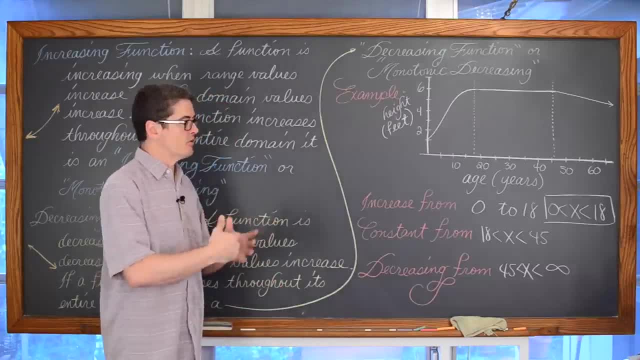 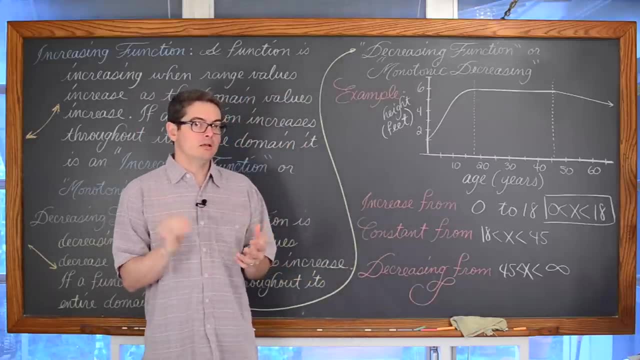 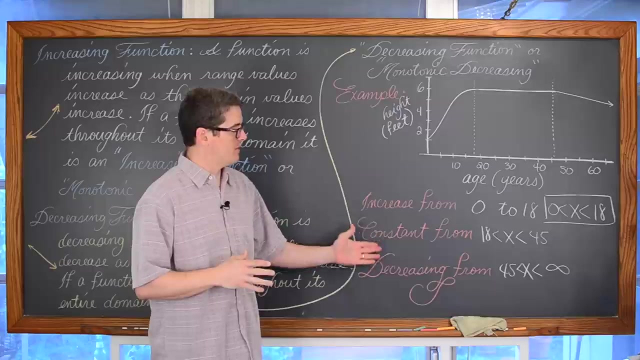 this is actually reinforcing some vocabulary that I have done in a previous lesson as well in our algebra class. Oh, also, before we move on to identifying domain and range, well, defining it and identifying it in a graph, please note that I am talking about the intervals along. 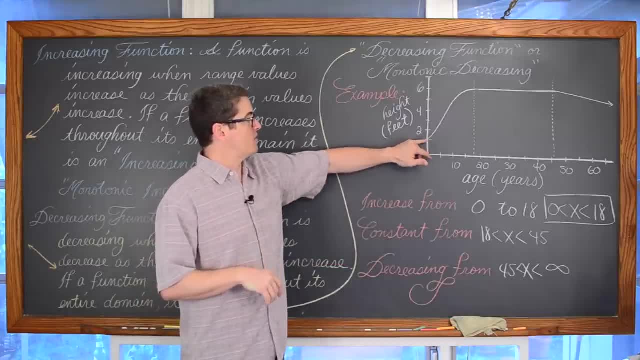 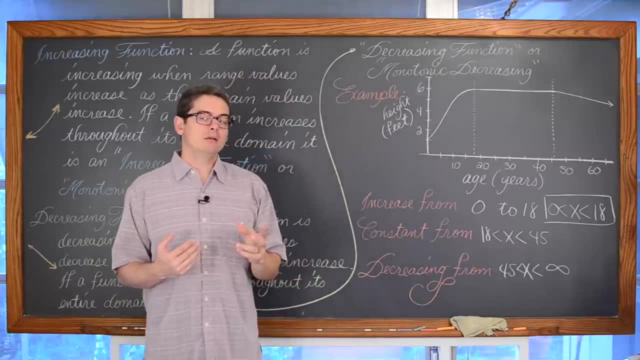 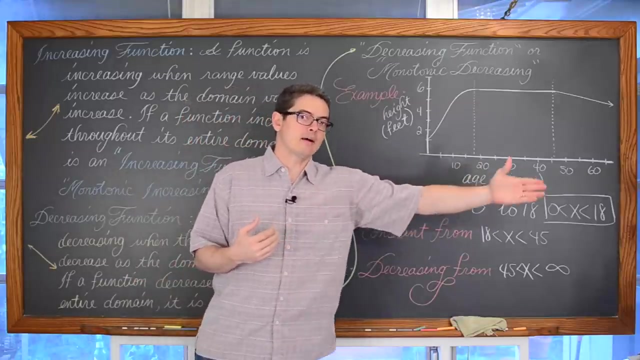 the x axis. A lot of students would want to say that this graph increases from one to six. Yes, the y value goes from one foot to six foot, but when we identify intervals where a graph is increasing or decreasing, we are talking about the interval along the x values. 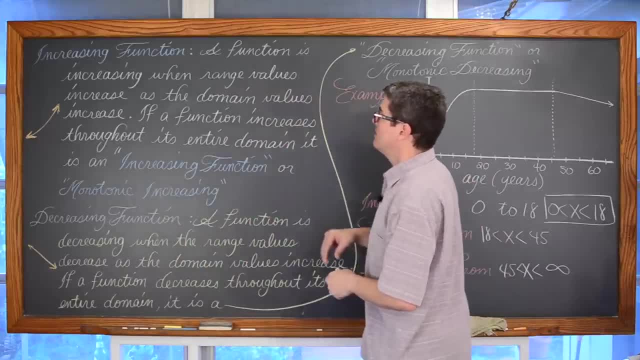 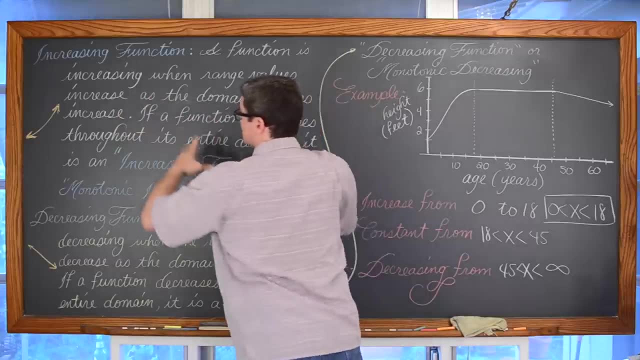 because you know and you can see that as part of the definition is a function is increasing when the range, the y values, are increasing as the domain values. It is about those intervals along the x axis where you want to identify the functions going up to the right horizontal. 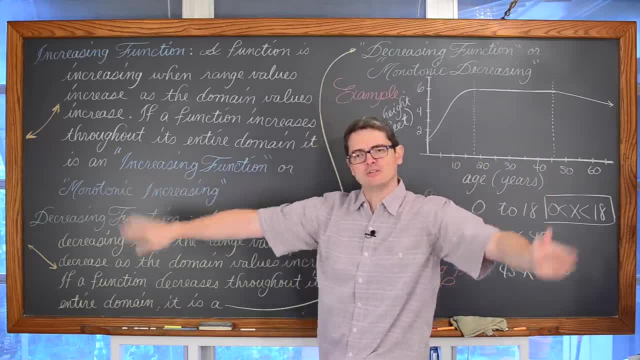 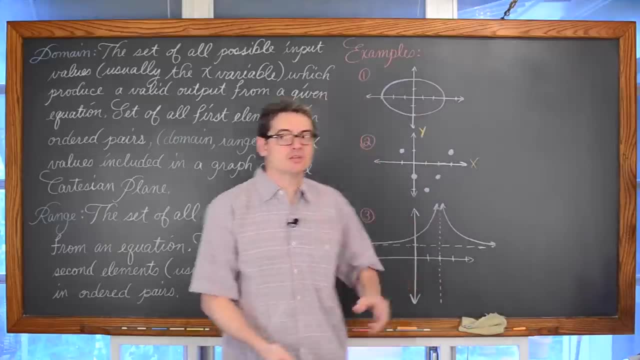 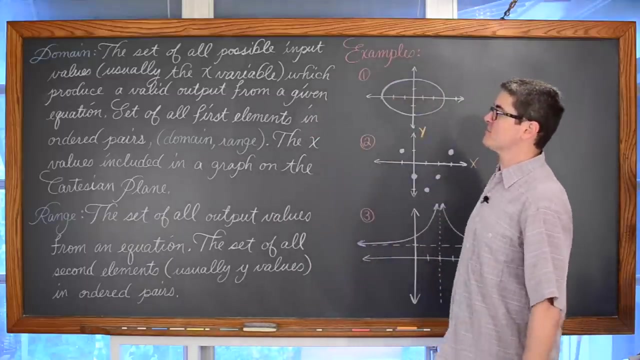 or down to the right. Let's move on to domain and range: BAM, BAM. So you want to identify what domain and range is When you look at the graph of an equation? well then, you are going to have to know the definitions And the set of all possible input values. you 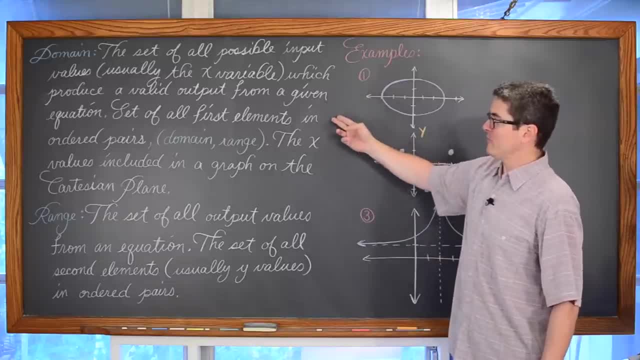 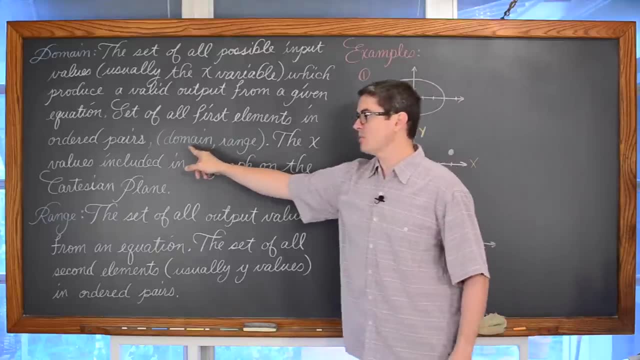 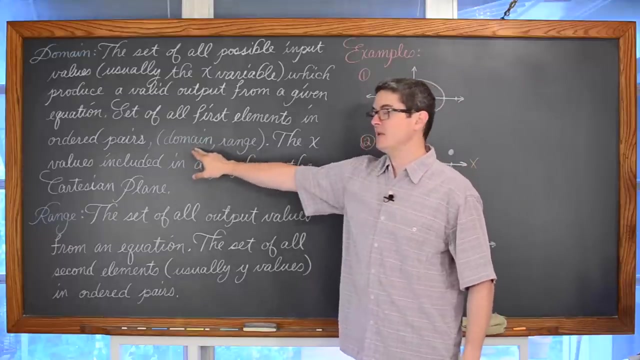 use usually the x variable, which produce a valid output from a given equation. Or you can say it is the set of all first elements in ordered pairs And ordered pairs are the well ordered pairs are a grouping of two numbers, which is the domain and range: the left right. 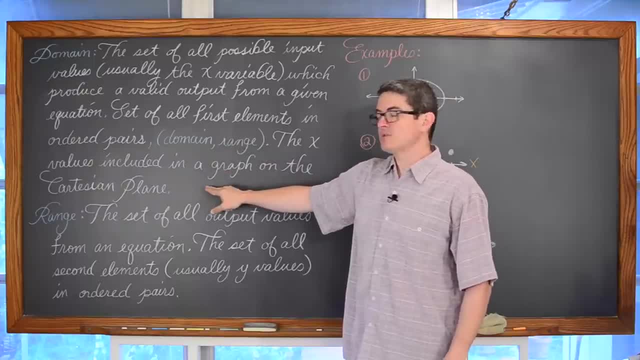 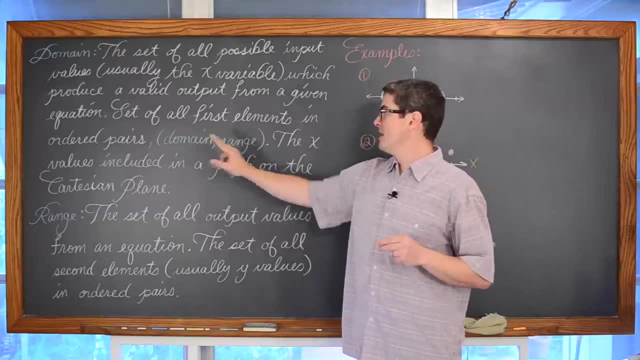 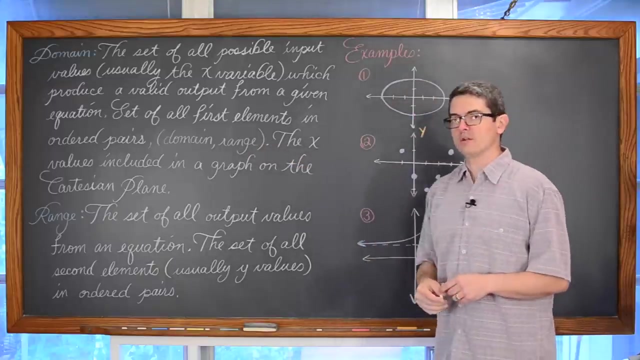 movement and the up and down movement. Or, if you are talking about your graph being on the Cartesian plane, that would be the x, the movement in terms of the x axis, and then the y values Or the movement along the y axis. The x values include in the graph on the Cartesian plane. 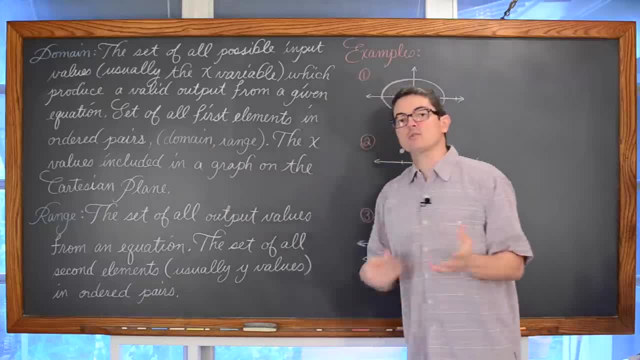 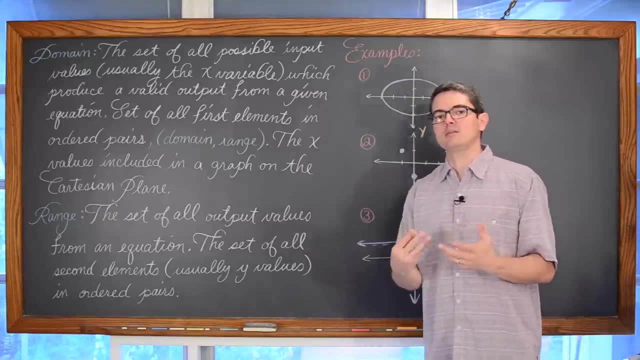 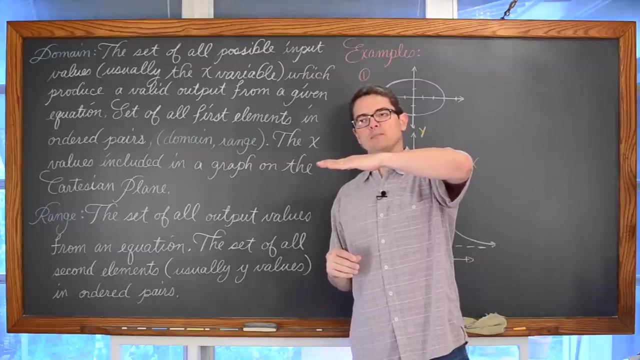 So usually it is x comma y, Unless you are looking at some kind of graph that is displaying a real life scenario where there is some real context to what the horizontal and vertical axis are, Such as maybe the age being along the horizontal axis or the x axis and your 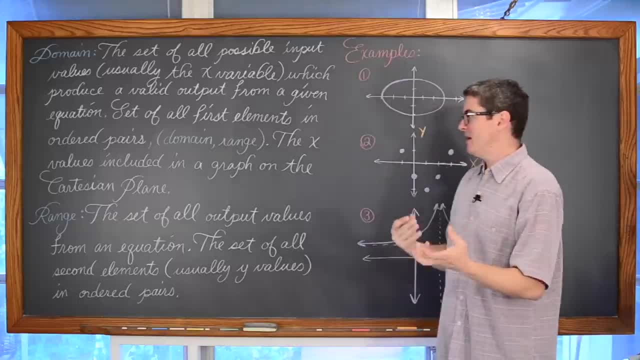 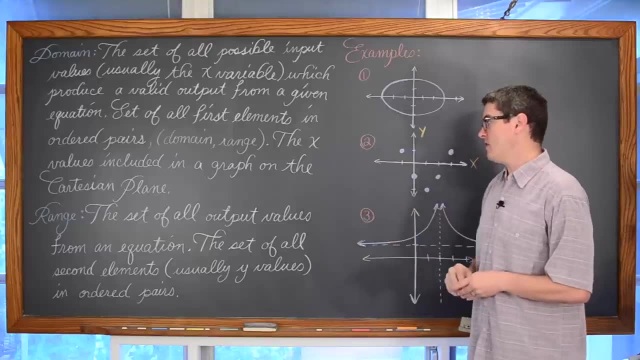 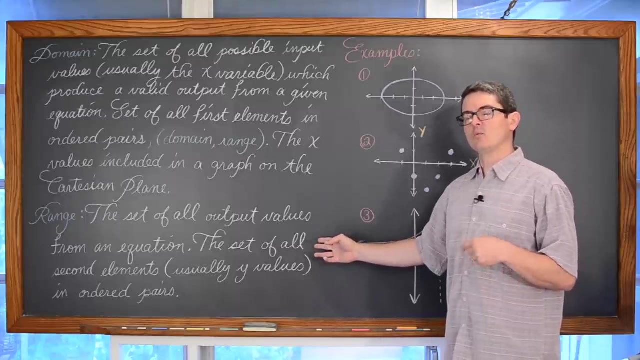 height being along the y axis. But I am saying this again because I am going to make this lesson that we are watching right now is actually an excerpt of a full length lesson. The range is the set of all output values from an equation, and it is very difficult to determine what the range is from an equation. 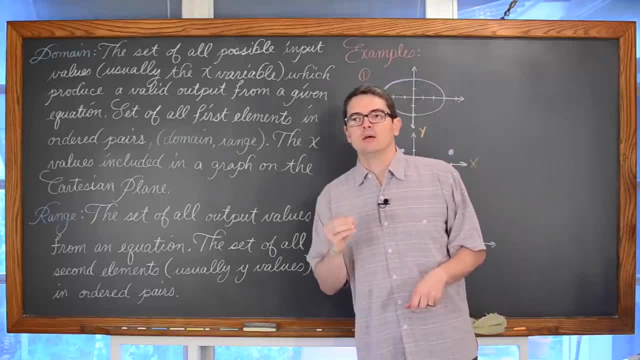 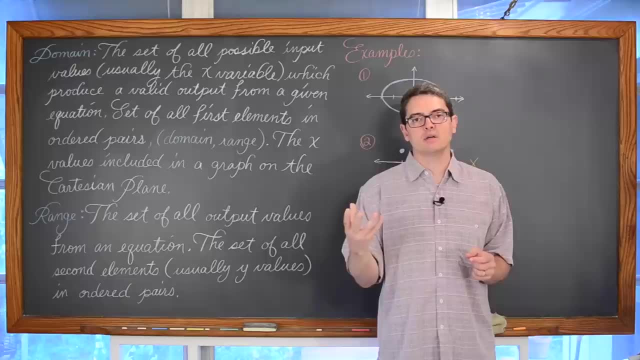 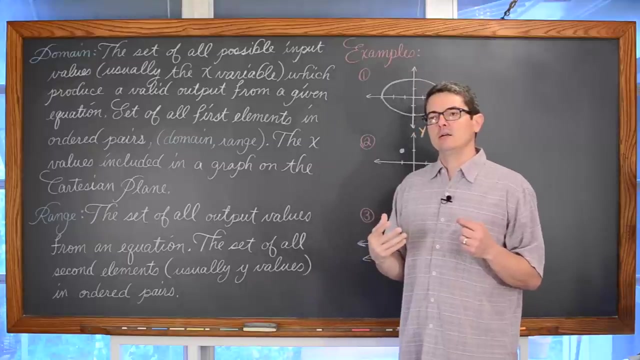 unless you are very knowledgeable. You have very strong knowledge of what all are- sort of the parent functions, if you will Like, if you know what a standard line looks like, A standard parabola, A standard absolute value, linear function, your function, maybe even square root functions and such. If you understand and you know what. 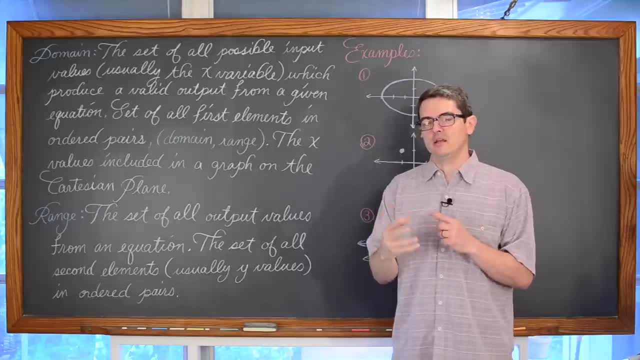 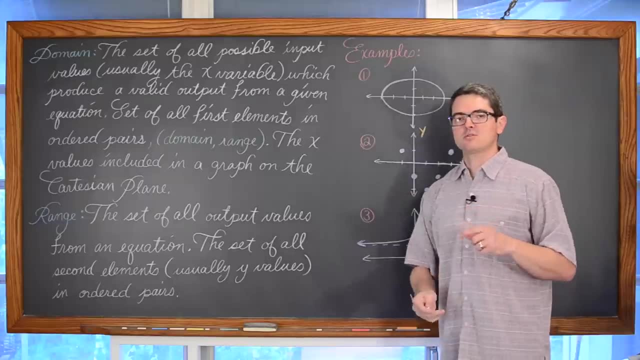 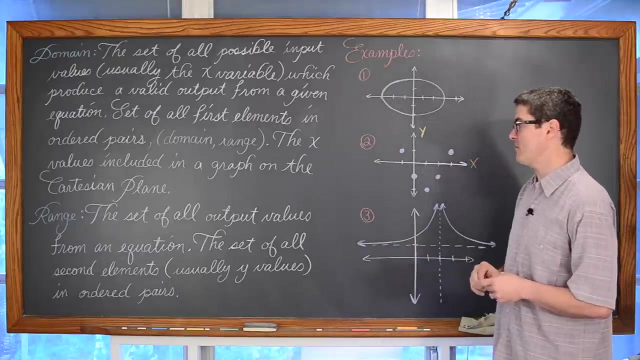 those parent functions look like, and you are very knowledgeable of translations and this lesson is for an algebra class. we haven't even gotten to that yet. I would strongly suggest you create a graph from that equation first, before you try to determine what the range is. But the set of all output values from an equation, the set of all second elements, 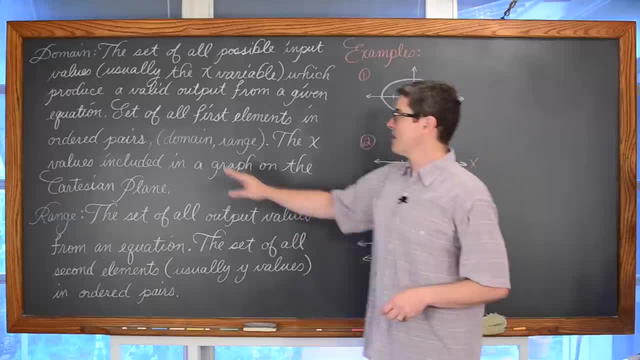 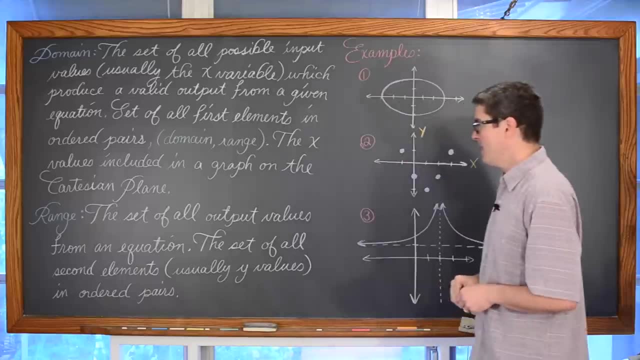 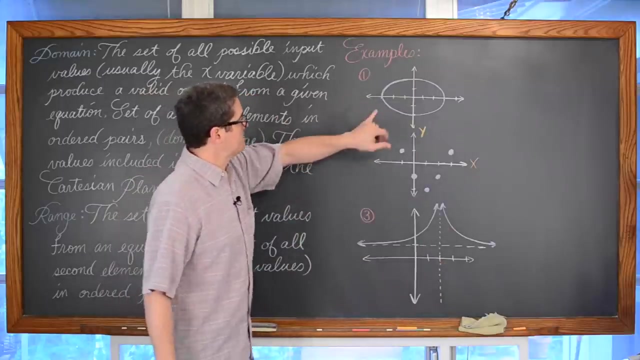 usually the y values in ordered pairs. Again, if you are talking about a domain, range, type, organization or ordered set, that is usually an x and a y value. So let's move on to our three examples. We have here an ellipse and the domain. It seems like again remembering 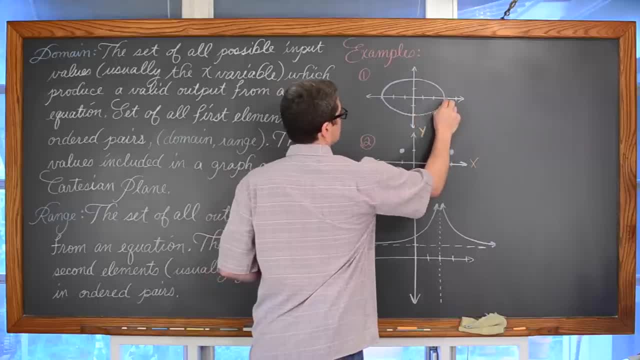 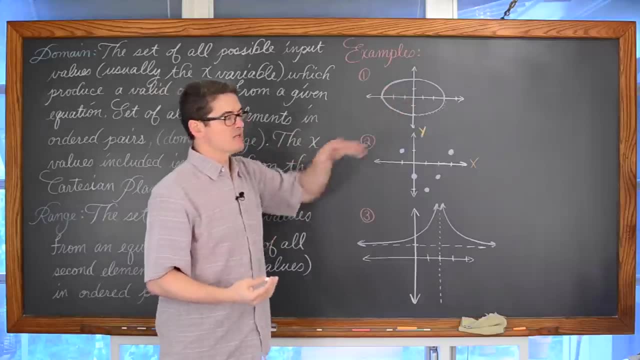 that this graph is made up of an infinite number of points, each of those individual points having, well, I guess maybe there is a couple of points with the same x values, But really each of those points having their own value of x, their own coordinate right. 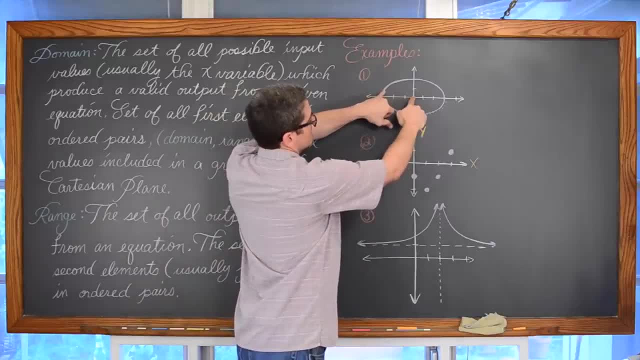 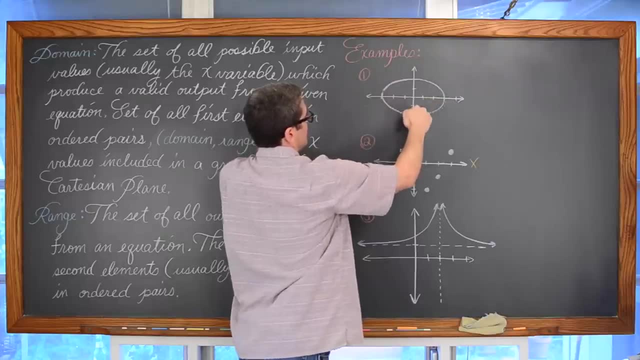 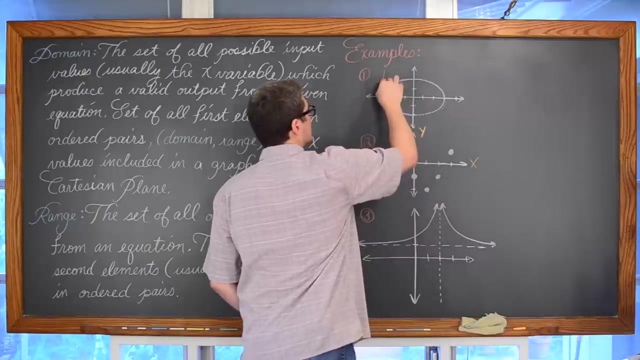 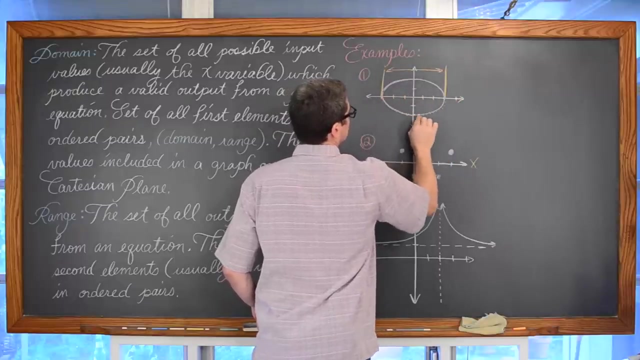 Because that point, a coordinate, describes how you get from the origin to that point. There is some kind of left-right movement, a negative x or a positive x, and some up and down movement, a negative y or positive y. So what values of x are included in all? 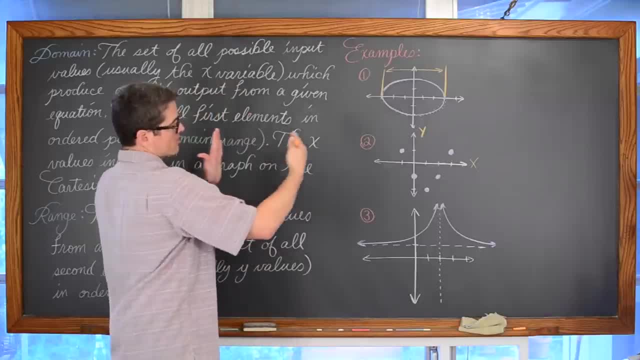 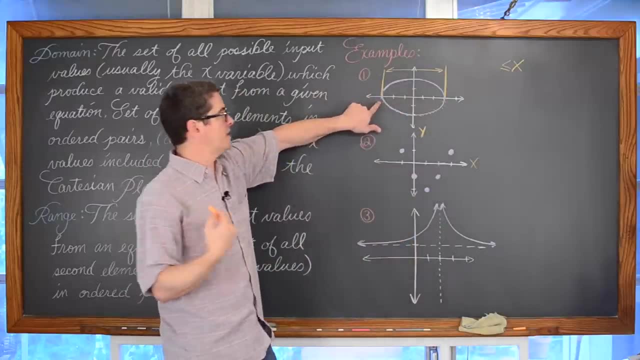 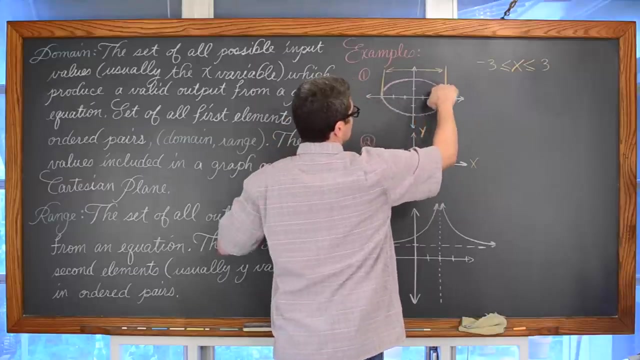 these points. Well, the domain looking at that horizontal movement is going to be x. the smallest value of x that is included looks like it goes as far to the left as negative three and then as far to the right as positive three. This is a smooth and actually being 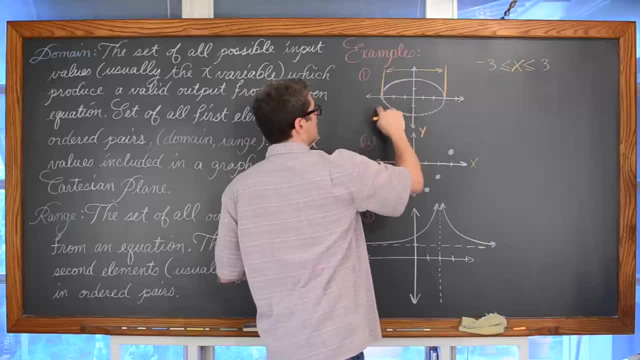 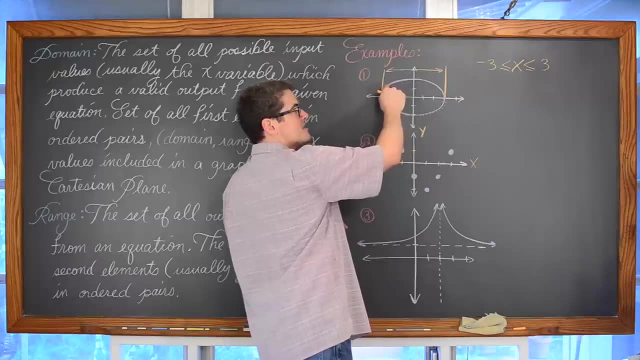 smooth isn't really important. this is a continuous graph. So every single like negative three. negative two point nine. negative two point nine. negative two point seven. negative two point six, nine, nine, nine, nine, five, three, eight, two, one, like any x that you can say. 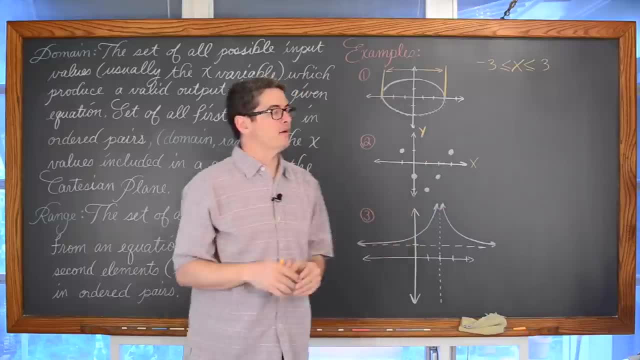 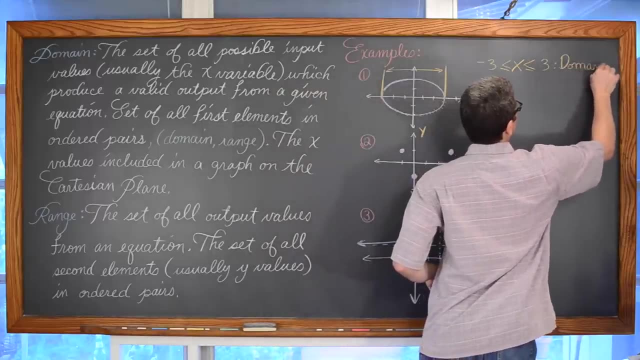 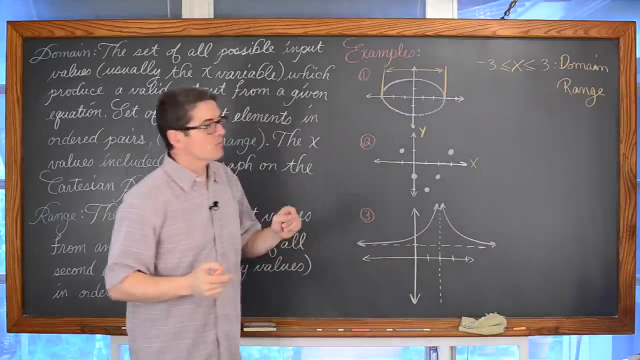 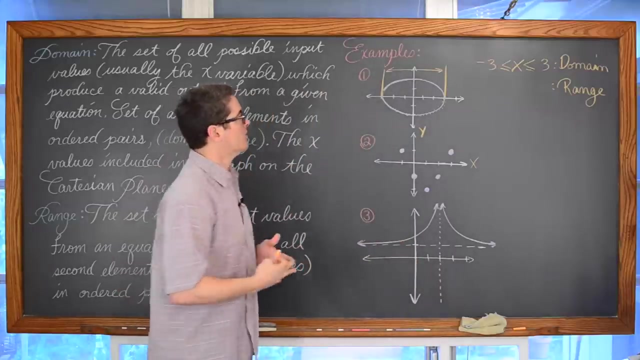 that is between negative three and positive three, including those values, would be part of the domain In the range. my- i kind of looks like an n there. my range then would be all of the output Output values, if I were looking at an equation, but graphically we are looking at again this. 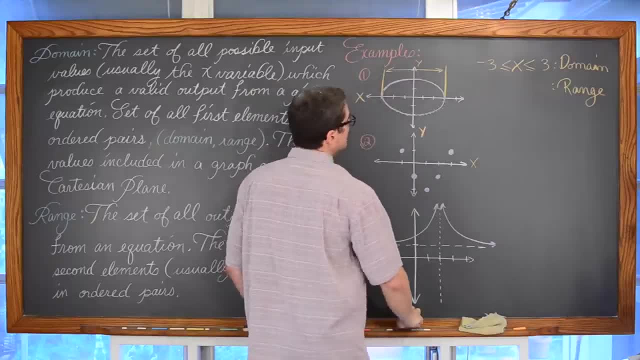 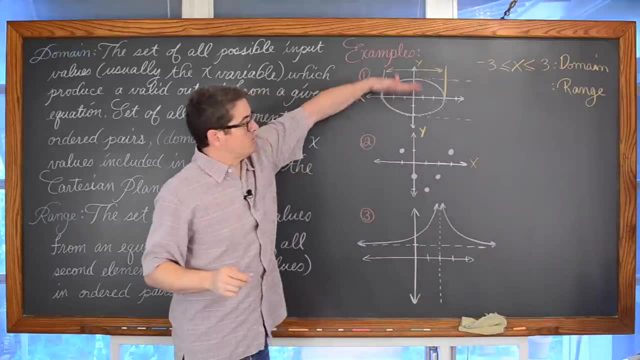 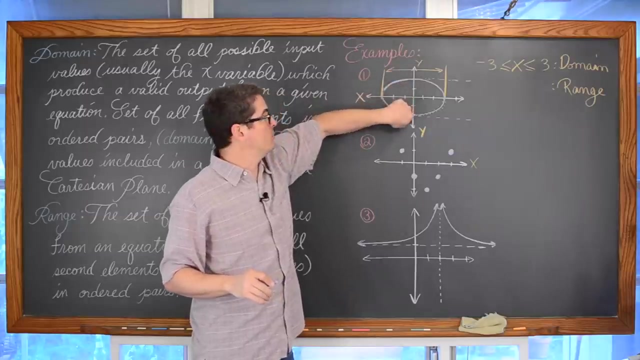 is the x axis and the y axis. the range are all the y values that are included in that graph. Now again, that graph is continuous, so it seems like it goes as far down as negative two and as far up as positive two, and every single y value is included between that. 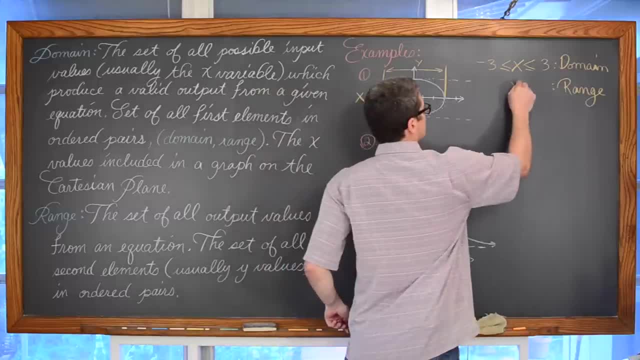 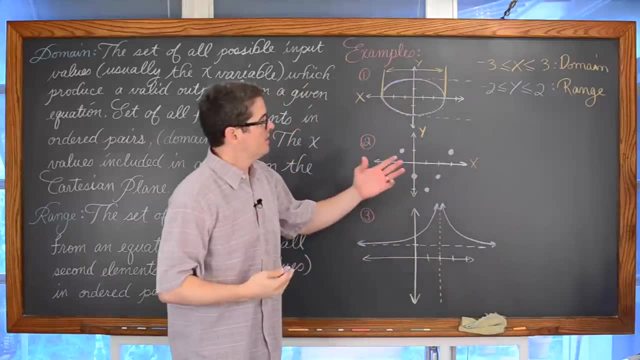 negative two and positive two. So the range is going to be: y is going to be greater than or equal to negative two and less than or equal to positive two. I am writing these in inequality notation in a pre-calculus book. you might see this in interval notation. 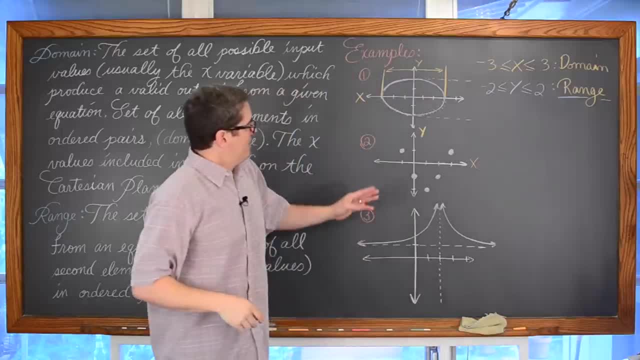 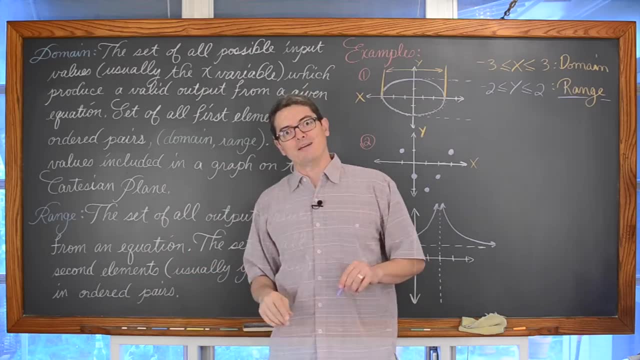 so I am not liking the fact that that color doesn't match now In number two. actually, my air conditioner came on. I know that kind of bothers the video sometimes a little bit, so let me shut that off and come right back. Ok, now that is better. Our system is now. 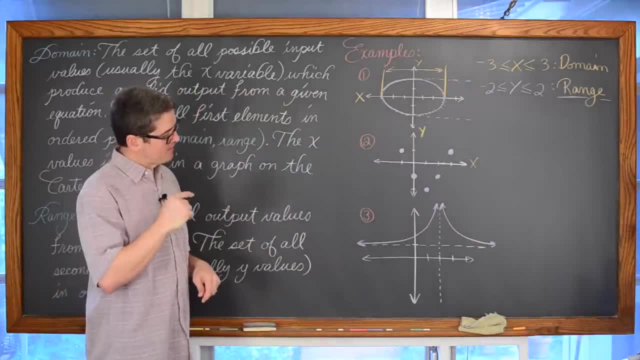 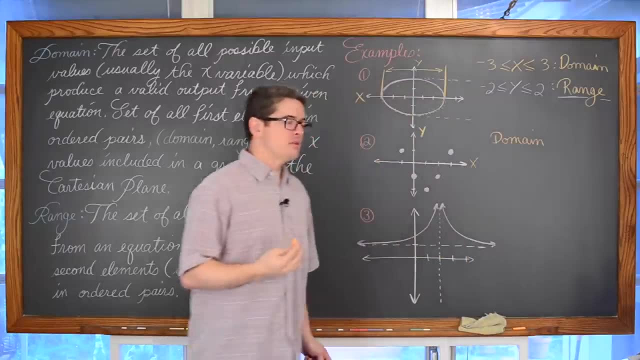 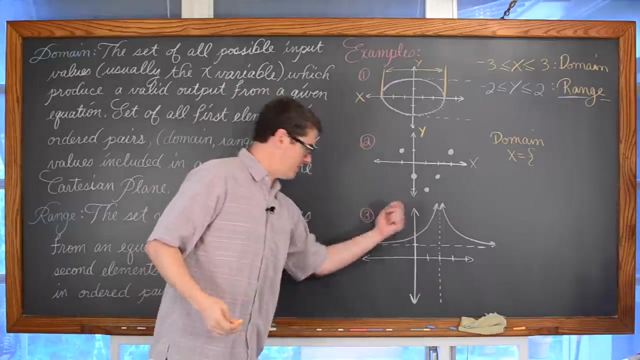 working. Our second graph is a collection of five points and if I want to list the domain here, then I really just need to write a list of values for x, Because this is a discrete graph. I can see ah, chalk down that there is only five points, So we have. 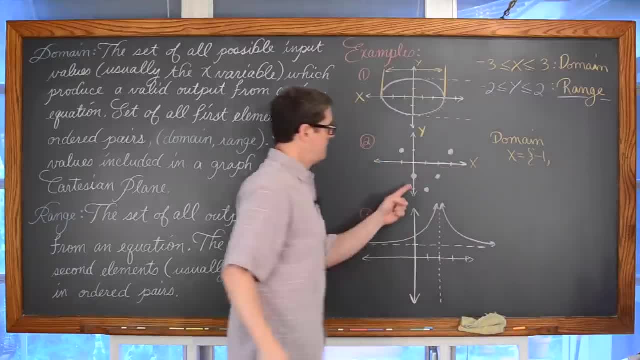 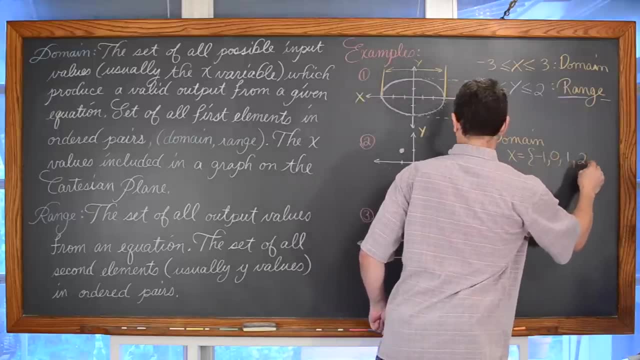 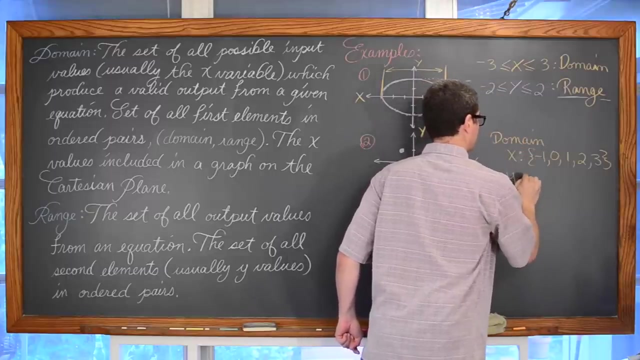 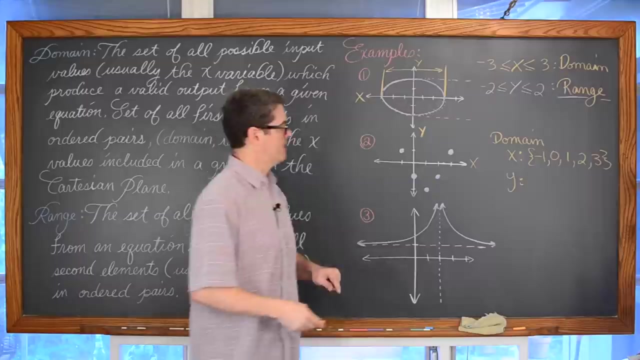 an x value of negative one, an x value of zero one, two and three, And then we have a y value of negative one And my y values are. now I don't need to repeat the same y value over and over and over again. I can just see that this point has a y value of. 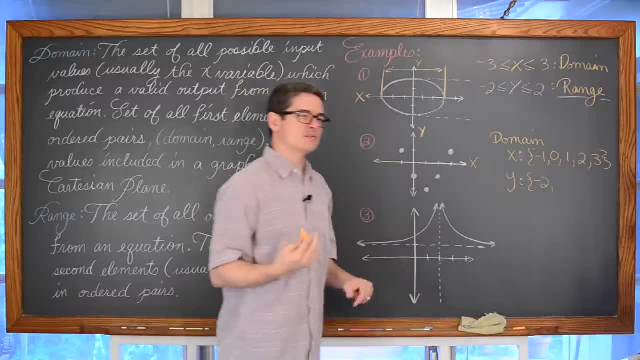 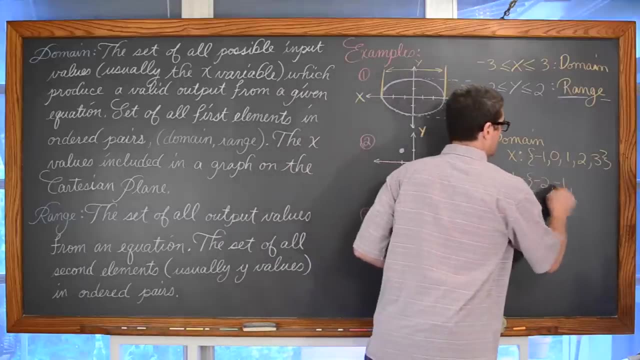 negative two, And it is a good practice to write these from low to high. Then we have a y value of from the origin. we have to go down one, so the y value is negative one. And finally we have a y value of positive one. Ok, 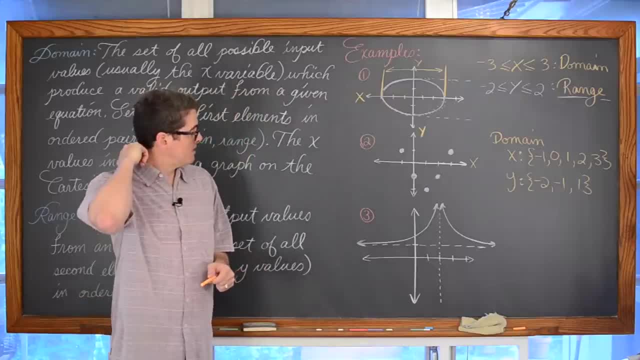 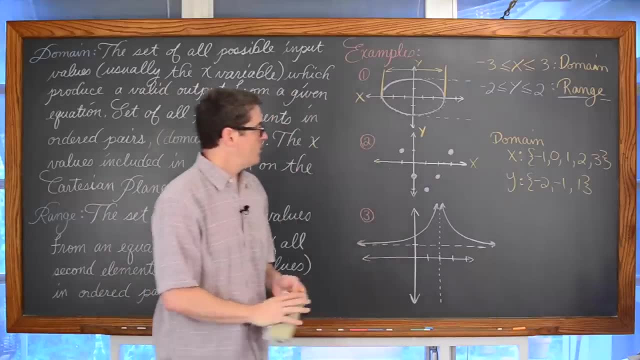 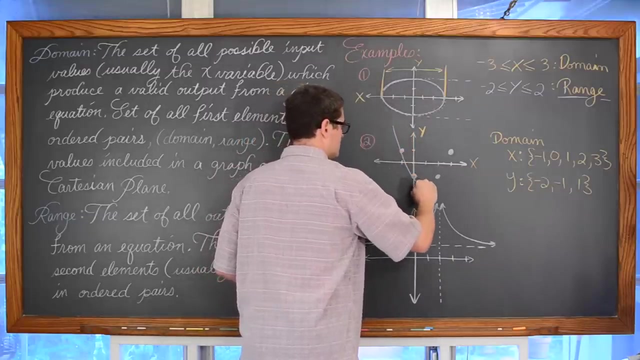 And that is how you list domain and range for a discrete graph. Excuse me, you have to just list all the individual x and y values. Now, if I were to come back here and change this example to one that kind of seems to go on forever and is continuous and not focus, 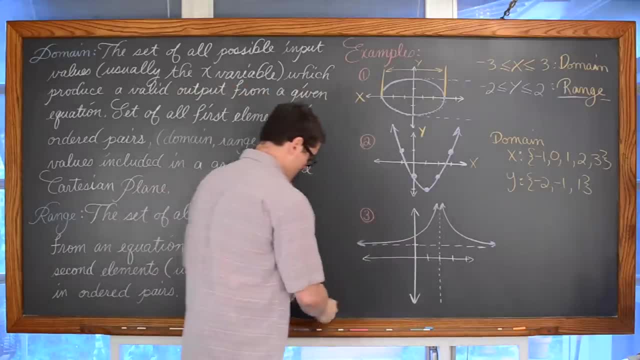 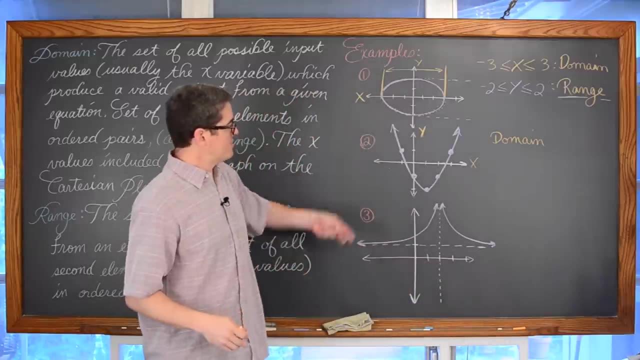 on those five discrete points. well, now my domain is going to be- And I really am intending on writing these in different colors- Now my domain. well, this graph goes. it is going up, but it is spreading to the left and spreading to the right forever. 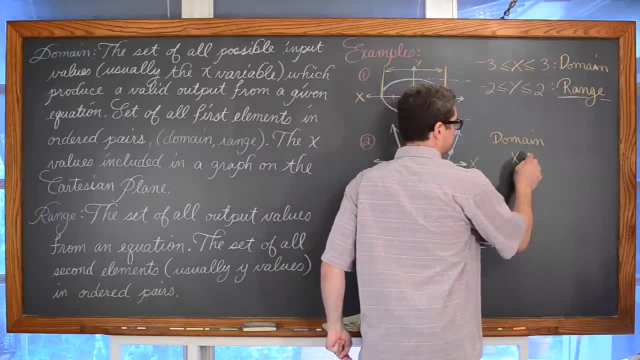 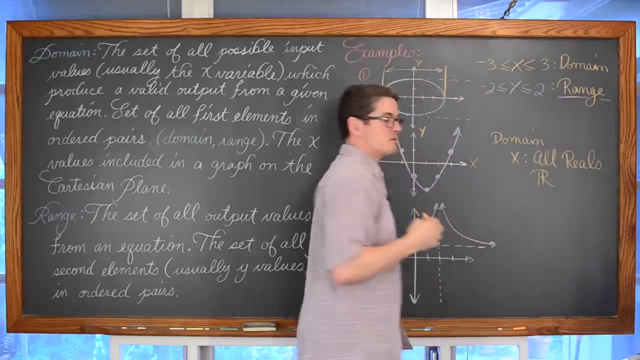 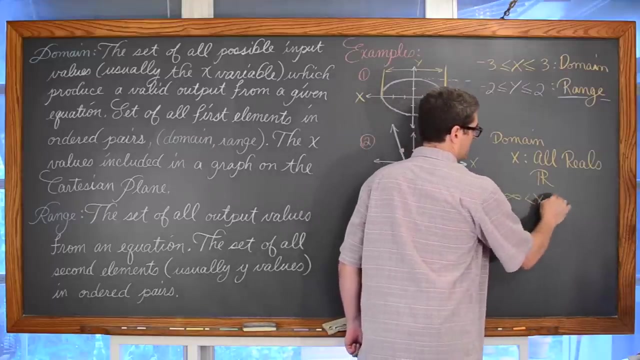 So the domain is all real numbers, And so you can say that x is either all reals- You might have a textbook that kind of uses a double r for all reals- Or you could say that x is less than- or excuse me- greater than negative infinity and less than positive infinity. 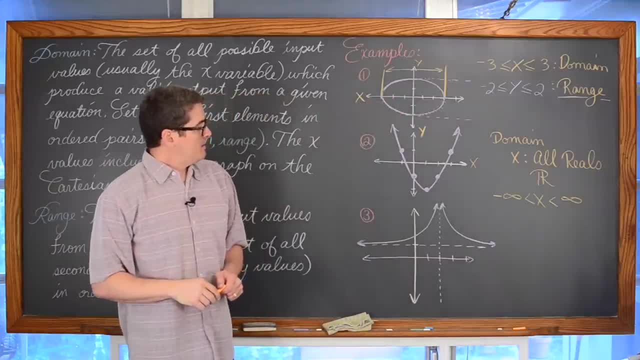 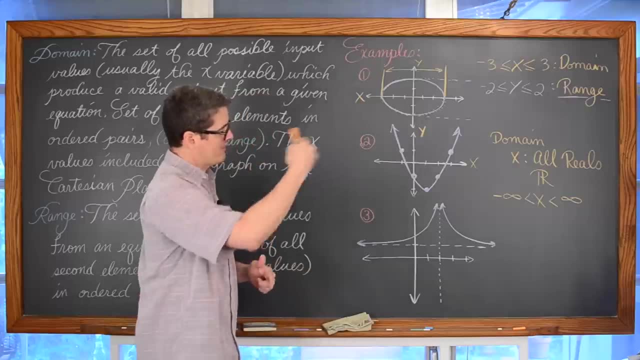 Because, again, it goes on forever And you can't say equal to infinity, because that is sort of like an infinite concept. It goes on forever and ever and ever and ever. And the range? well, the smallest. again. all these points are in here. now There is an infinite. 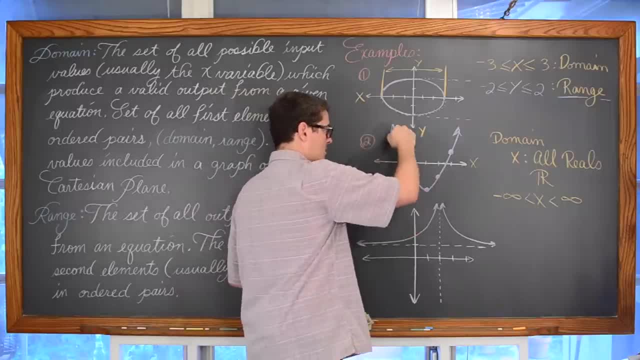 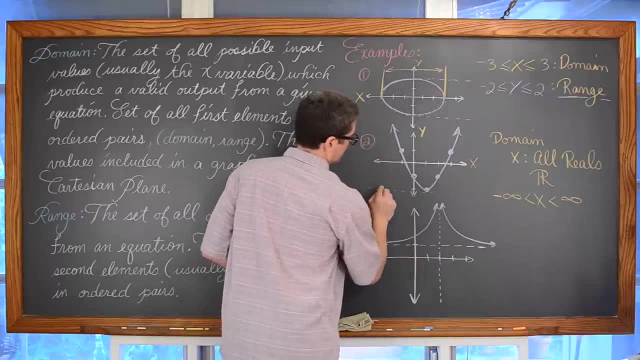 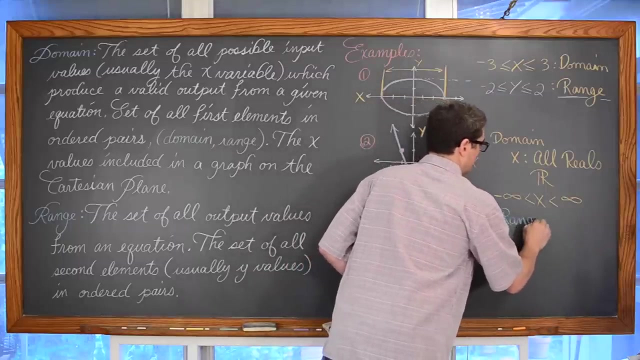 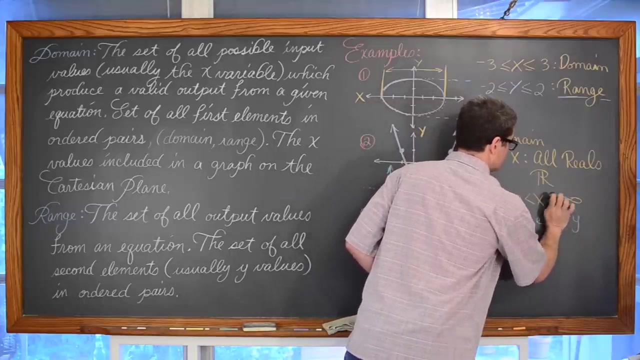 number of points And the smallest y value, or the point that is the farthest down on this graph, and then from here the graph kind of just goes up forever. So the smallest y value is negative two. So the range is going to be: y is greater than or equal to negative. 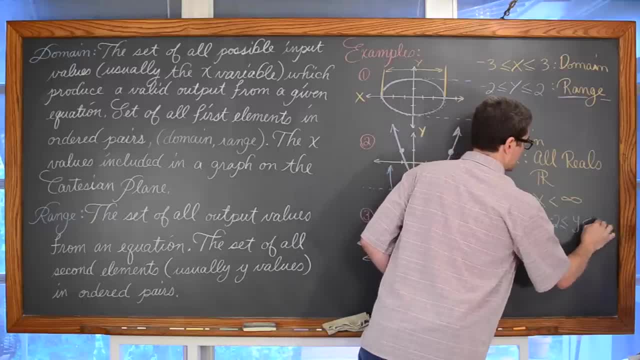 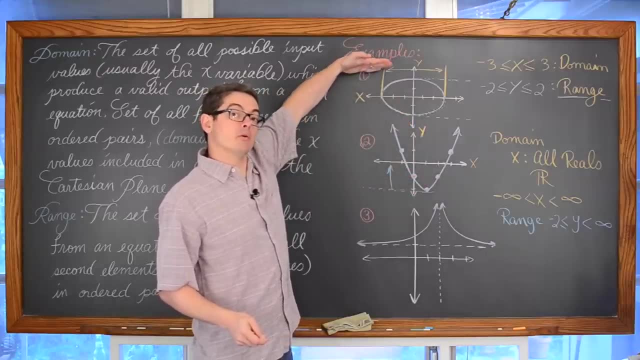 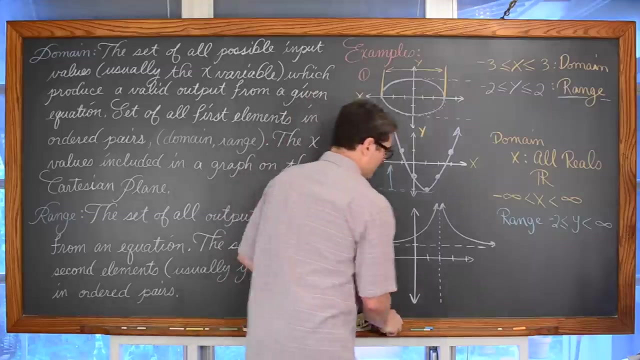 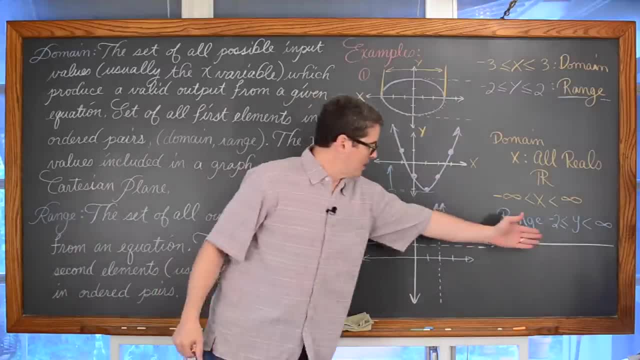 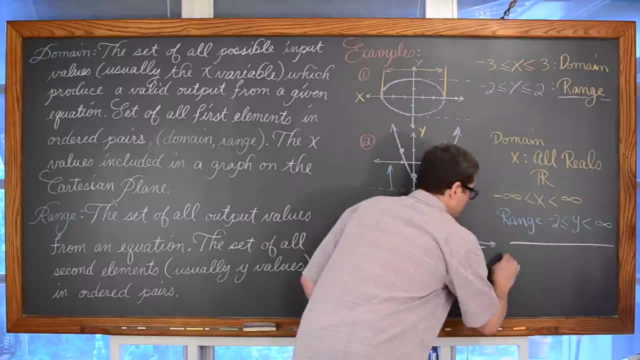 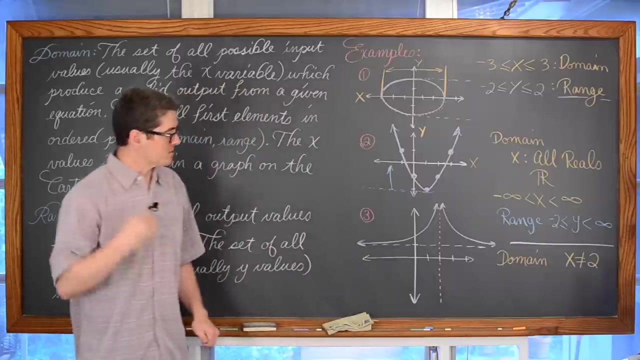 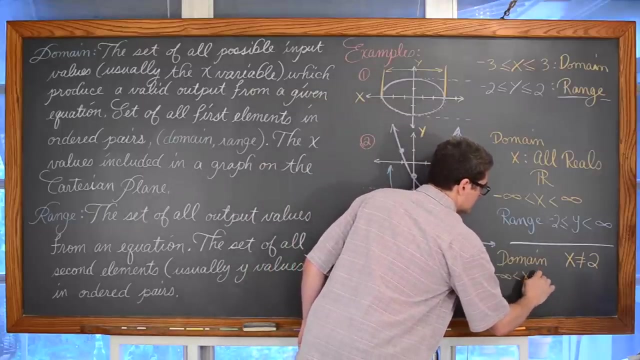 going to have a graph that seems to go left and right forever. It seems like there are no breaks in this graph except at two. So our domain is: x cannot be equal to negative two. Or you may write that x is greater than negative infinity and less than two And x. 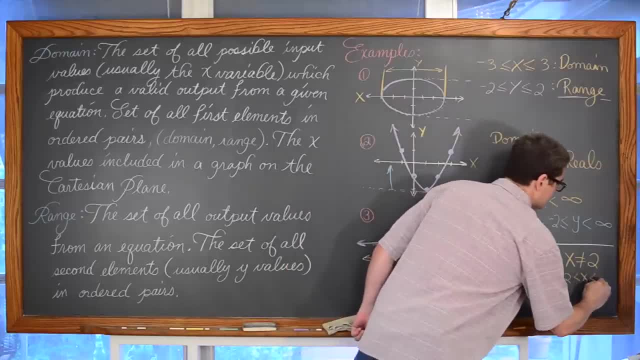 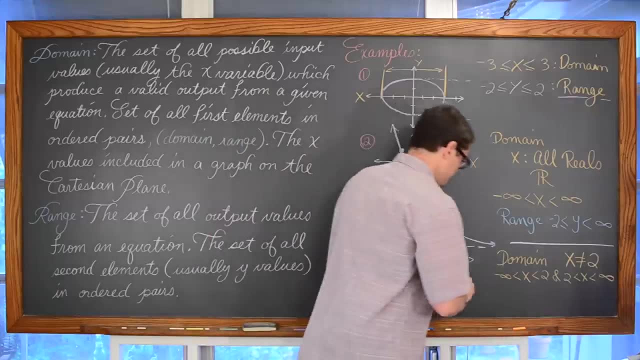 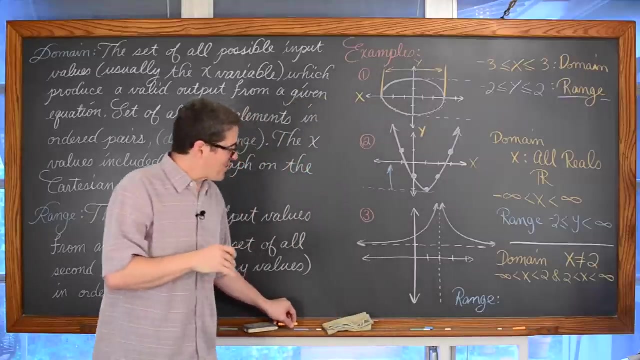 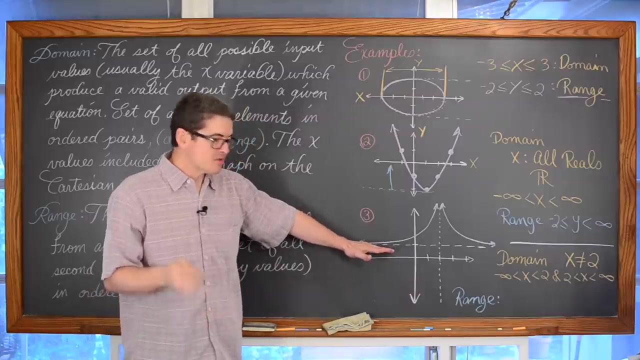 is greater than two And less than positive infinity, if your teacher wants you to write it that way. And now the range values Get down with it. The range values are all the y values that are included in the graph. Well, the graph is nowhere below. nowhere do you see a purple line below this. 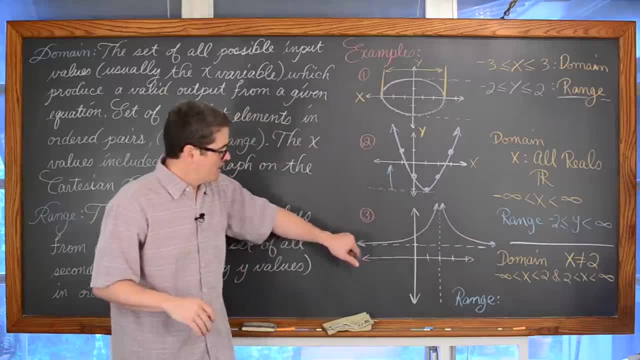 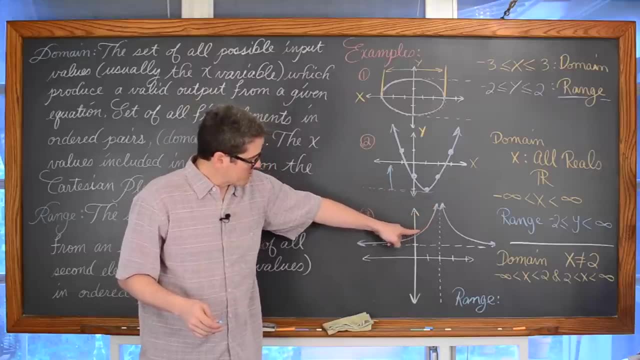 horizontal asymptote. this horizontal line that is at y is equal to one. So the graph, These y values, are going to get smaller and smaller and smaller. maybe here it's at 2, maybe it's at 1.5, 1.1,, 1.0000001.. 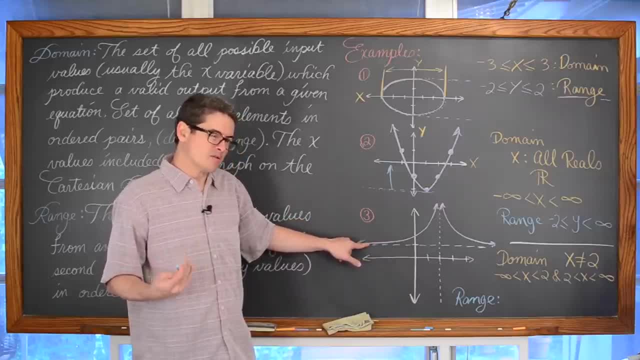 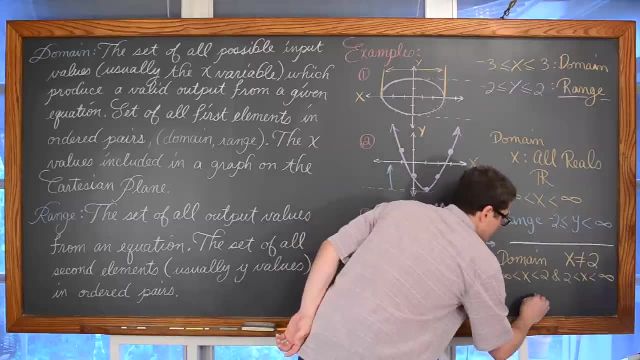 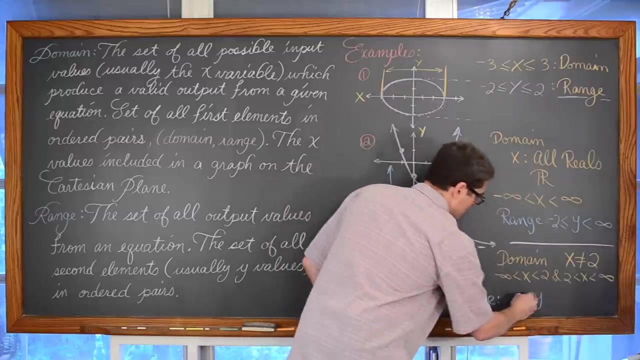 Now I'm on the left side, right, where the x's are negative but the y's still positive And it's going to get closer and closer to that y value of 1 but never really become 1.. So we're going to say that the range is y is less than 1, or, excuse me, not less than 1,, greater than 1 and less. 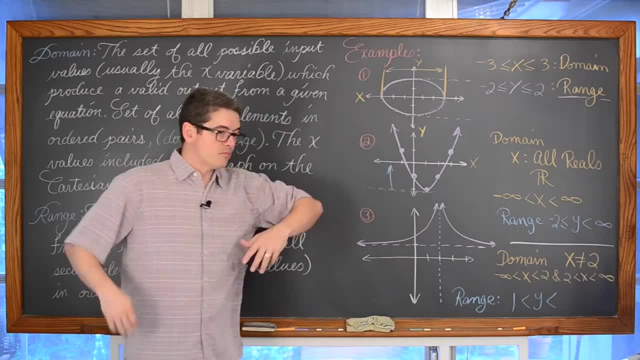 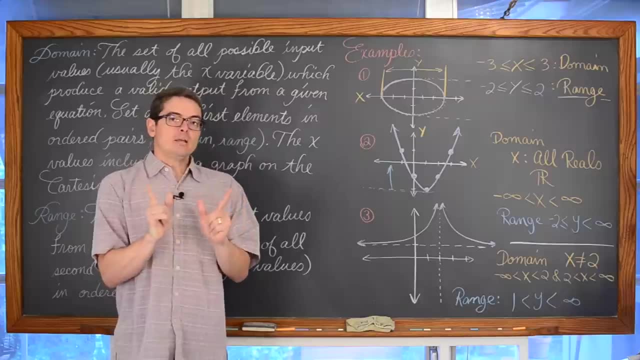 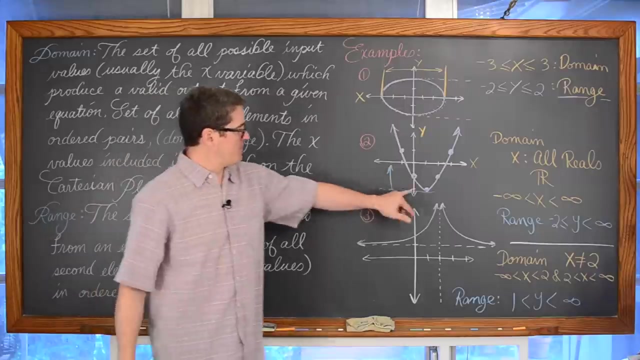 Now this goes up forever, right? so y is never going to stop growing. So y is less than infinity. Okay, in an upcoming algebra lesson we're going to be talking about identifying min and maxes. This parabola has a minimum y value of negative 2.. 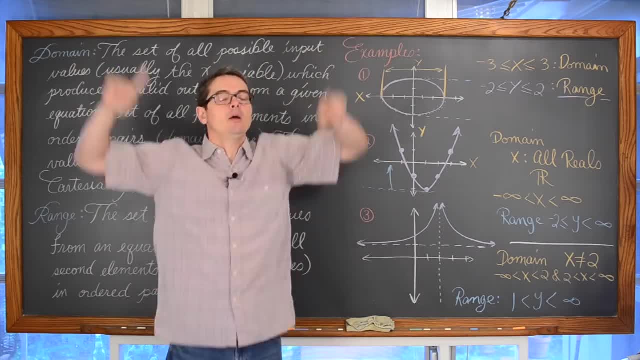 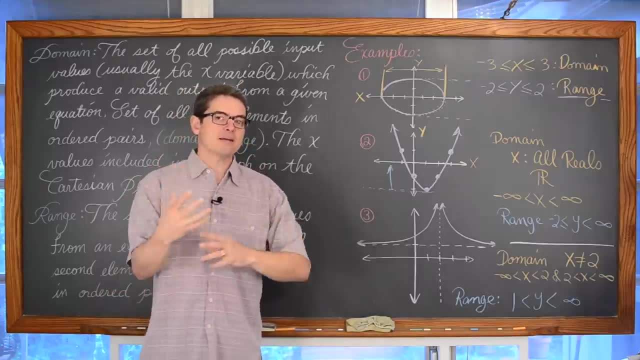 But because it goes up forever and never stops going up, we could not say that there's a maximum value unless you want to say the maximum value is infinity. But when we talk about identifying maxes and mins in a graph, we're looking for a concrete, like a real answer, if you will. 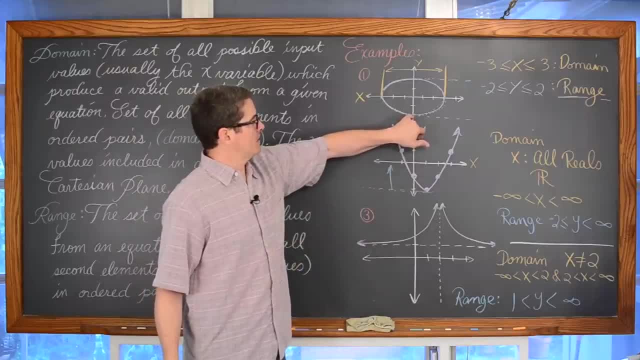 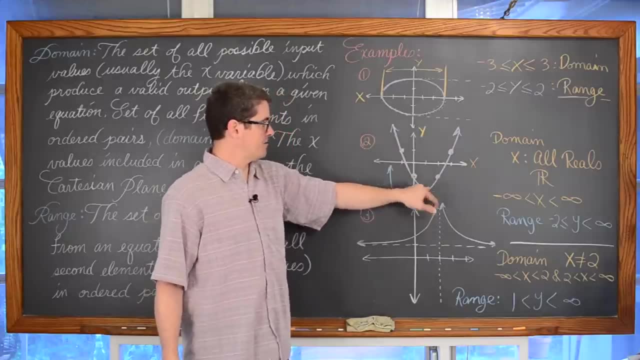 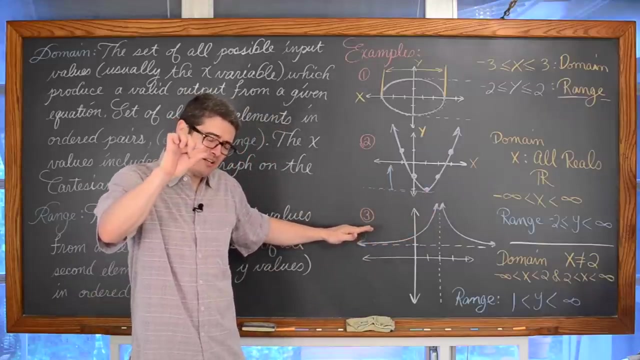 So this graph has a min of negative 2 and a max of positive 2.. This function, this parabola, has a min of negative 2 but has no maximum. And this graph is approaching 1, but it's becoming infinitely and infinitely and infinitely and infinitely closer to 1,.